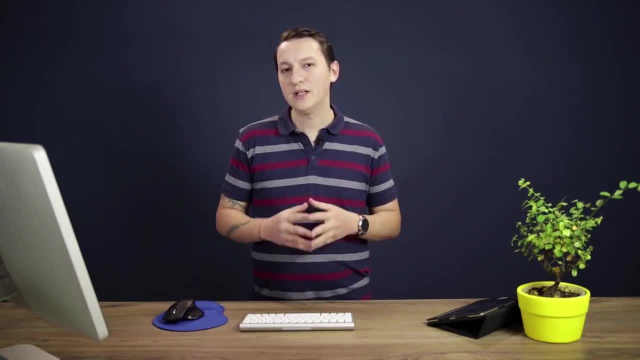 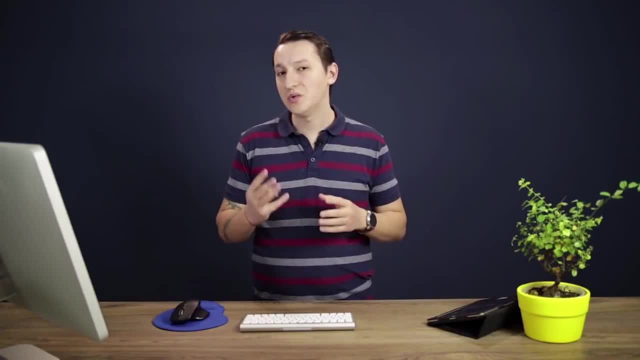 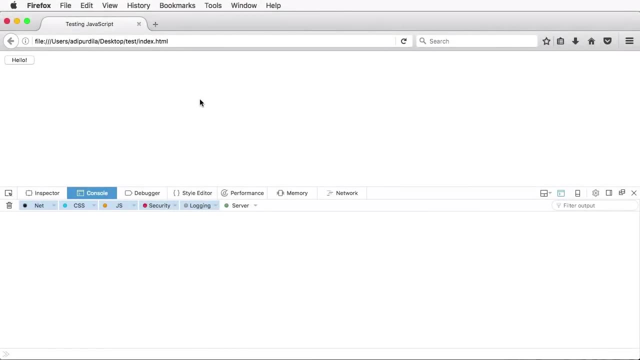 When it comes to writing and running JavaScript code, you can do it in three different ways. The first way is in the browser console, So I have Firefox here open And this right here is the console And, for example, I can type stuff like alert. 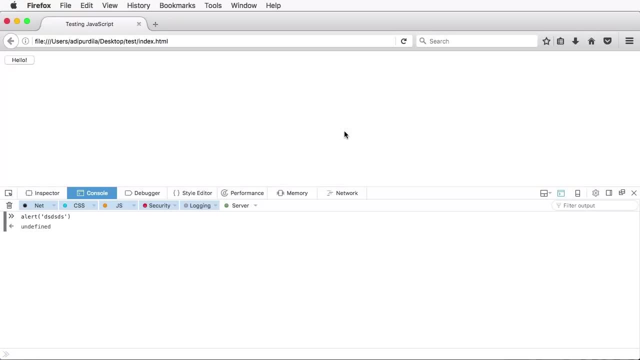 I can specify a message and hit that and I get an alert box. Or I can do a console log something else, a different message, and that will log to my console. So this is a very quick way to check things. For example, check a variable value, maybe debug your code or do very simple operations. 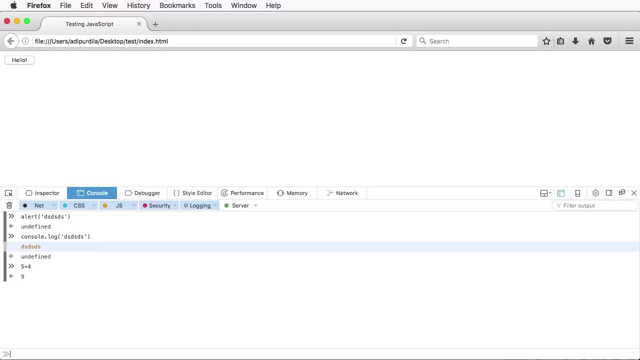 So, for example, I can do stuff like 5 plus 4 and it gives me 9.. I can do arithmetic operations, I can do Boolean operations. So if I say 1 is higher than 5, it gives me false all sorts of stuff. 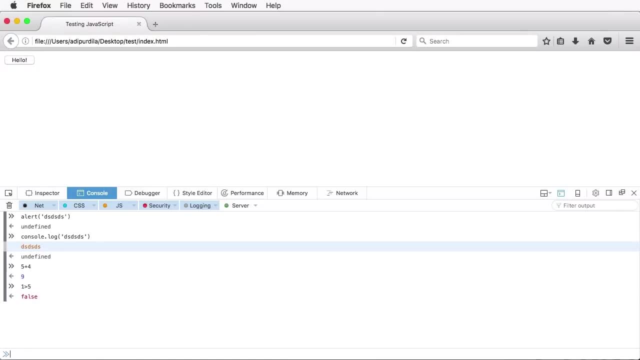 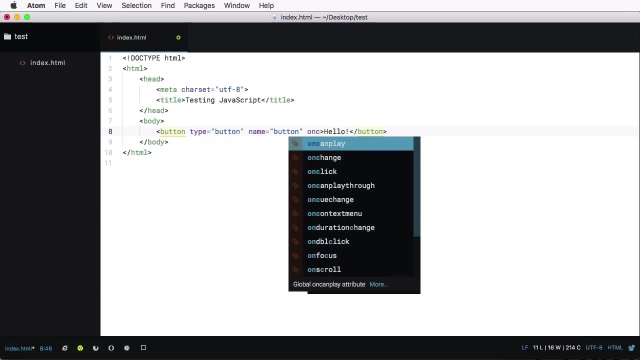 The second way is by writing it inline in your HTML document, And first you can for example go to an element and say stuff like onClick, for example, and type your JavaScript code. So let's do an alert here And say: click. 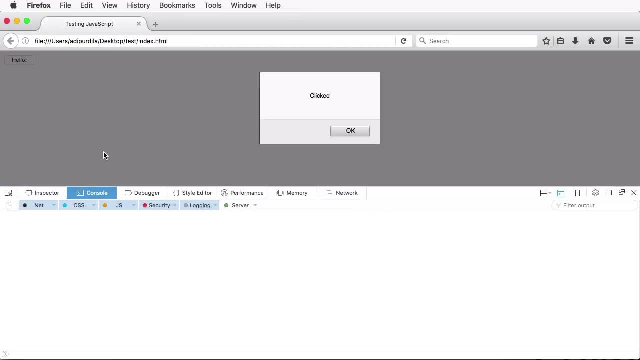 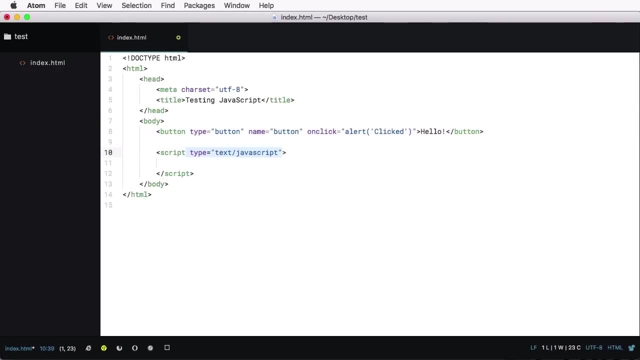 Then refresh, and when I hit this it gives me an alert. Or you can use script tags, So script also adds this type text JavaScript. You can leave it, but it's not necessary, So you can just do script script. 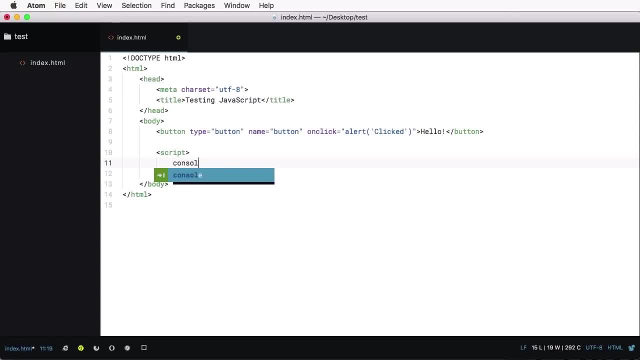 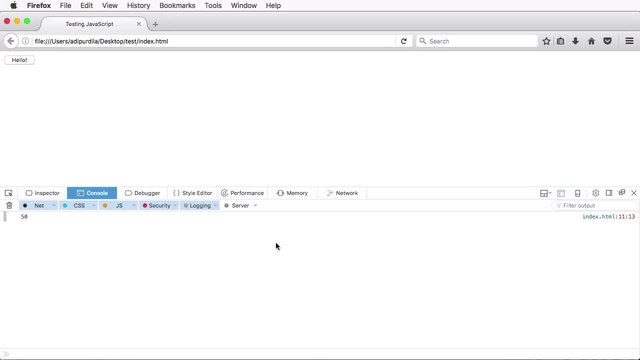 And then inside you can type your JavaScript code. So, for example, console log 10 times 5. And that's gonna give us 50 on the console. So finally, the third way of running and writing and running JavaScript is by using a dedicated JavaScript file. 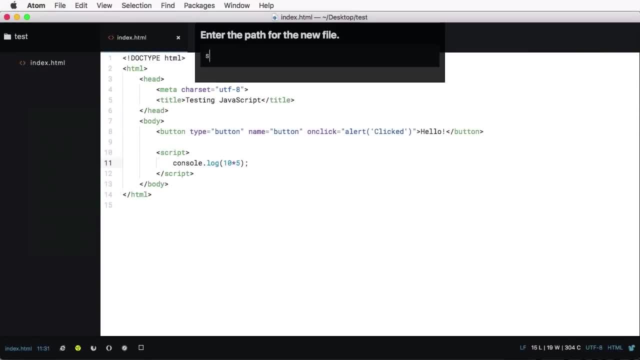 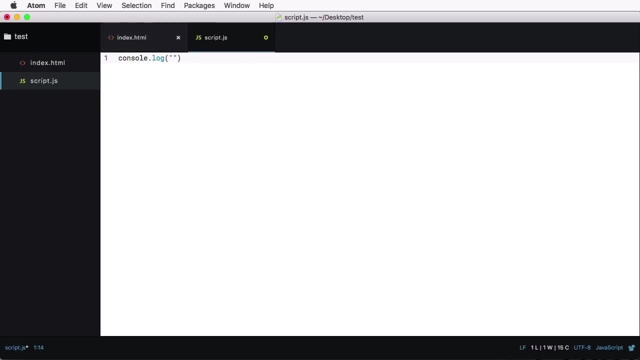 So, for example, I'm gonna create a new file here called scriptjs And I'm gonna do a console log from here. It says this is a log from a dedicated Js file, And then we actually have to load our Items file. 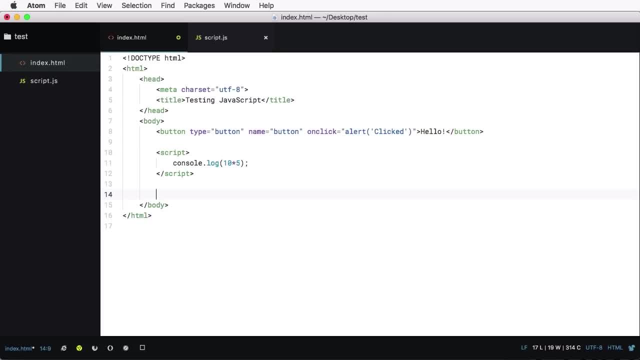 load that JavaScript file And we're gonna do it in the footer of our document. We're gonna say script, We're gonna delete this And we're gonna specify a source to scriptjs. We're not gonna type anything inside the script, only setting its SRC. 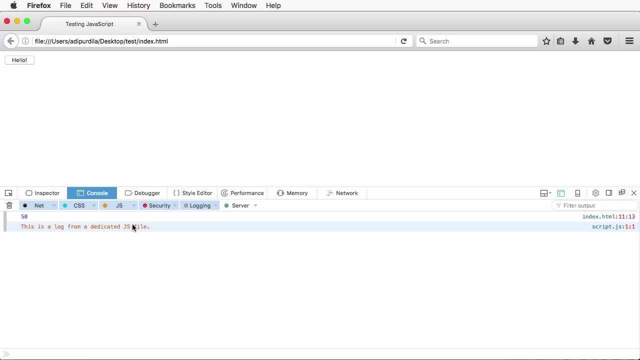 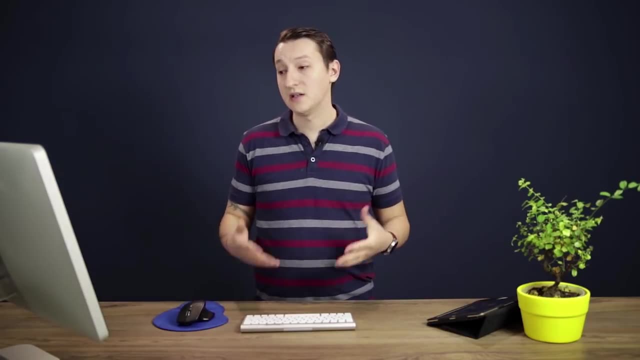 So now refresh, and we have that log entry. And these are the three methods you can use for writing JavaScript. Now for the upcoming lessons. go ahead and pick the one that you feel most comfortable with. Personally, I'm not a big fan of the first one, because, while it is good for, 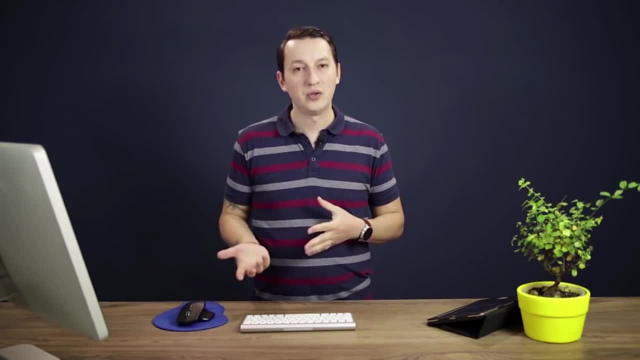 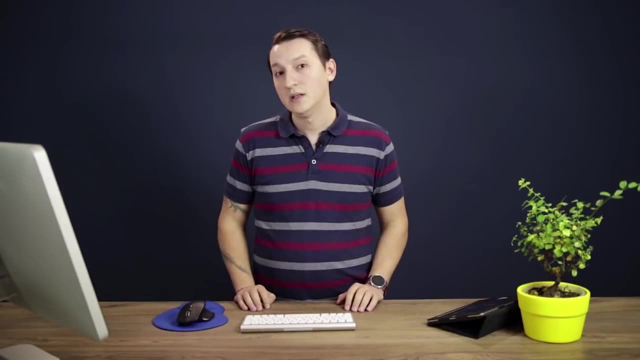 quick checks and very simple things. it's not very suitable for large blocks of code. Instead, I'll be using the second and the third, depending on the lesson. In the next lesson you'll learn everything there is to know about variables. 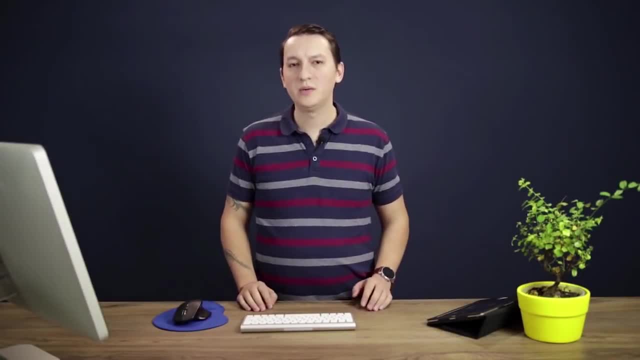 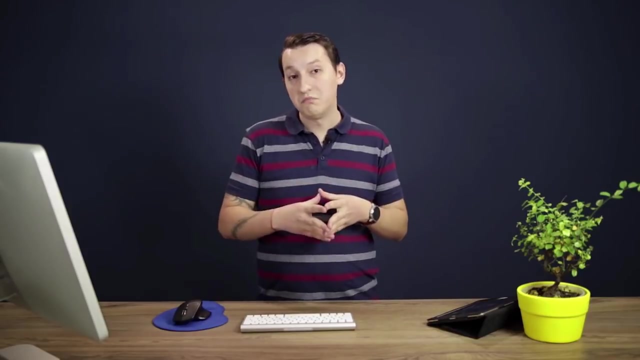 I'll see you then. Welcome to lesson number two, where you'll learn about variables. Now, if you've ever worked with a CSS preprocessor, like Less or Sass, then you're already familiar with variables. These store values of specific data types. 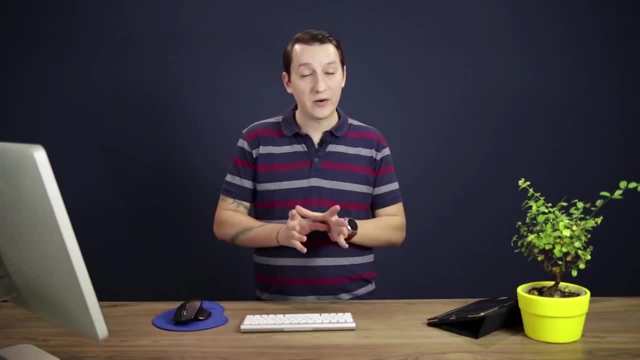 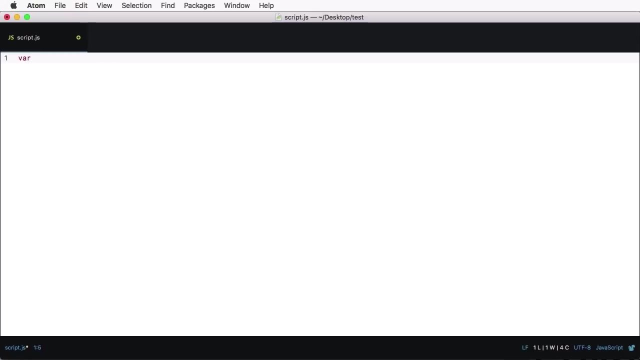 For example, you can store numbers, you can store strings of characters and so on. So in JavaScript, things are very similar. So in JavaScript, things are very similar. To declare a variable: that's where you start, right, You declare a variable and you do that with the keyword var. 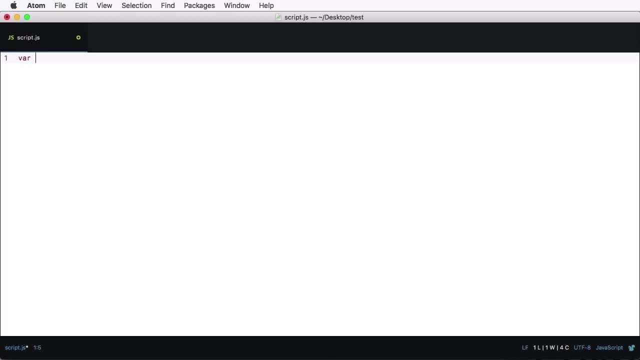 Now, following this keyword, var is the name of the variable or the identifier. Now you have to be careful when naming your variable, because identifiers have specific rules. They can contain letters, digits, underscores and dollar signs. They must begin with a letter. 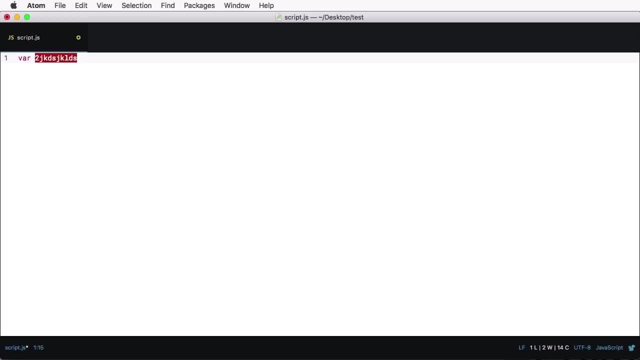 So, for example, if I do 3 or 2, followed by some letters, that's not valid. The names can also begin with a dollar sign and underscore, but we're not gonna use them in this tutorial And also names are case sensitive. 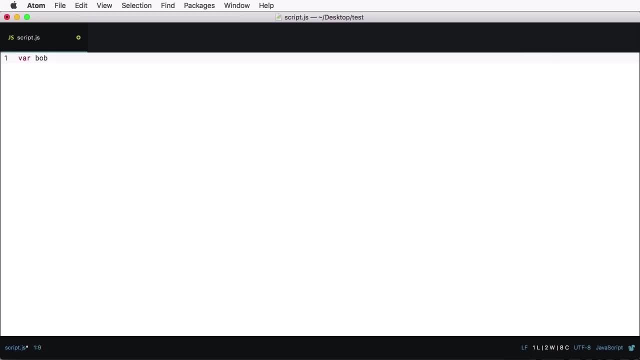 So Bob here is different than Bob with a capital B. These are two different variables. Also, remember that the reserved variable, the reserved keywords from JavaScript are also prohibited from being used as identifiers. So, for example, if I do var var, that's not correct. 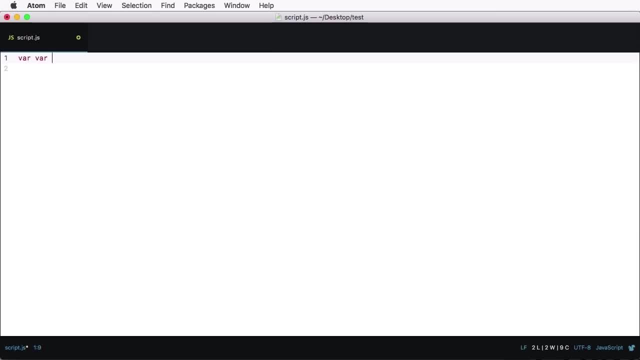 because var is a reserved keyword in JavaScript. So let's name a simple variable, let's say item, and then we're gonna end that line. If you want to define another variable, you can do again: var item2.. But you can also do it: var item colon, and then you can do var item2.. 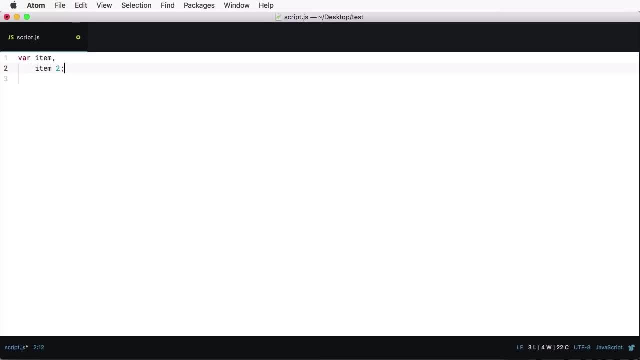 Now, this right here is not a valid identifier because it has a space. So either concatenate them like this or use an underscore. Now, how do you set a value in a variable? Well, after you've defined the variables, you can call them like this. 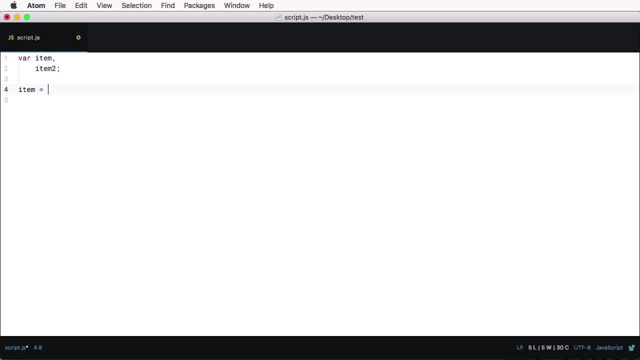 item equals and you can specify a value. I'm gonna say 5 here, and then item2 equals 5.. Okay, so I'm gonna put a string, I'm gonna say hello. So now the variable item holds the value of five and. 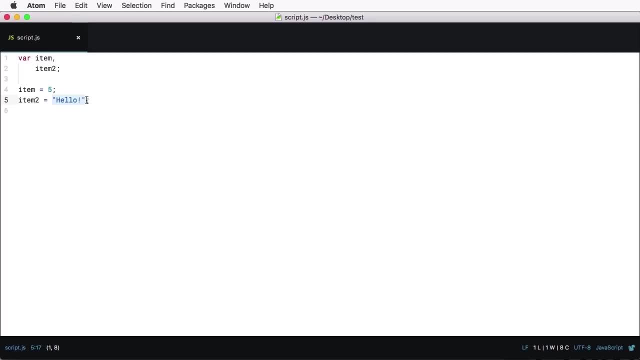 the variable item two holds the value of hello, and this is a string. So how do you call these variables? Well, very simply, by their name or by their identifier. So if I go back in our page here and I open up the console and 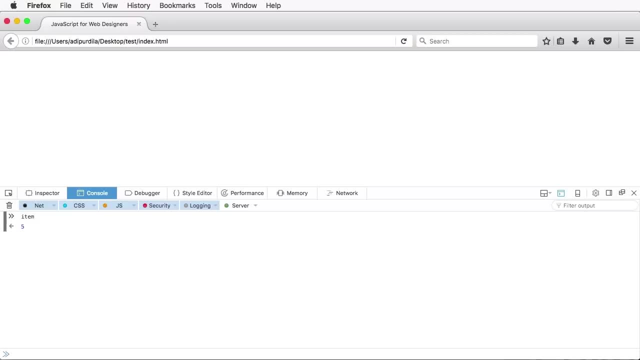 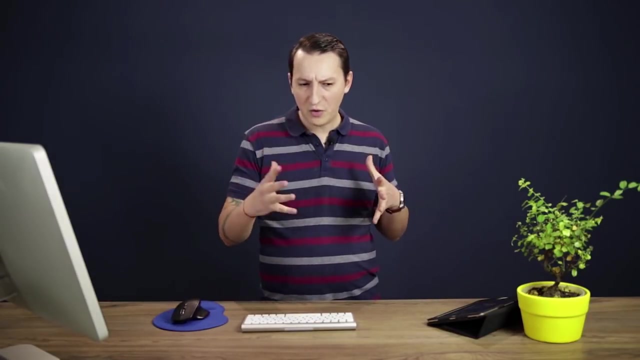 I say item, that's gonna print five. If I say item two, it's gonna print hello. If I say item space two, it's gonna give me a syntax error. So that's the easiest way to work with variables. Now, variables also have something that's called scope. 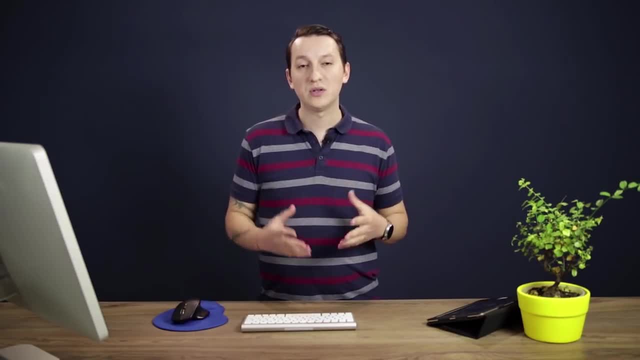 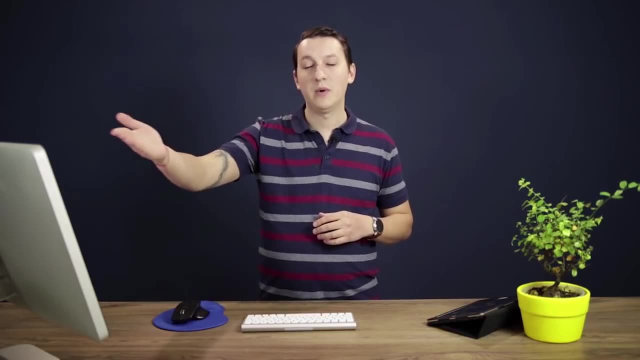 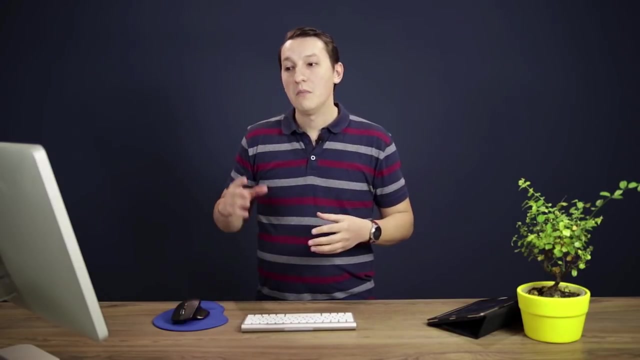 And scope refers to the context in which these variables are available. If you define a variable like this, the way I did it- item item two- they have a global scope, Which means they are available globally, But, as you'll find out in a later lesson, you can also create a local scope. 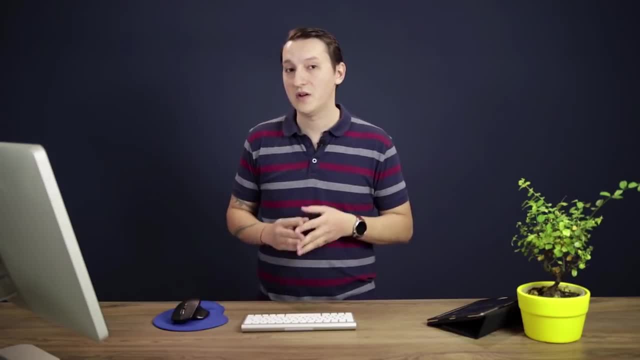 Inside, for example, a function or a specific block of code. In that case that variable, which has a local scope, is only available within that function or that block of code. But I'm just mentioning this right now. We'll go into in more detail. 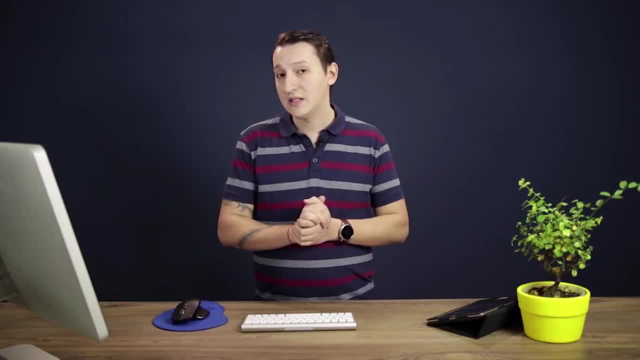 further down the line. But that's about it for variables. just a quick lesson Now. as I was saying in the beginning, variables can hold multiple data types And we'll be learning about that in the next lesson. See you there. 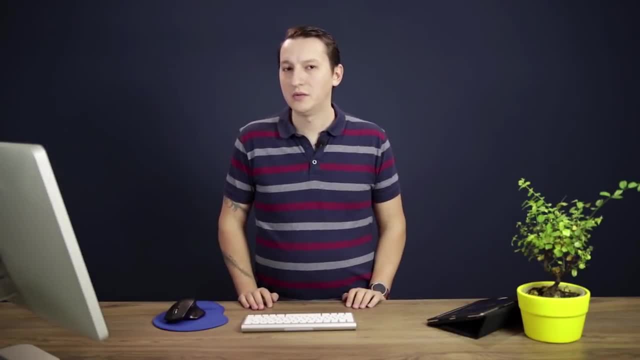 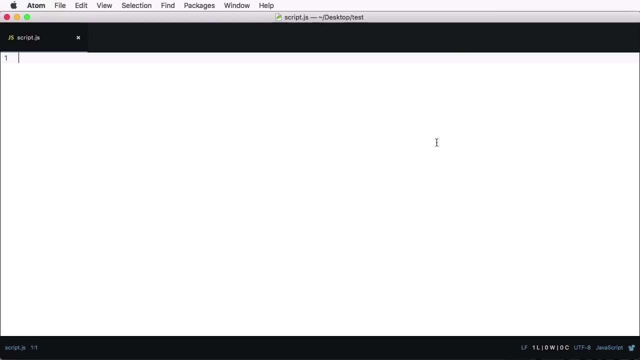 Hello and welcome to lesson number three of this course, where you'll learn about the data types in Java's root, And there are seven data types in total. Five of them are primary, two are composite. Let's go ahead and start with the primary ones. 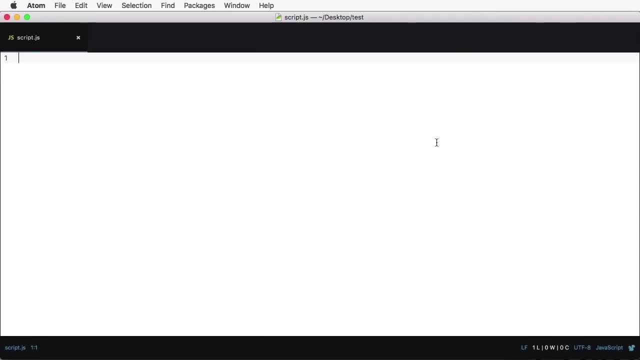 These are string, number, Boolean, null and undefined. The string is basically a group of characters, So you would say, for example, var name equals John. That's a string And you can use double quotes and you can also use single quotes. 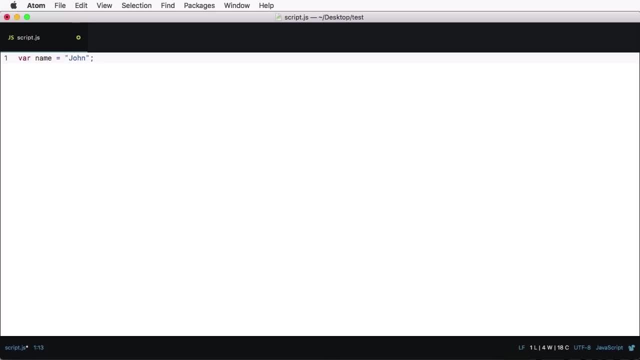 But it's usually preferred to use double quotes. The number data type would be something like this: age 32.. This is written without any kind of quotes. If you would put 32 inside quotes, it would then be treated as a string instead of a number. 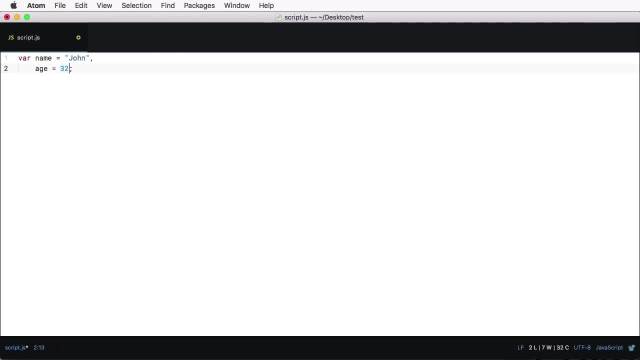 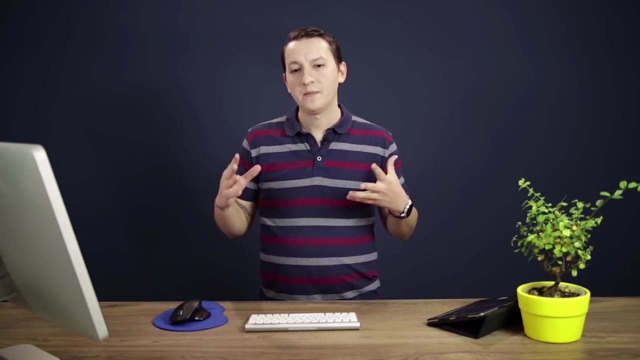 Now, numbers can be either integers, like this, or floating points, like this: 32.12, that's a valid number. The next type is Boolean. Now, Boolean is a special type because it can only hold two values Very different from the other two types. 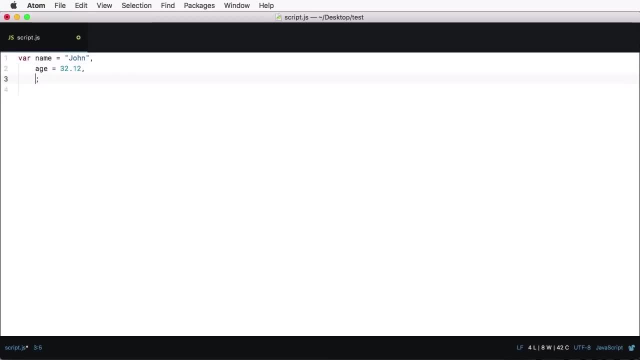 It can be true or false, So I can say something like married equals true or equals false. The fourth primary data type is null. Now, the null data type has a single value, a single value in JavaScript, and that is null, And it's usually used to erase the contents of a variable without deleting. 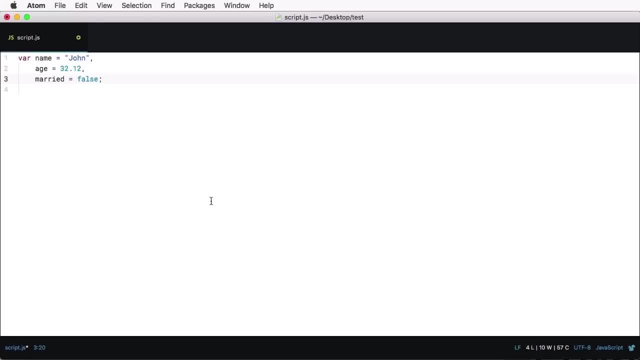 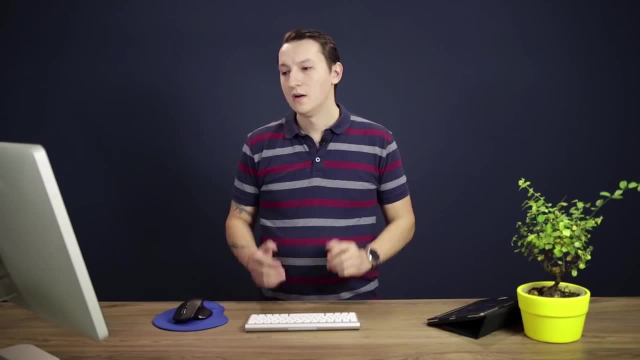 the variable itself. All you have to do, for example, is set age to null, And age will have no value whatsoever. Finally, the undefined data type usually happens when you're trying to access an object properly that doesn't exist, or you're trying to access 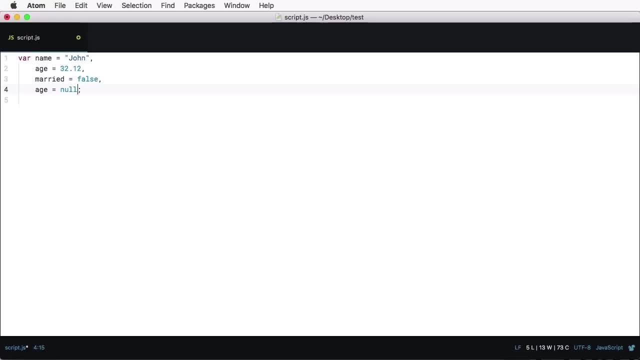 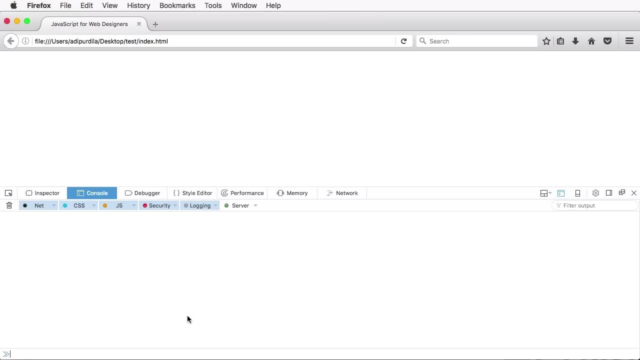 a variable that has not been given a value. So, for example, if I set a variable here called carModel, for example, And I go back here and I say carModel, it's gonna return undefined, While if I say age, it's gonna give him back null. 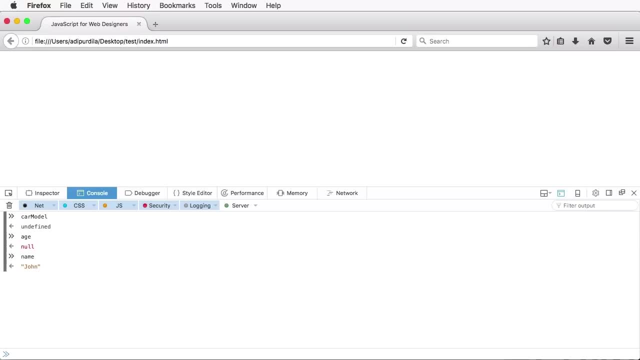 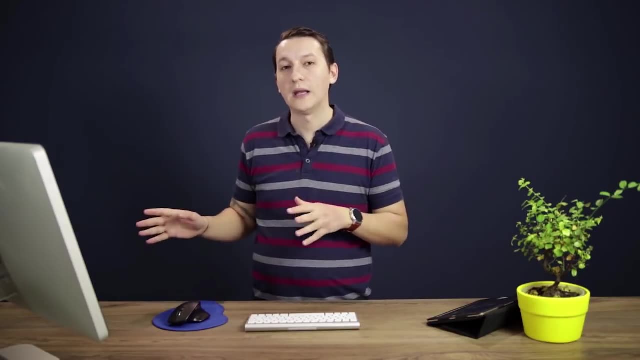 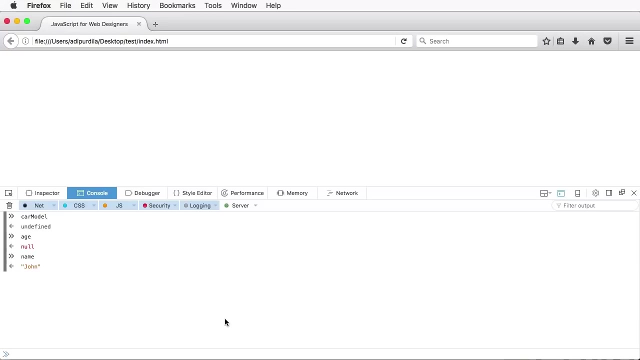 So you see the difference between the two. But if I say name, it's gonna return John. So those are the five primary data types. Now, before we move on, I just wanna quickly show you something called typeof. Now, typeof is an operator. 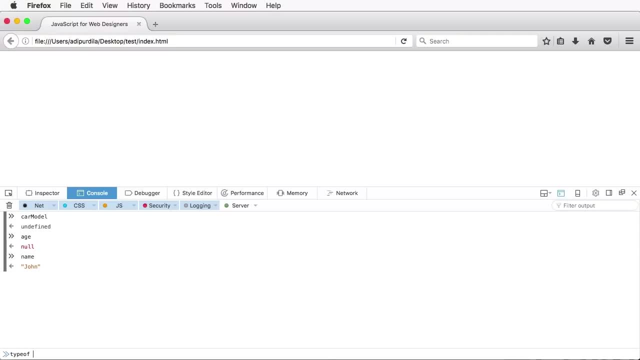 And you do something like this: typeof, and it's followed by an operand. So watch what happens. if I say typeof age, Typeof age gives me an object, But if I say typeof name, it's gonna give me a string. Let's try typeof. 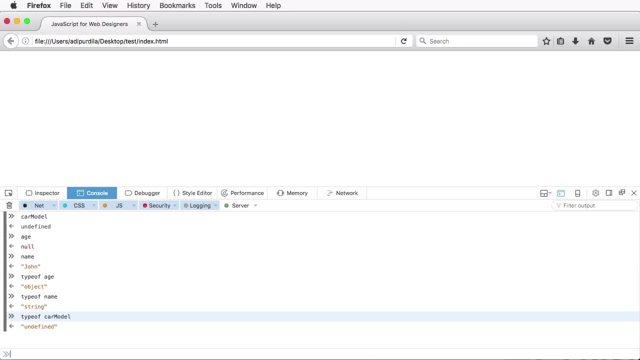 CarModel gives me undefined. So what happens is when you're using the typeof operator, it's gonna return the type or the data type of the operand. So, for example, if I say typeof false, it gives me boolean. If I say typeof false in double quotes, it's gonna give me a string. 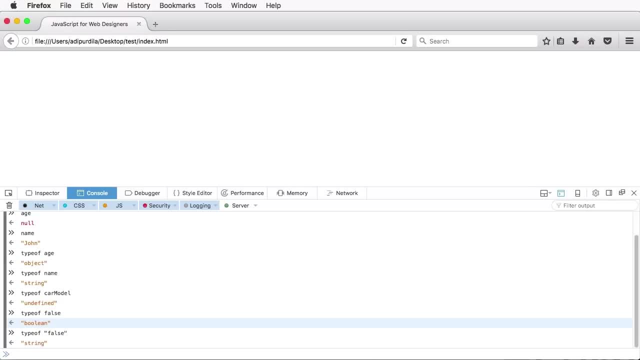 So it's a very nice way of checking the type of a variable, And this can be used in lots of different ways, For example, when you're doing some operations between two variables And first you wanna make sure that they have the same type to prevent errors. 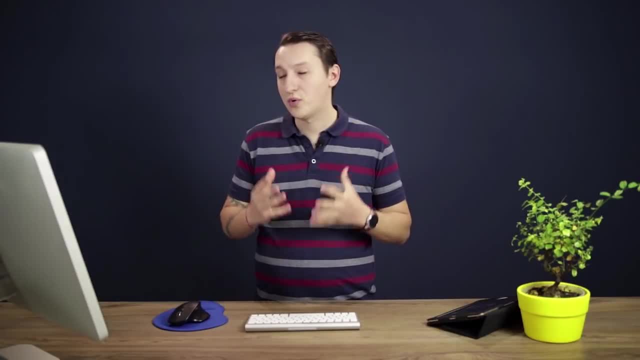 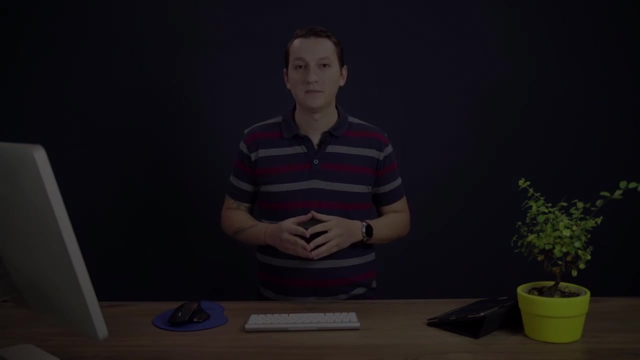 Now, that's pretty much it for the primary data types. The composite data types I mentioned earlier are arrays and objects. There are two of them And we'll be learning about those In the next lesson. Hello and welcome to lesson number four. 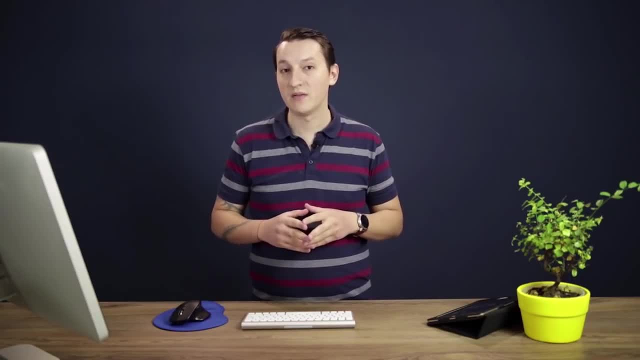 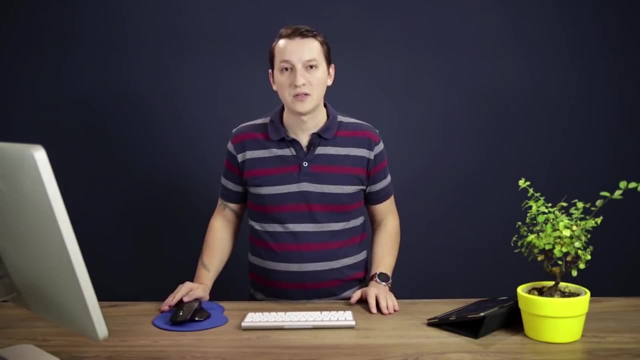 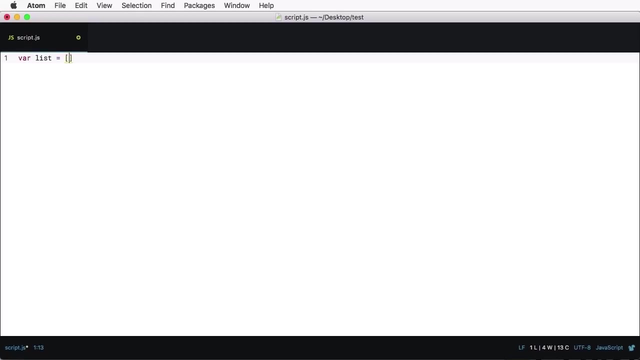 where you'll learn about the first composite data type in JavaScript, which is arrays. Now, an array is basically a list of values, And the way you can clear one is simply var. Let's call it list equals and we'll use square brackets. 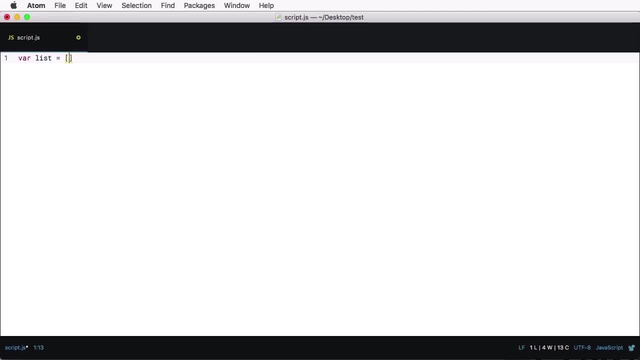 And we can put in the list of values. For example, I can say John Marie, and we separate these by commas, And Sander- I can think of a better name there. So this is an array which has three string items. 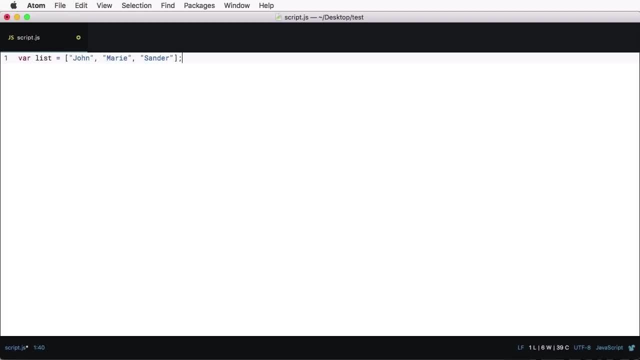 But you're not limited to string items. You can have an array of booleans or an array of numbers, Or you can mix and match. So, for example, I can add another one here that says 32.. Or, for example, I can add another one here that says 32.. 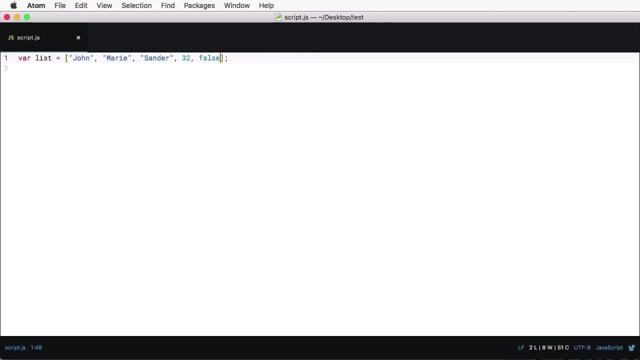 Or, for example, I can add another one here that says 32.. Or I can put another one here that says false. right, So this is a valid array. Now, this is the first method of declaring an array. You can also declare an array like this: 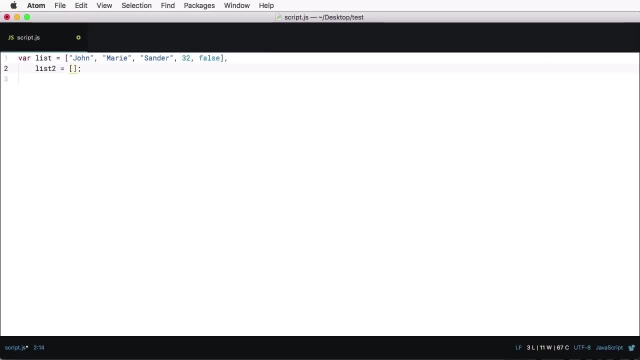 For example, list2 equals this. This is an empty array, but it's an array nonetheless. Or let's call this: list3 equals new array, And here you can also specify its contents, For example 12 and false. This is a valid syntax. 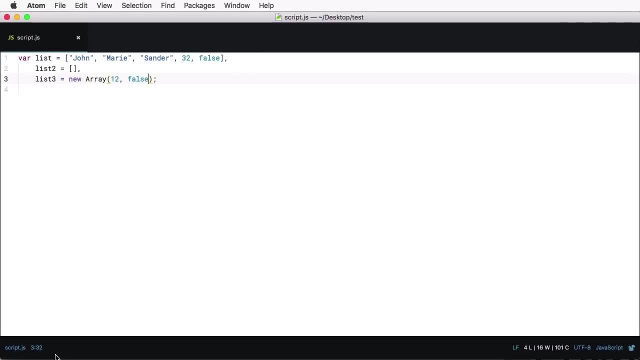 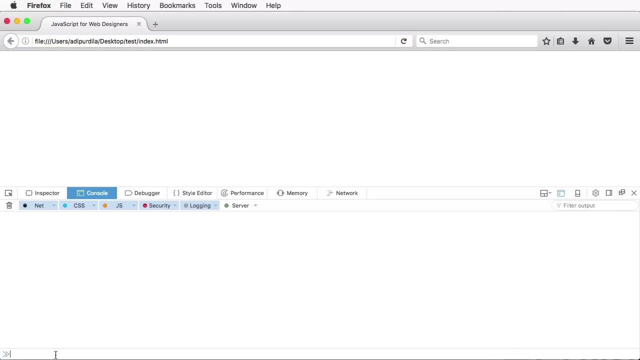 Now, this is how you declare an array, But how do you access it? Well, just like you would access any normal variable. So if I go back in here and I say, for example, list, it's gonna give me my array John Marie Sander, 32 and false. 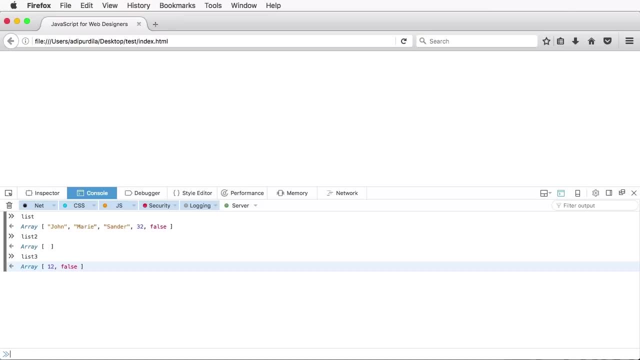 Or list2, it's gonna give me an empty array. Or list3, it's gonna give me the third array that we've just created. Now, this will give you the entire array, But what if you want to access a specific element from that array? 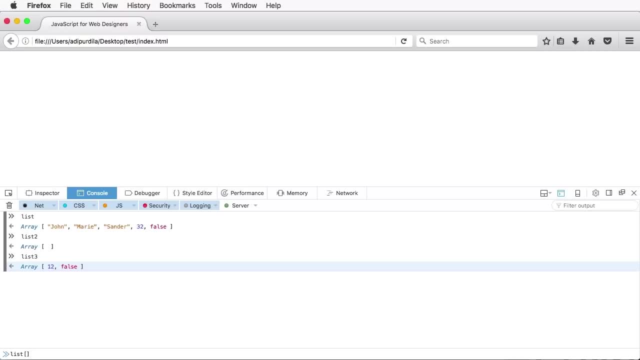 Well, to do that, you would say list, You open up square brackets and you specify a number from 0 to whatever you want. basically, Arrays are zero-based index, which means the first item sits on position 0.. The second item sits on position 1, and so on. 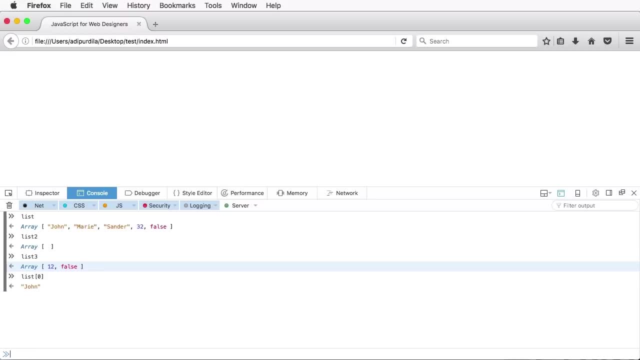 So if I say list0, it's gonna give me John. If I say list2, it's gonna give me the third item, which is Sander. If I say list5, it's gonna give me undefined. Now, why is it giving me undefined? 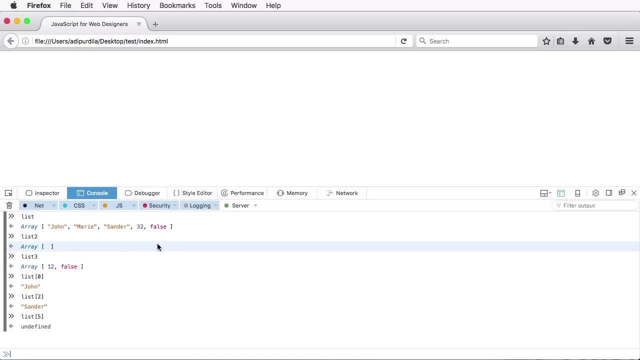 Well, because our array has five elements, So its element count only goes up to four: 0,, 1,, 2,, 3, and 4, five items. So if I specify an index, this is: this is what it's called. 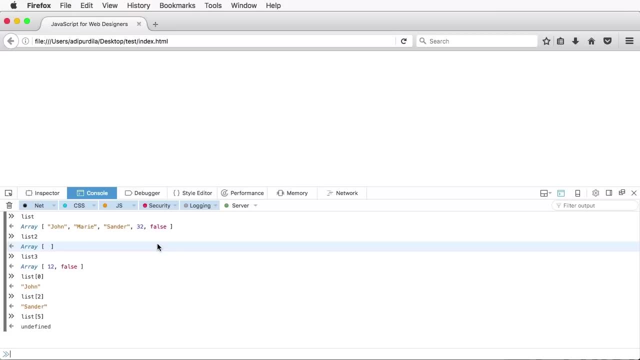 If I specify an index that's larger than the length of the array, it's gonna give me undefined. But if I say list4, it's gonna give me the item on the fifth position. Now, the way to access these arrays is the same. 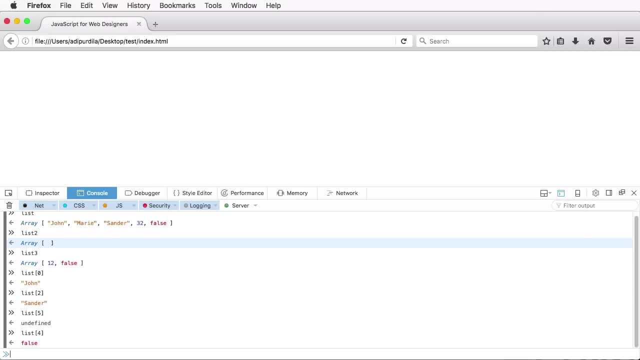 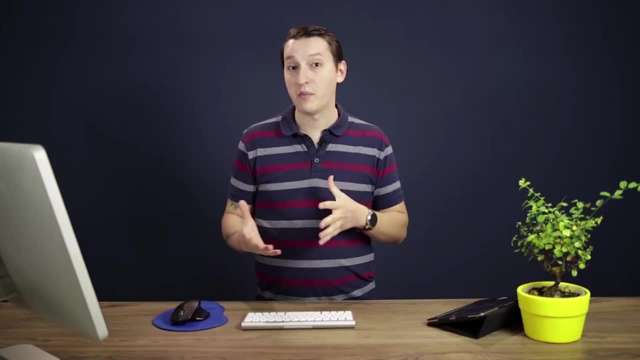 regardless of how you define them in the first place, Either using this syntax or using the new array syntax. Now, arrays have properties and they have methods Properties we're only gonna talk about one, and that is length, And the length property gives you the number of items from that array. 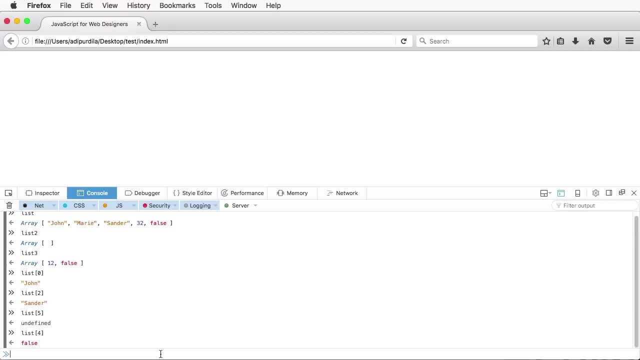 The way to access that property is with the array name. In our case, let's do listlength, And listlength is gonna give me five because I have five items. List2.length is gonna give me five items. List2.length is gonna give me five items. 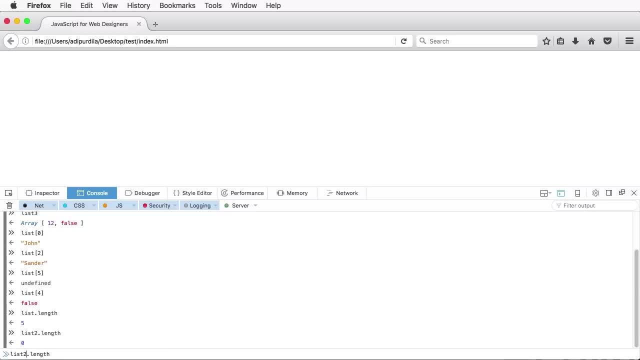 List2.length is gonna give me five items And list2.length is gonna give me 0, because it's an empty array, And list3.length is gonna give me two because we have two items in that array. A very simple property you can use to find the number of items in an array. 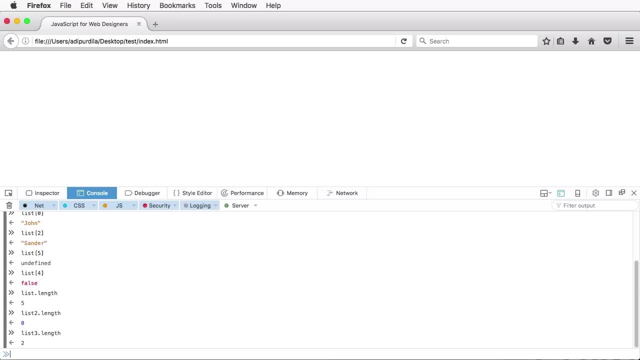 Now let's move on to the methods, because these are a bit more interesting. The methods we're gonna be talking are push-pop-shift-un-shift and indexOf an item to the end of an array. So I have my list array here and if I want to add another item, 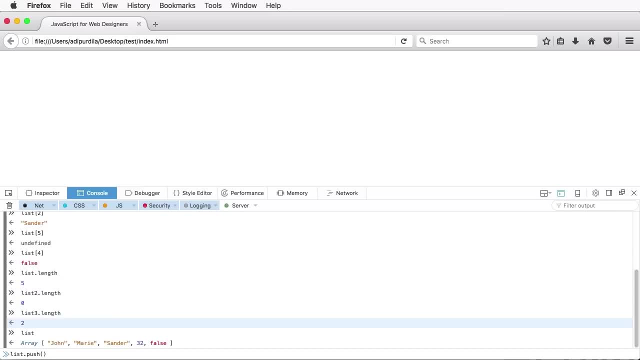 I can just say listpush and then in parentheses I'm going to put my item and that can be anything: boolean, number, null string, whatever. So I'm just going to put a string and I'm going to say hi. So now it gives me the new length of my array and if I do list again, I get the updated array. 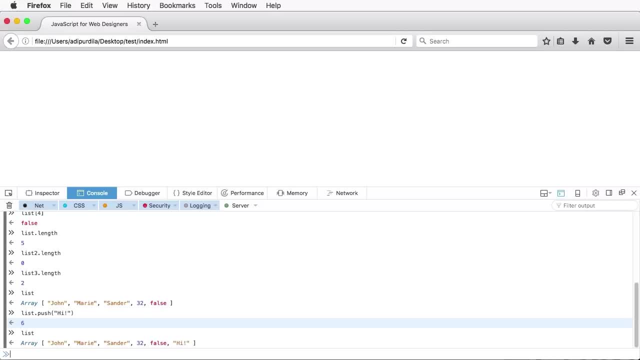 So that's push Pop will actually remove an item from the end of the array, So I can say listpop. make sure you use parentheses because this is a method and that gave me the item that was removed from my list. So if I redo you'll find that with the list. 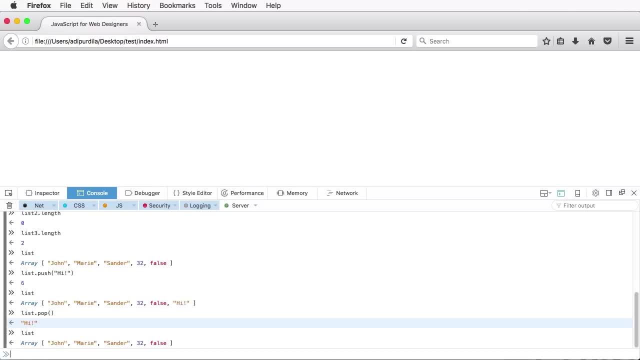 We now have an array with just five items. The third method is called shift and it's used to remove an item from the front or the start of an array. So if we do listshift, it removed john. As you can see, john is now gone. Now to add to the front of an array, you would use unshift. 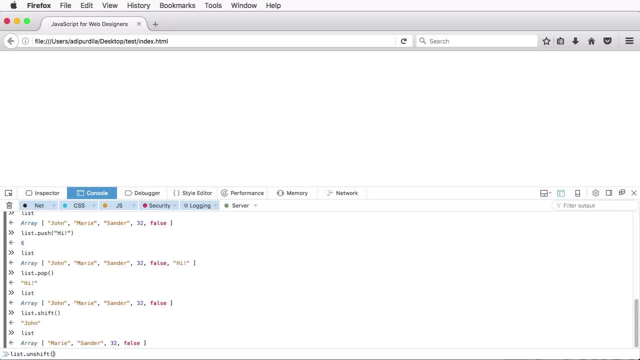 So listunshift, I'm going to add 10 here. So now list is this bit. Finally, index of is used to find the index of a specific item in an array. So let's say, for example, that I want to find a position of the number 32 in my. 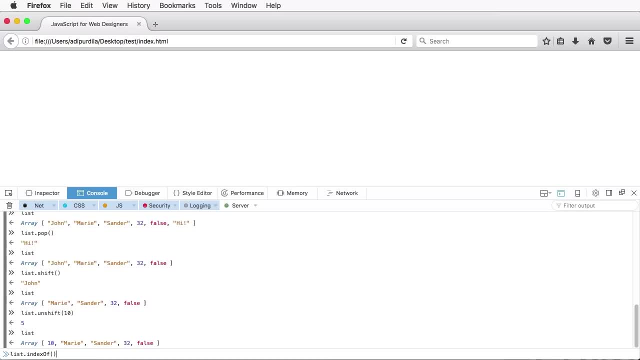 array So I can do list index of 32 and that gives me 3.. So we have 0,, 1,, 2, and 3.. But if I do index this bit, it actually tells me that it's not defined. But if I do index of 32,, 32,. 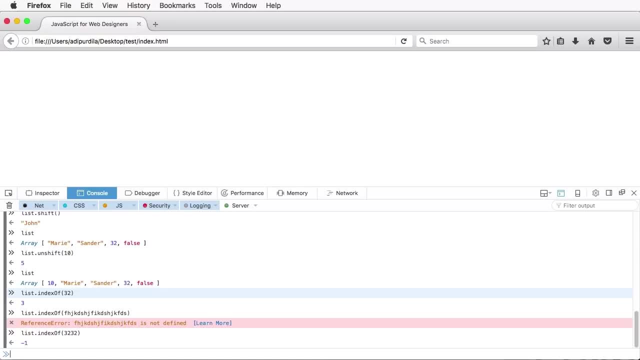 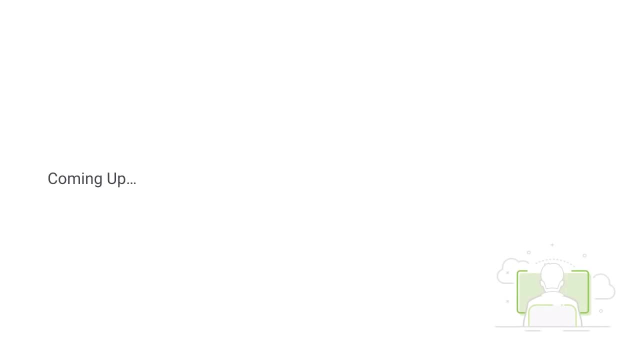 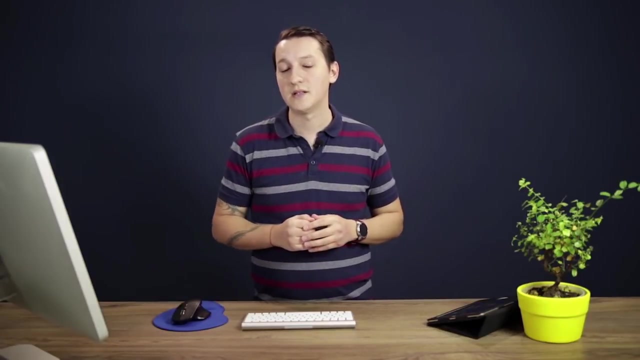 it gives me minus 1.. And this is the value that's returned in case that item is not found in the array. And that's pretty much it for arrays. Now coming up, we'll talk about the second composite data type, which is objects. See you there. Hello, and welcome to lesson number 5, where 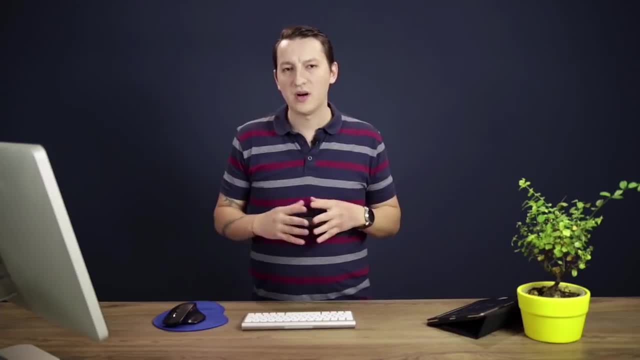 we learn about objects Now. objects in JavaScript are, I think, pretty easy to understand, And it all starts from properties. A property is an association between a name and a value. For example, color equals red. That's a property. Properties can also have functions as values, In which case those properties are called methods. 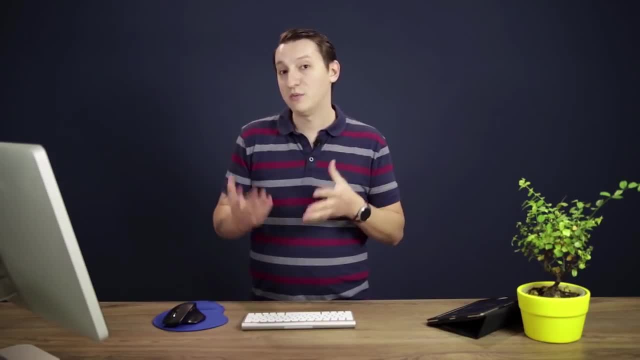 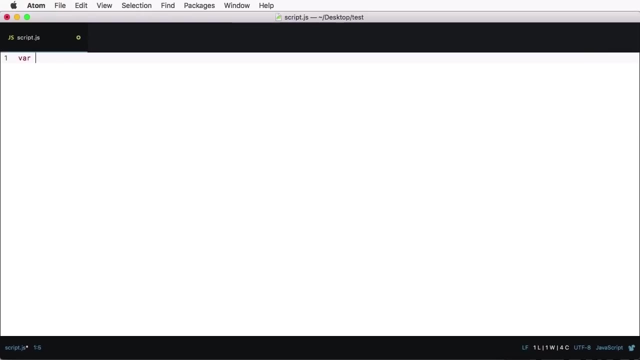 But we'll come back to that Now. objects are collections of properties, plain and simple. So let's have a look at how you can create an object, how you can access it and all that good stuff. To create an object, you start, of course, with a variable, And let's call: 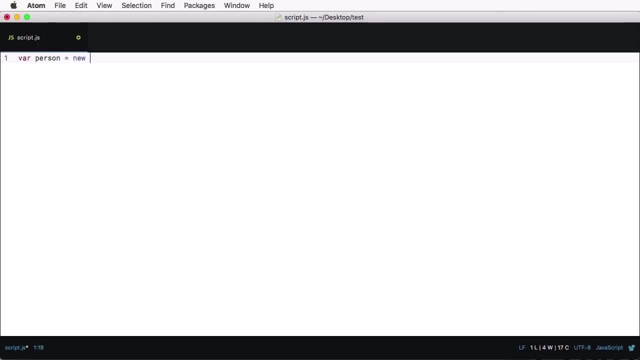 this variable person And we're going to say new object. That's one way to create it. Another way is to create, let's say, car equals curly brackets. So just like arrays, where we used square brackets to create them, or the syntax new array objects, we use new object. 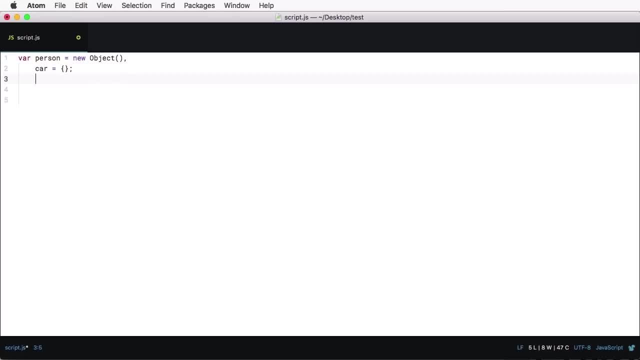 and curly brackets instead of square brackets, And what you can do now is start adding properties to these objects. So, for example, person, What could we want to know about that person? We want to know its name, its age, maybe its height, right, So you can say: person, dot name. 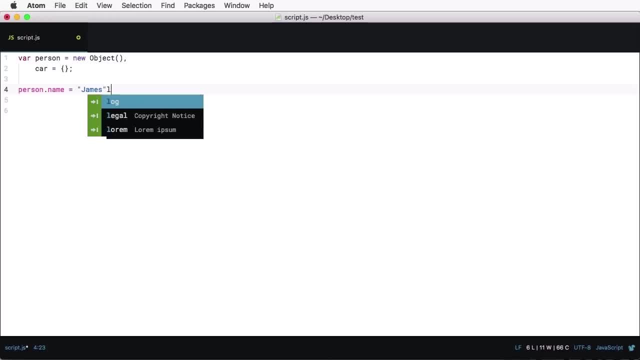 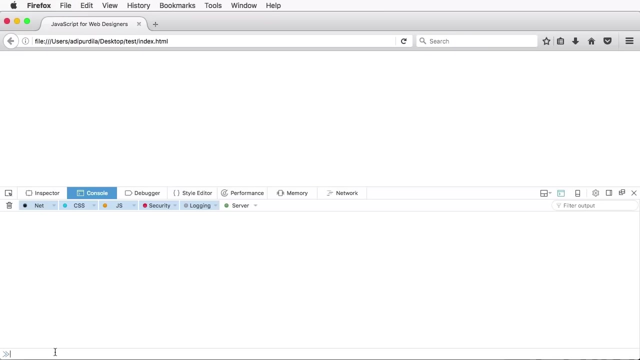 equals. let's say, James. Person dot age equals- I don't know- 43.. Person dot height equals 1.76.. And actually this should be a number instead of a string. And we can also say: person dot married equals true. So now if we type person, 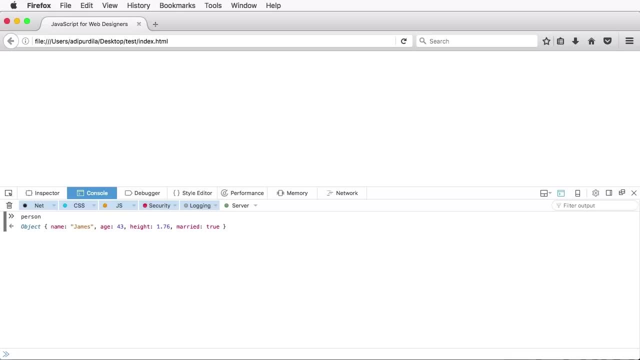 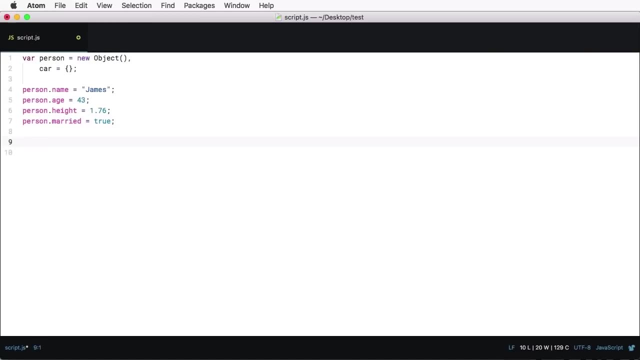 in our terminal. here we get an object with name: age, height, married, set to the values you just saw. You can also access these properties in the following way: Person, square brackets and then, inside double quotes, the name of the property. Person name equals. 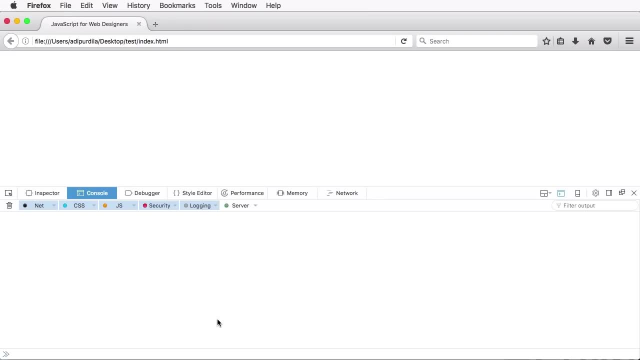 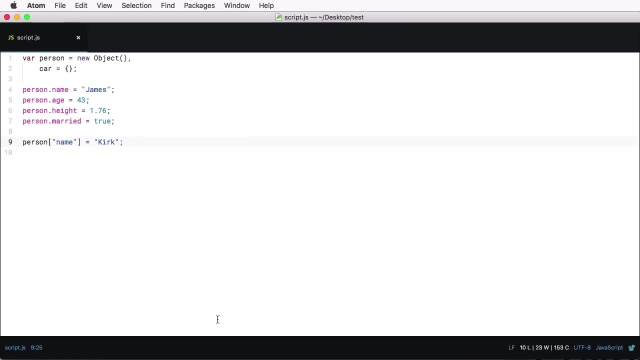 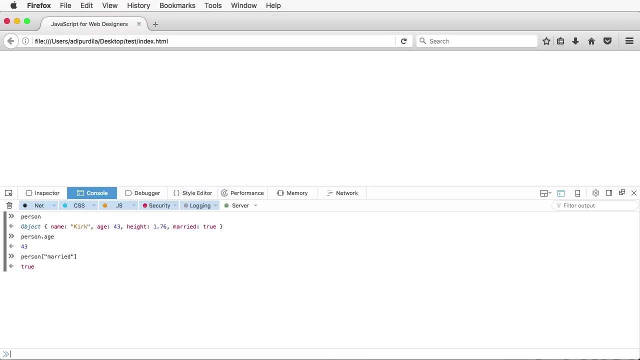 let's change this to Kirk Refresh. And now, if we bring up person, it's going to give me Kirk For its name And that's how you can access these properties and also how to change these properties. Both syntaxes are valid, but probably the dot followed by the name of the. 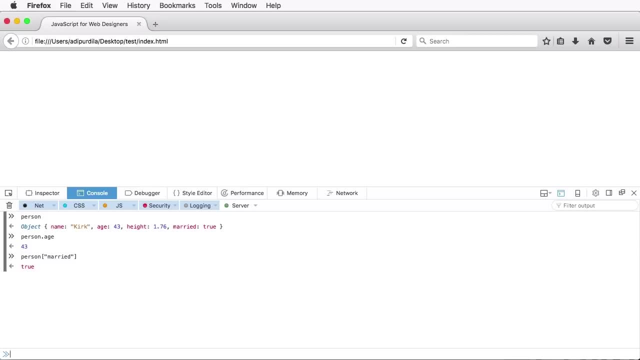 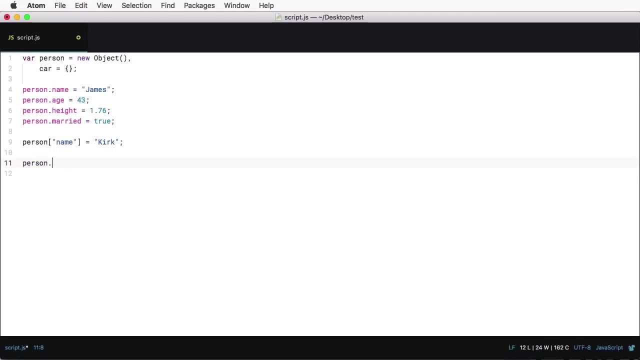 property is the easiest one to use. Now you can use objects inside objects, in the way that an object is the value for a property. So, for example, if I add another property here called car- or let's not confuse it with this one here, Let's just delete this, Yeah. So I'm going to say 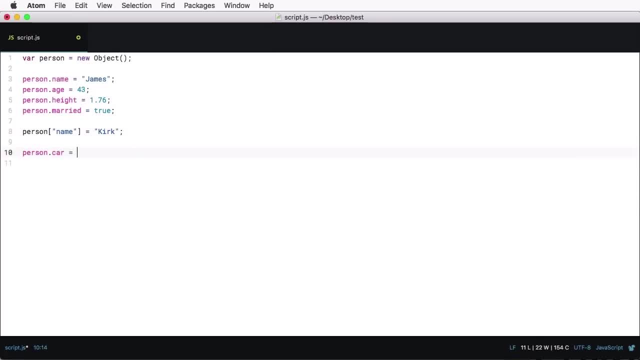 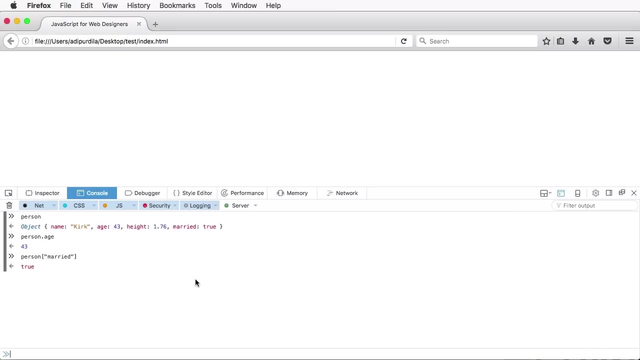 person dot car equals a new object. And then I can go and say: person dot car, dot make equals Honda, for example. Right So now, if I recall person, it gives me this object. And if I do person dot car, it gives me another object. And if I do person car make, 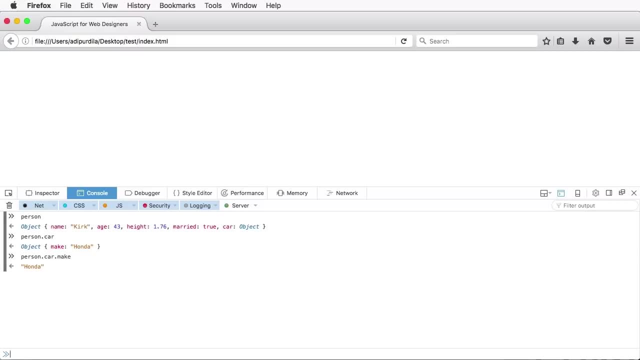 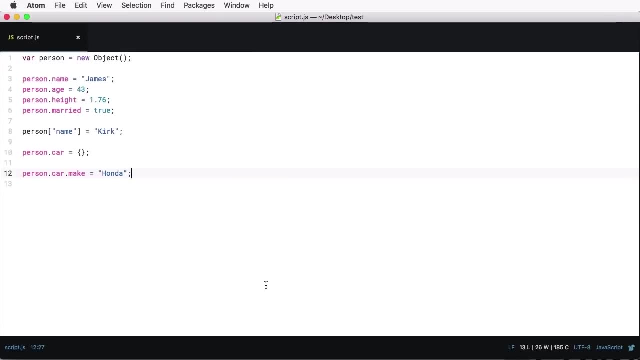 it gives me Honda. So this is how you can access these object properties, even if they're embedded in one another. Now you can also define these properties when you first initialize an object. So, for example, let's delete this and I can say: var person equals. 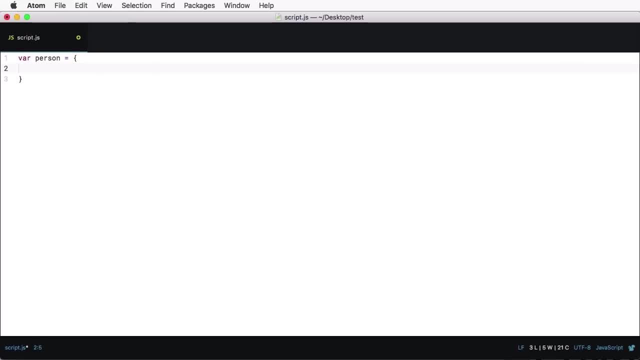 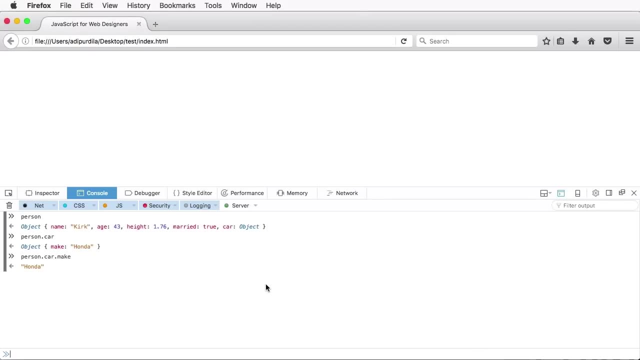 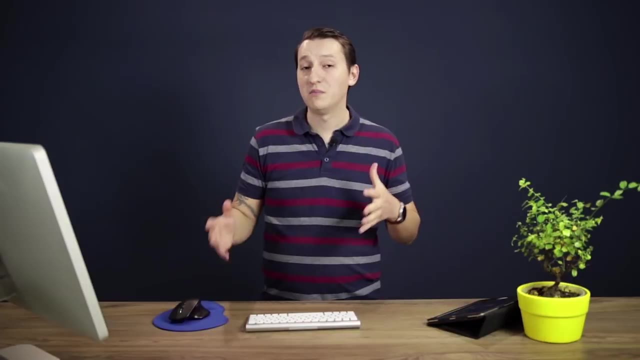 and I can specify it like this name: Adi, age 30.. Notice, the syntax here is a little bit different. So now, when I access person, I get this object. As I was saying in the beginning, objects can also have methods, And a method is simply a property that has a function as its. 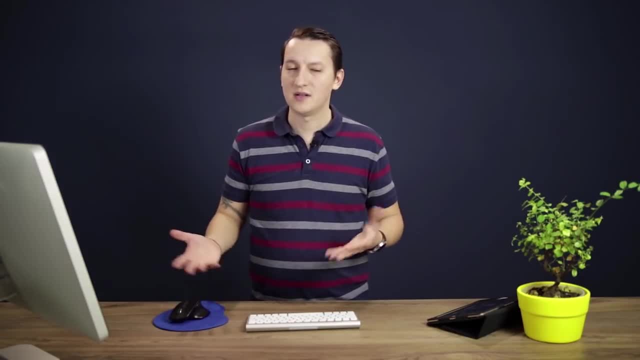 value. But we didn't learn about functions just yet, So there's no point in me talking about object methods right now. What I gave you right here are the basics of objects: How you can create them, how you can use them, how you can access. 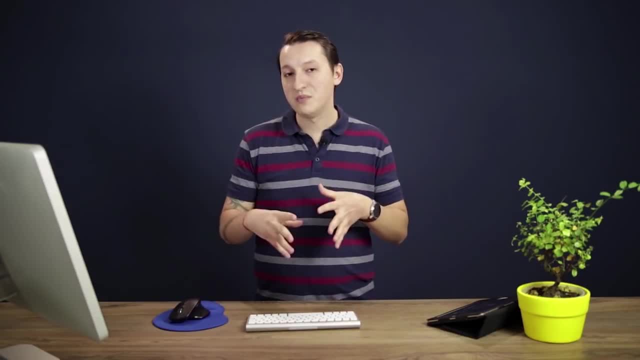 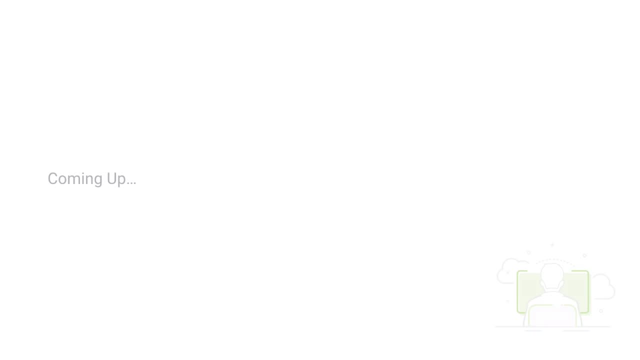 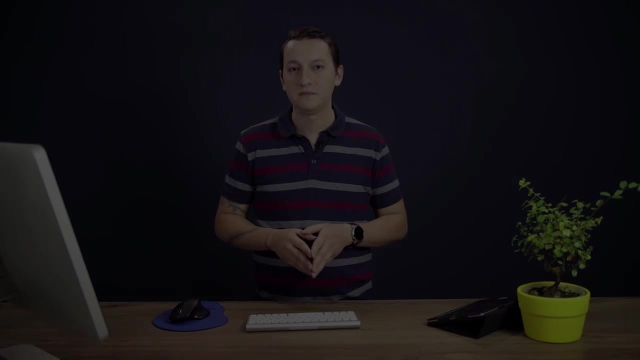 their various properties And with objects. we've actually completed all seven data types in JavaScript Now coming up. in the next lesson we'll learn about the available operators in JavaScript. See you there, Hi. Welcome to lesson number six, where we're going to learn about the available cell function stones. 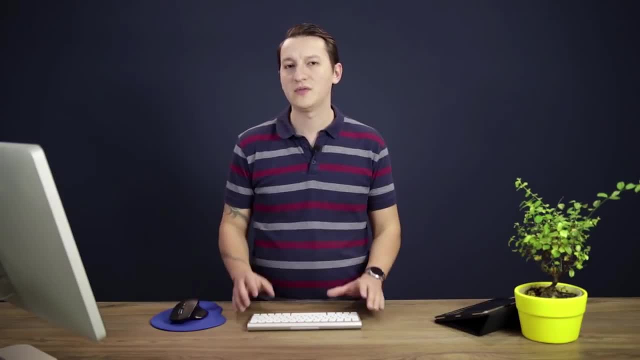 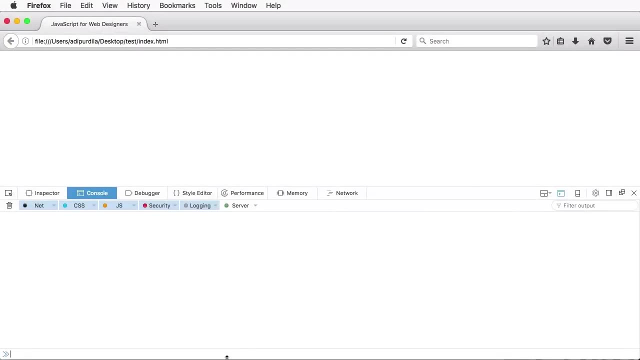 where you'll learn about operators, and there are a few different types. Let's begin with the assignment operator, since this is the most basic Now. the assignment operator will basically assign a value to its left operand based on the value of its right operand. 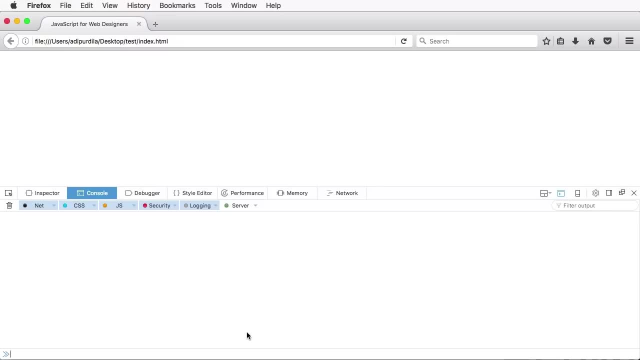 And the simplest one is the equal operator. So let's say, for example, that I have a variable: x equals 1.. We assign the value of 1, the right operand, to x, the left operand. So now if I type x, that's gonna be equal to 1.. 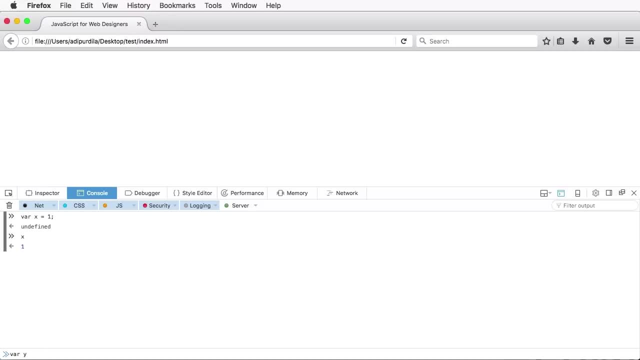 I can also have a variable. for example, y equals 3.. And then what I can do is say x equals y, and now x will have the value of 3.. So that's the best way to do it. So that's the basic form. 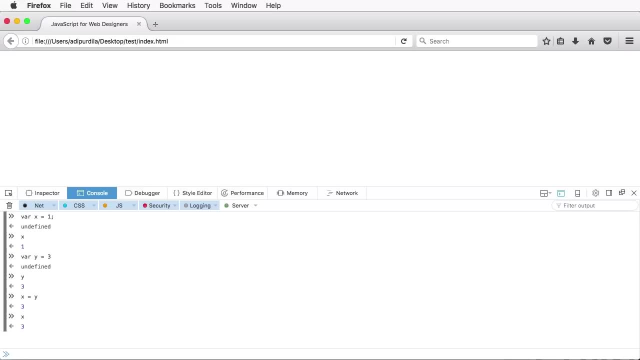 Now there are also compound assignment operators, For example the addition assignment. That looks something like this: x equals x plus y, And that gives us 6, but I can also say x plus equal y. X plus equal y is the same thing as x equals x plus y. 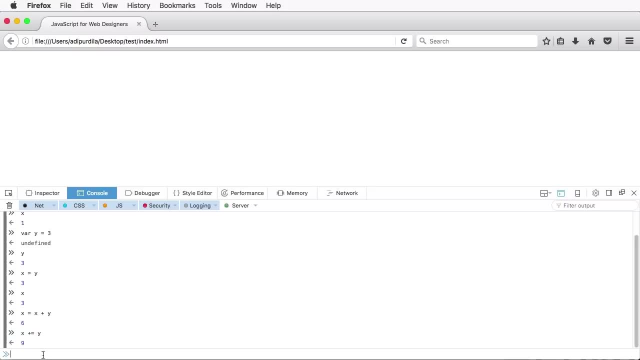 Similar to these are subtraction, multiplication and addition And then division and a bunch of others. But I'm just gonna show you a few examples here. So the subtraction will be x minus equal y. The multiplication's gonna be x multiply equal y. 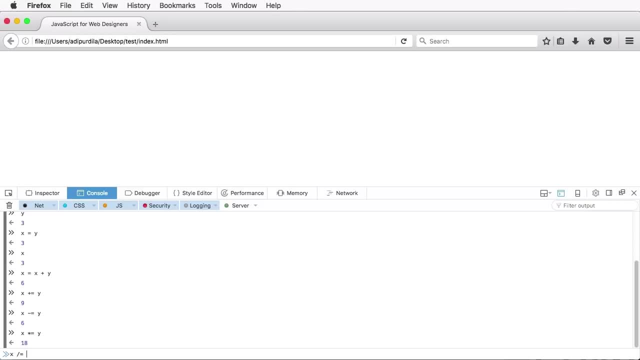 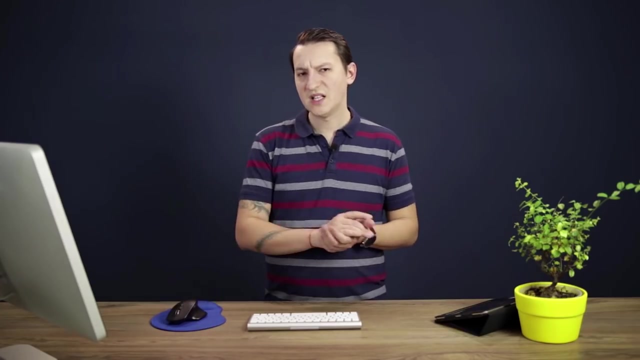 And the division will be x slash equal y And, just like the addition assignment, you can already deduce their full form. So, for example, For example, the subtraction is x equals x minus y. And that's a quick look at the assignment operator. 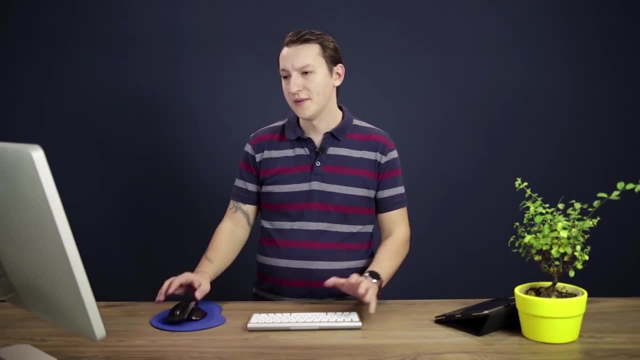 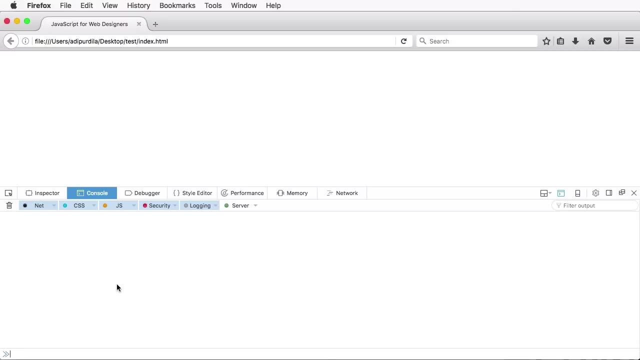 Now let's move on to the comparison and logical operators. And the comparison operator will basically compare its operands and return a Boolean value based on the result of that comparison. So if the comparison is true, it's gonna return true. If it's not, it's gonna return false. 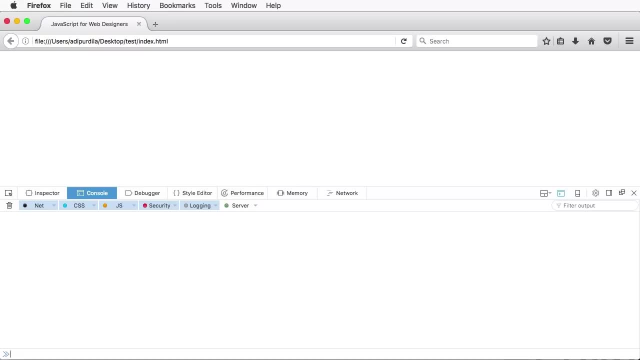 Now I'm sure you already know what the comparison operators are: It's equal to, it's greater than, smaller than greater than, or equal to, and so on and so forth. So you see where I'm going here. Let's see a few examples. 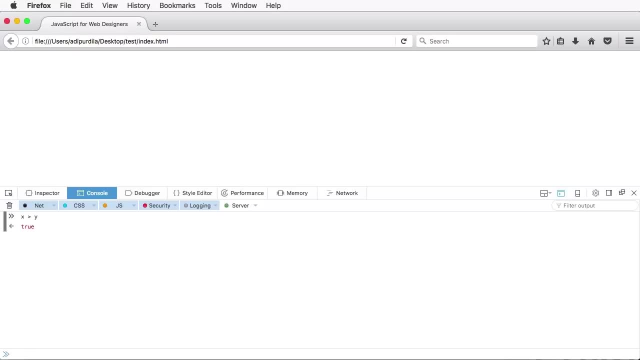 So if I say x is higher than y, it's gonna give me true, because currently x is 6, y is 3.. But if I say x equal to y, it's gonna give me false, because then it's gonna give me false. 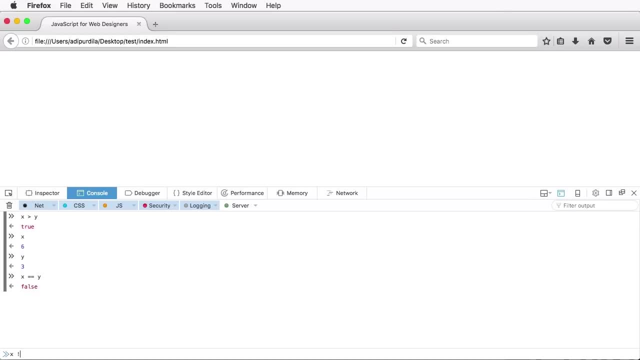 Those two values are not equal. I can also say x not equal to y and that's gonna return true. And there's also a strict equal that I wanna show you real quick. So if I say x, strict equal, so 3 equal signs y, it's gonna give me false. 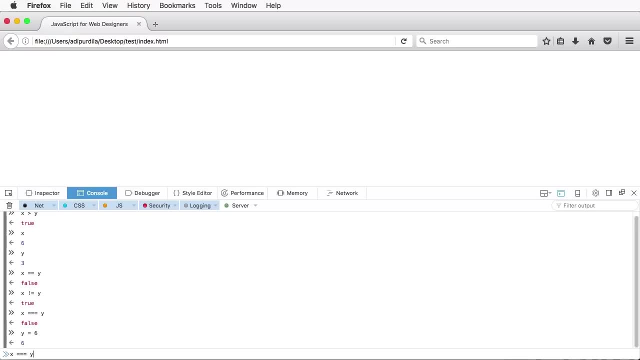 But if I set y to 6, and then I repeat, x strict equal y, it's gonna give me true. But what if I'm doing x equals 3? I'm doing x equals 6.. So instead of a number, I'm assigning a string to the y variable, right? 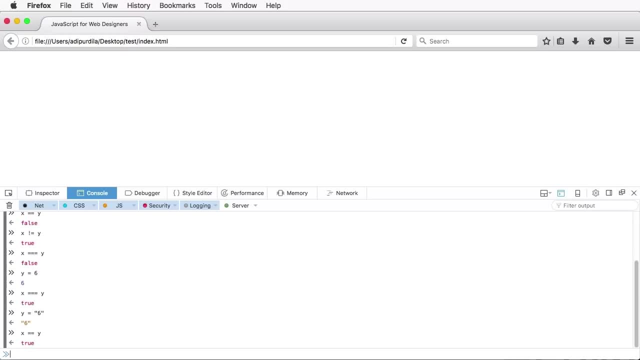 Then if I say x equals y, it's gonna give me true, because it's 6 and 6. But if I say x is strict equal y, it's gonna give me false. And that's because strict equals also considers the operant type. 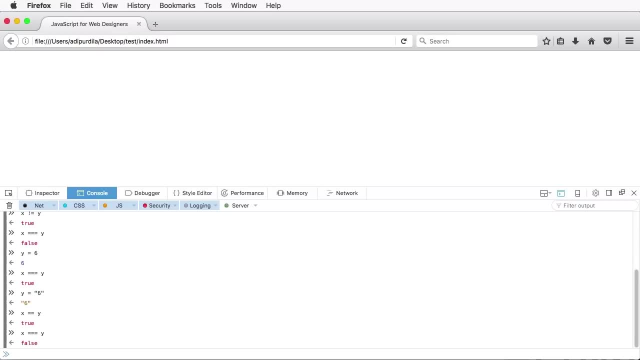 If you do, just is equal. so 2 equal signs it's just gonna compare the value, while strict equal is gonna look at the type as well. Now the logical operators are and, or and not So and let's say, for example, x equals true and y equals false. 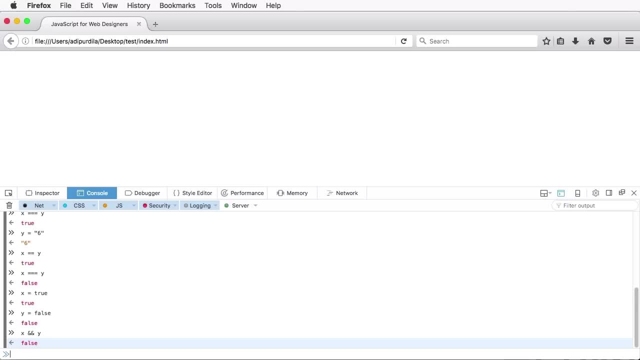 If I say x and y, it's gonna give me false, because the x and y are not equal And operator will return true if both operands are true. otherwise it's gonna return false. If I do x- excuse me- x or y, it's gonna give me true. 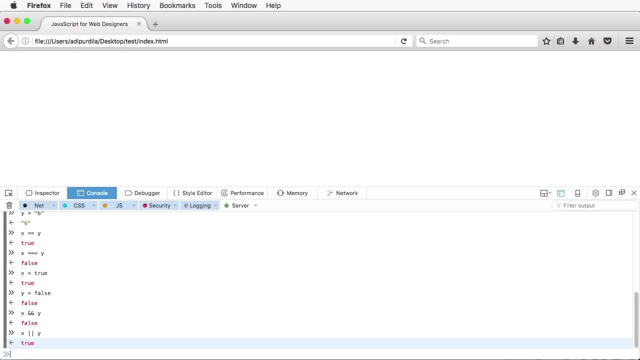 because the or logical operator will return true if either of the operands is true. If both are false, it's gonna return false. Finally, the logical not operator will not operator will basically switch things around. So x is currently true, but if I say not x, it's gonna return false. 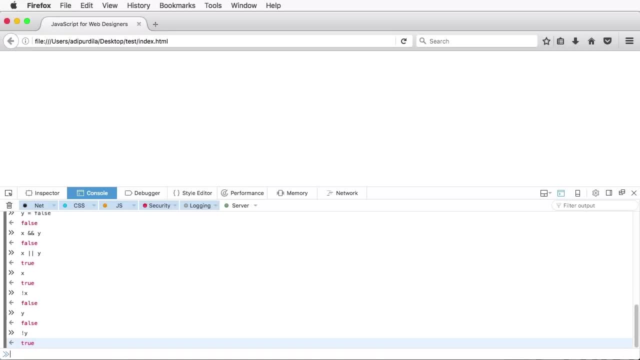 And y is currently false. So if I say not y, it's gonna give me true. Basically, the not operator is gonna return false If it's operant can be converted to true. Otherwise it's gonna return true. Now let's talk about the arithmetic operators. 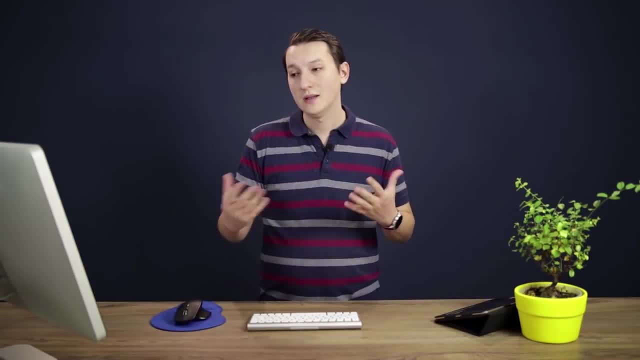 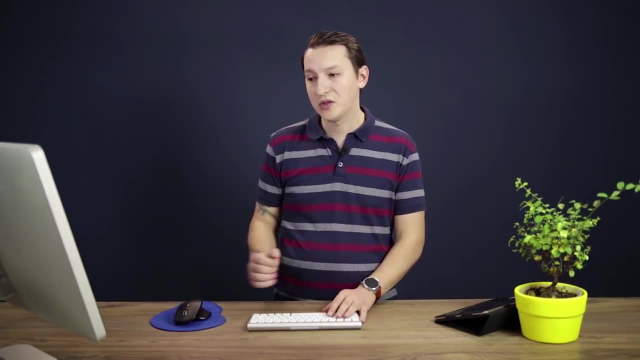 And you've already seen a few like plus minus. These are arithmetic operators, But there are a few that are a bit more special and I would like to show you those. So first of all, we're gonna talk about the increment operator. 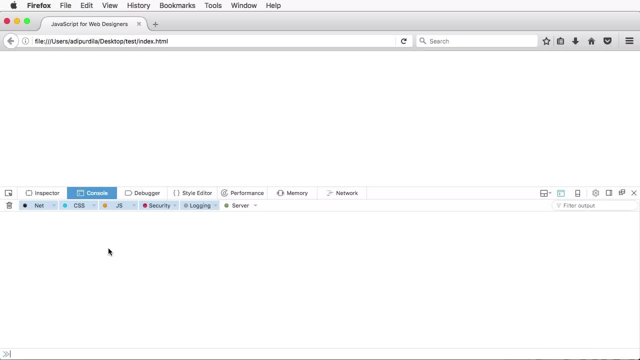 And this is a unary operator, which means it only needs one operand. It's not like, for example, the equal operator, which needs two operands, right? So the increment operator basically will add one to its operator and then it's gonna return, true? 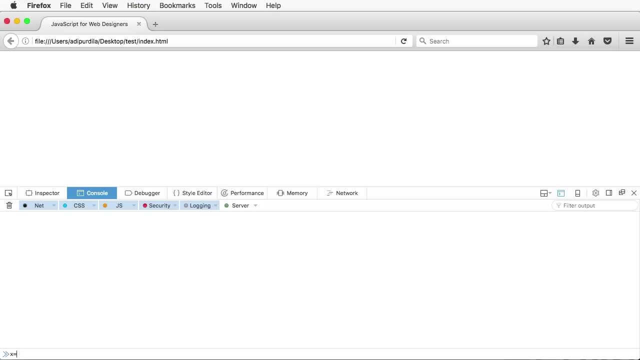 So if I say not y, it's gonna return true, It's operant. So, for example, if we set x to 3, and I say x++ and I read x after that, it's gonna give me 4.. So what happens is x++ will first print x and then it's gonna increment it by 1.. 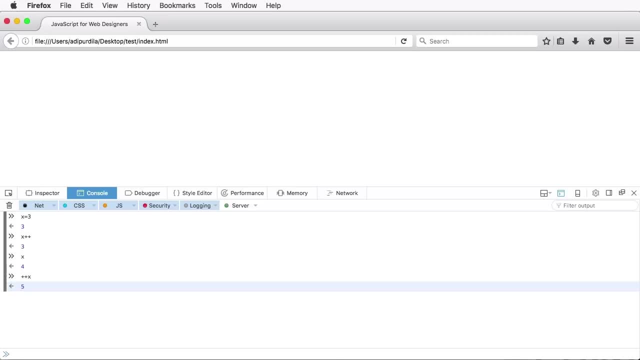 If I do plus plus x, it's gonna give me 5, because it's first gonna increment it and then it's gonna print it. Same goes with decrement, also a unary operation. Instead of adding 1 to its operand, it subtracts 1.. 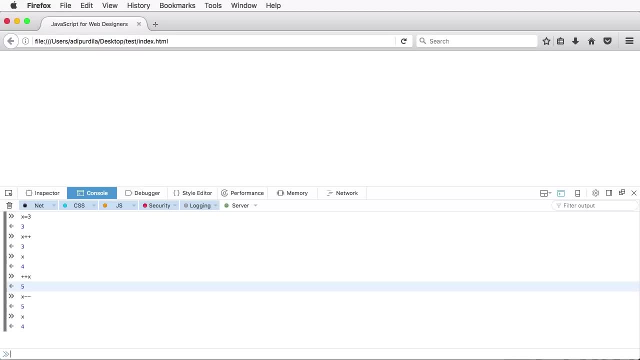 So if I say x minus minus x is gonna be equal to 4. And it also works the other way around: minus minus x. Now there is also a unary negation and unary plus, And the unary negation basically will return the negation of its operand. 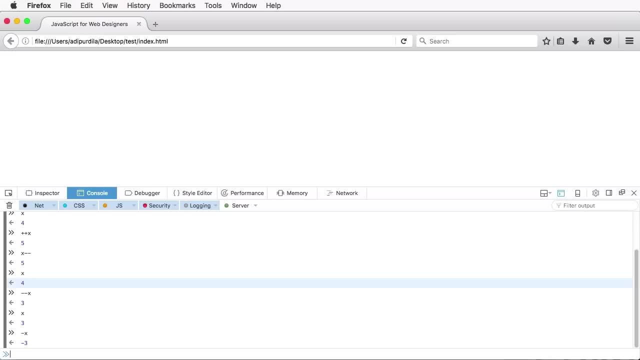 So x is currently 3.. If I say minus x, it's gonna give me minus x. So if I say minus x, it's gonna give me minus x. So if I say minus x, it's gonna give me minus x. 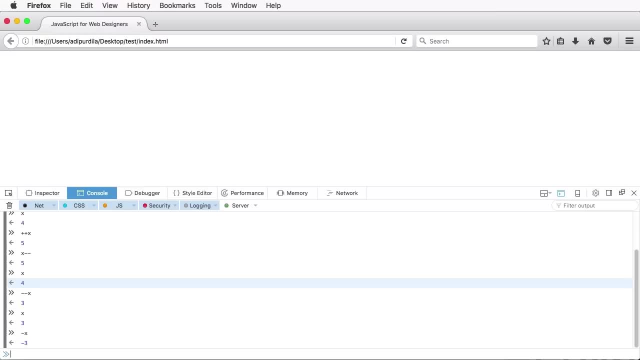 The unary plus will actually attempt to convert its operand to a number, if of course it's not already So. for example, plus 3 will give me 3.. But if I have plus and the string of 3, it's gonna give me 3.. 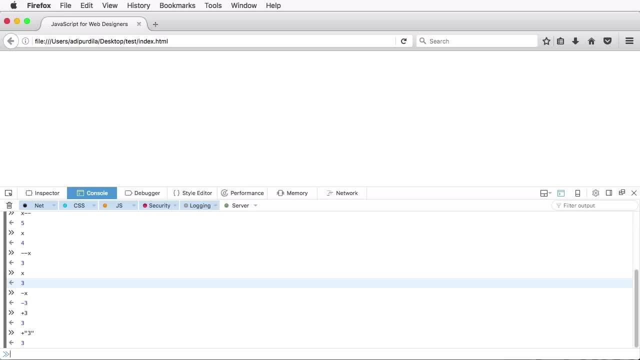 It's gonna transform that type into a number. If I say, for example, plus true, it's gonna give me 1.. Plus false is gonna give me 0, because 0 and 1 are considered false and true. Finally, we're gonna talk about the concatenation operator or the plus. 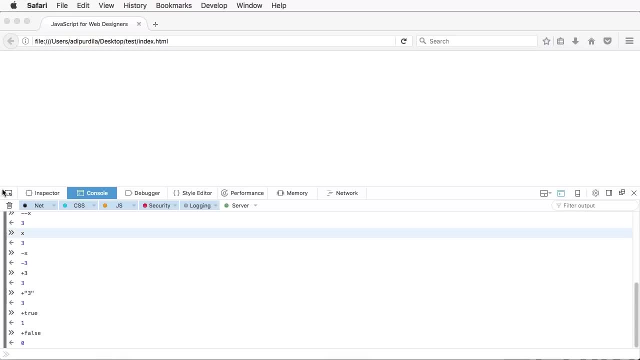 And that can be applied to a string. So, for example, if we're gonna set some strings here, For example, x equals hello and y is gonna equal to world, right, What I can do is say x plus y and that's gonna give me hello world. 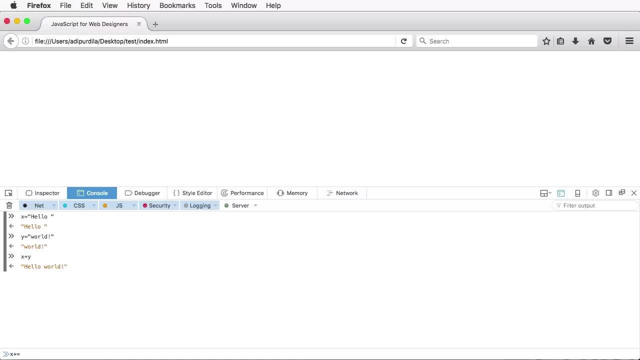 I can also do something like x plus equal and I can add another string to it. For example: hello again, and that's gonna give me hello, hello. And I can also do this: 32 plus 32, 32 is gonna give me that big string. 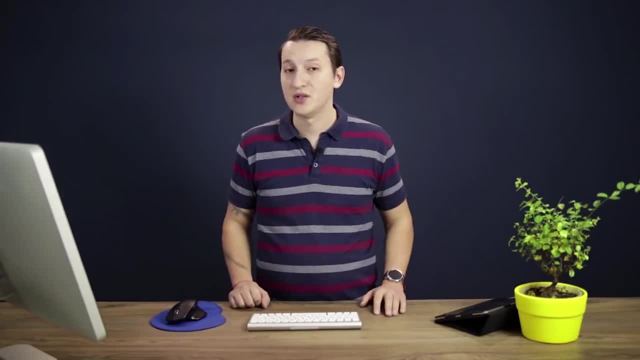 And that's a very quick look at operators in JavaScript. Now, the reason why I'm doing this is because it's gonna give me a string that's gonna give me a number. Now, the reason why I'm doing this is because it's gonna give me a number. There is a programming concept that is: 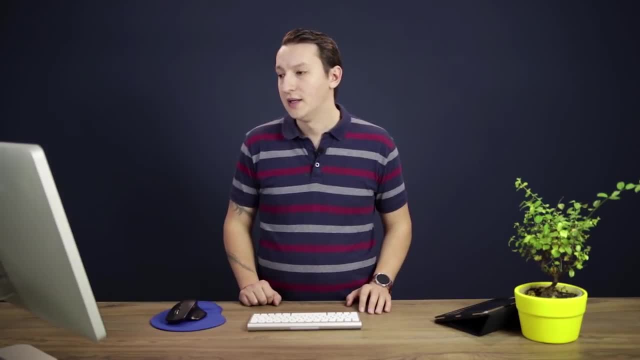 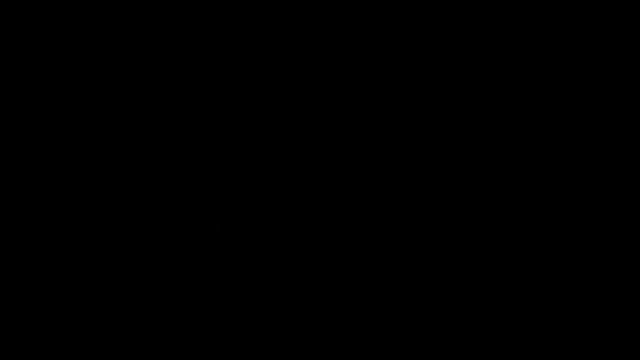 I think is essential for any kind of JavaScript developer, And that is the if else statement. Again, if you've done computer science in school, then you already know what that is, But we're gonna cover that in the next lesson. See you there. 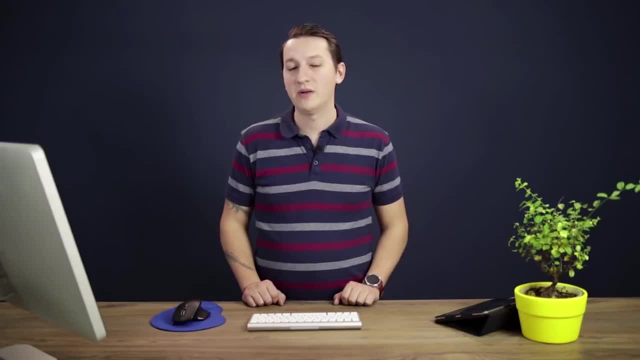 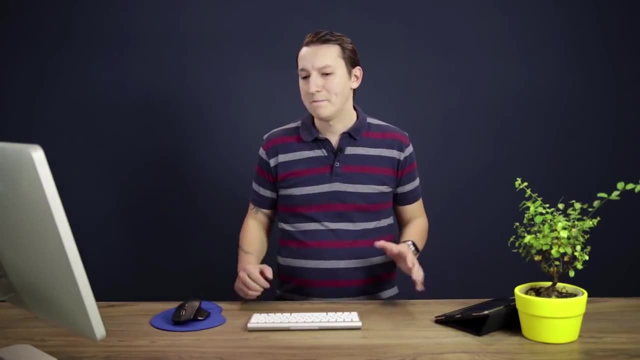 Hello and welcome to lesson number seven, where you'll learn about the if else statement Now, and this is something essential for any kind of programmer- And the if else statement allows you to execute various blocks of code if a specific condition is met. 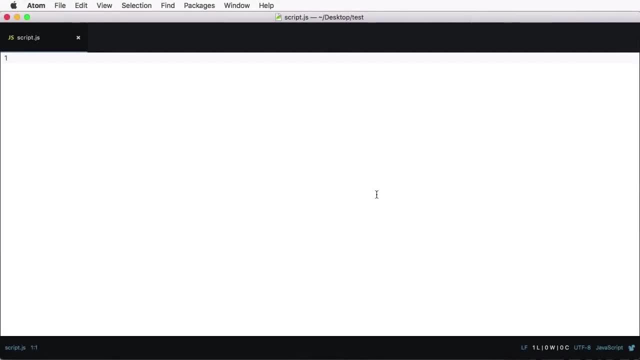 So first let's have a look at the if statement. So this index is very simple if we open some parentheses And in here we put a condition. So let's begin by declaring a variable: x equals 5.. 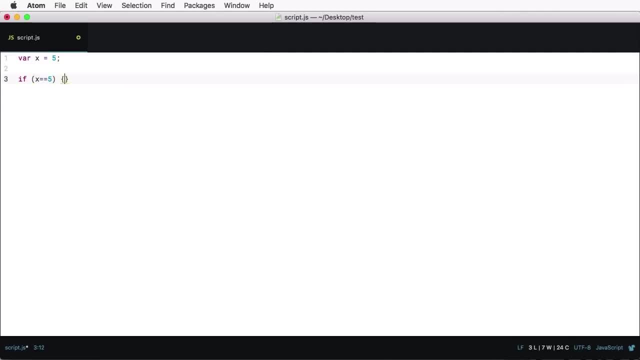 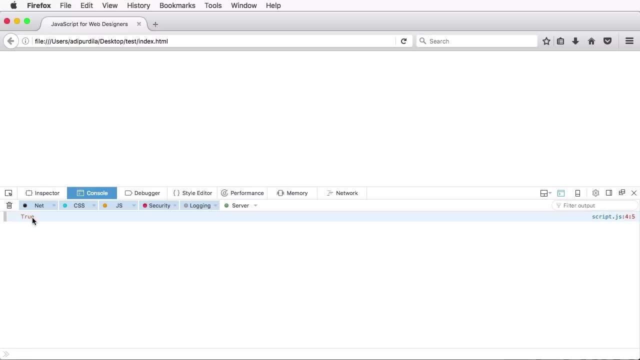 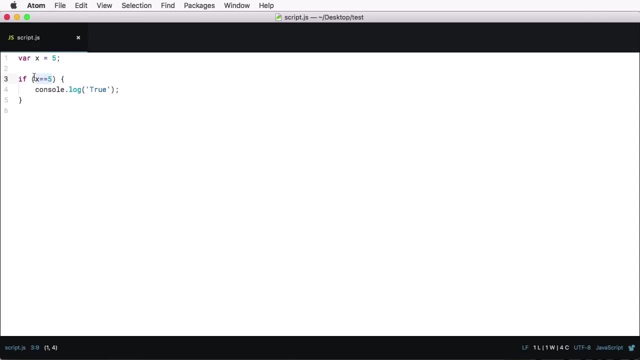 And I can say: if x equals 5, then we're gonna do a console log, true. And if I do a refresh, I get a console log of true. Now what happens here is first: JavaScript evaluates this expression: Is x equal to 5?? 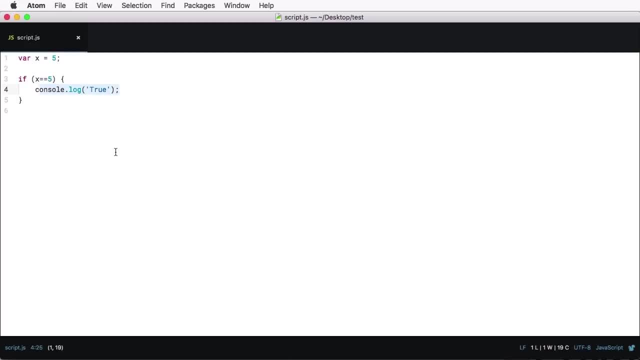 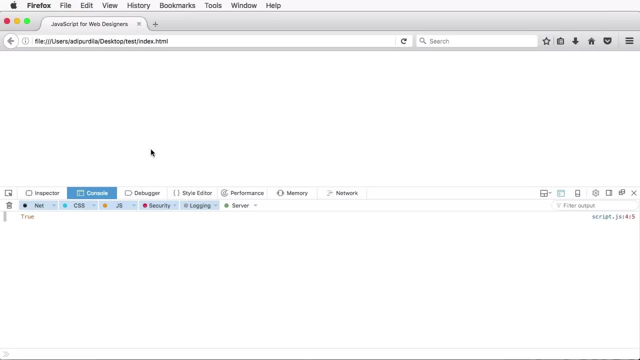 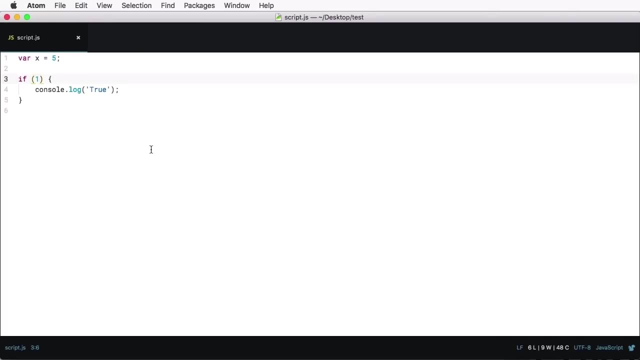 Yes, it is. If true, then we do the console log. So it's the same thing as saying if true, It's gonna have the same result. Or if 1,, 1 is also interpreted as true. But if I say if x equals to 51, for example, 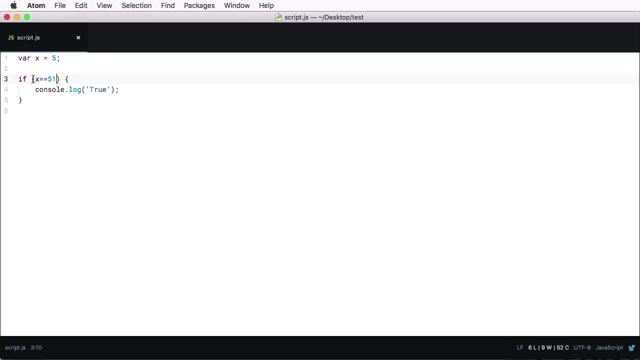 nothing's gonna happen because this condition is gonna be evaluated. It's gonna be evaluated to false, actually, and the code inside the curly brackets is not gonna be run. Well, in that case we can specify else. So if this condition is not met, then we do this. 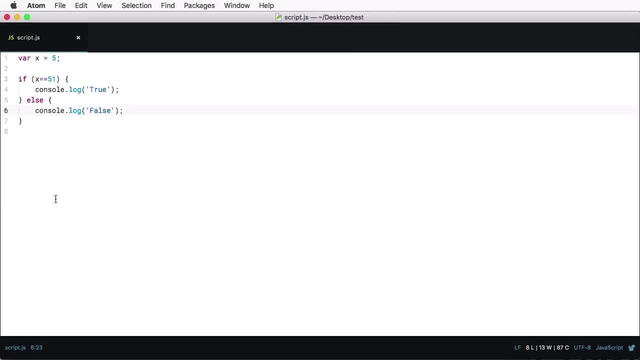 And I'm gonna say console log false. And you can actually chain these together, right? Let's make a better example here. Let's say: age var, age equals 24, right? So we're gonna say: if age is smaller than, let's say, 20.. 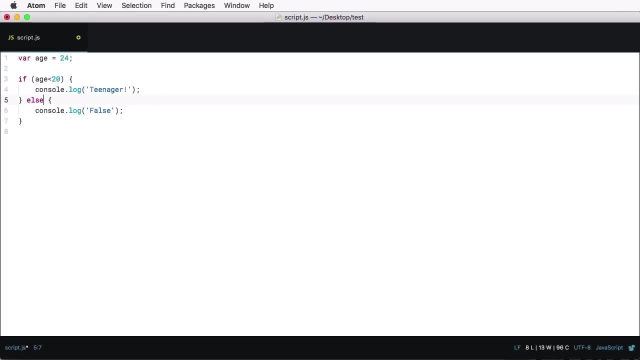 We're gonna log to the console teenager. Else, if age is higher or equal than 20, and age equals smaller than 70, then we're gonna log a young man, Else we're gonna log not so young anymore. So let's see. 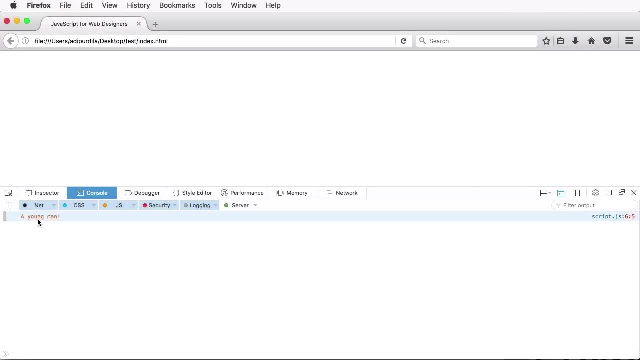 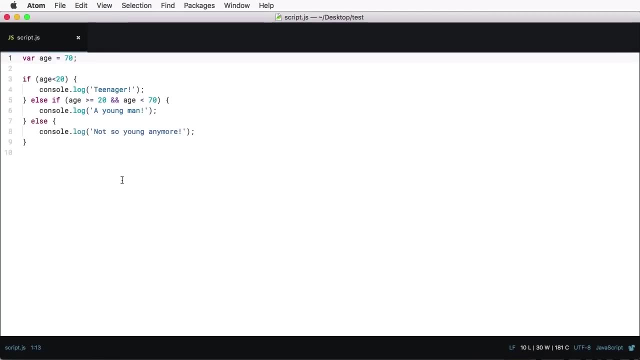 Let's see what happens. If I do a refresh, it tells me I'm a young man. But if I change my age here to, for example, 70, it tells me that I'm not so young anymore, Because 70 doesn't actually fall in these two categories. 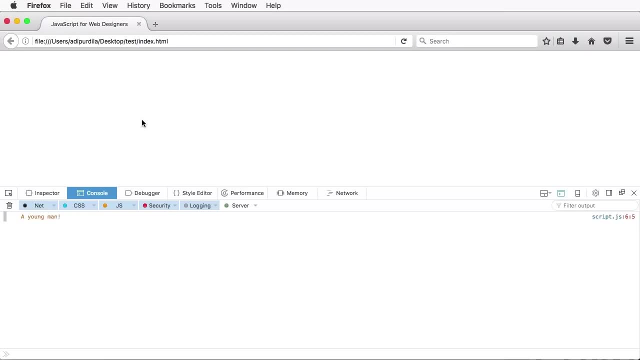 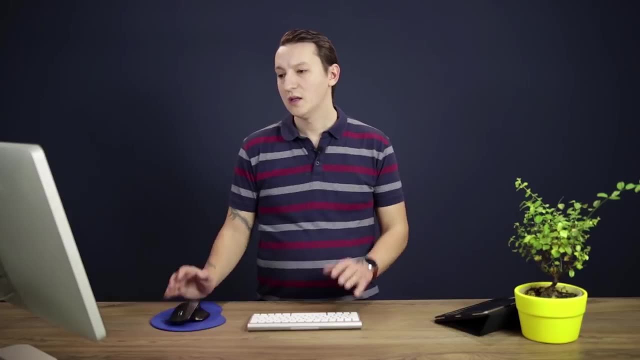 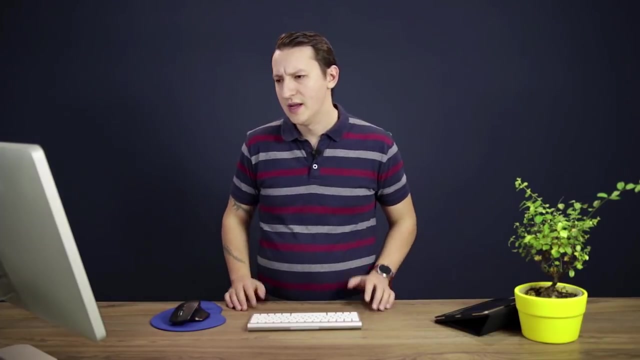 If I would say smaller or equal than 70,, it's gonna still say I'm a young man. So this is how the if else statement works. Now, finally, I want to show you another operator that's called the ternary operator or a conditional operator. 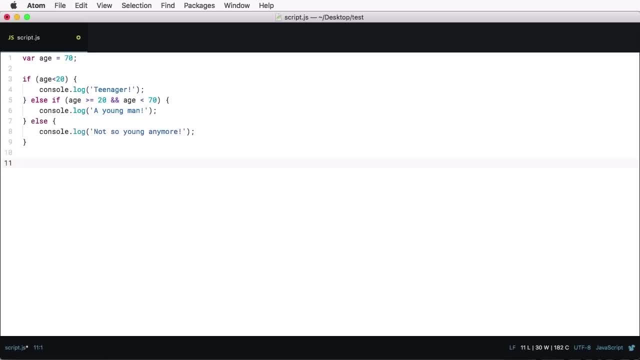 And that goes something like this: This is actually a special case because it's the only JavaScript operator that takes three operands And let's do a simple. if else, I'm gonna say: if age is higher than 20, then I'm gonna consolelog: not a teen anymore. 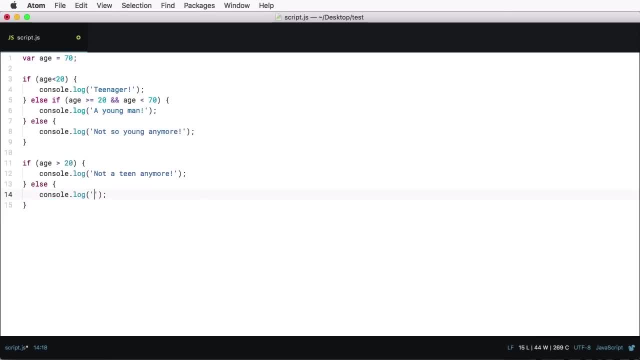 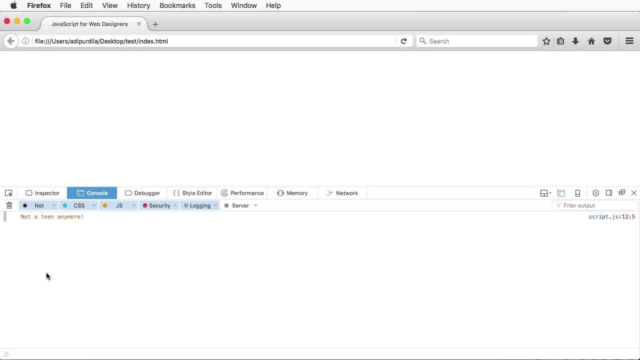 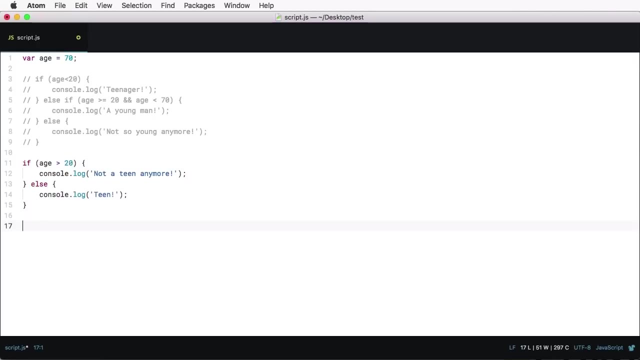 And I'm gonna do else. Consolelog teen and I'll just comment this bit, okay. So now it tells me not a teen anymore. Well, this I can actually compress to this Age, higher than 20, question mark: consolelog, not a teen anymore. 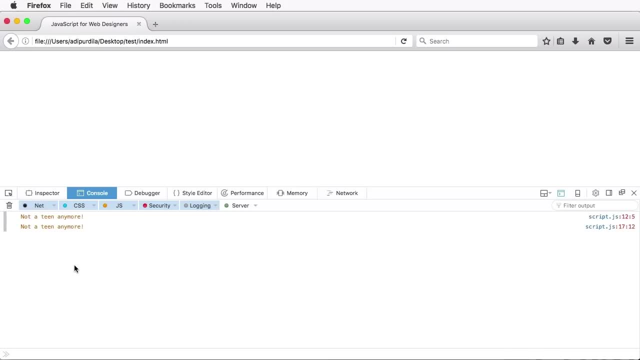 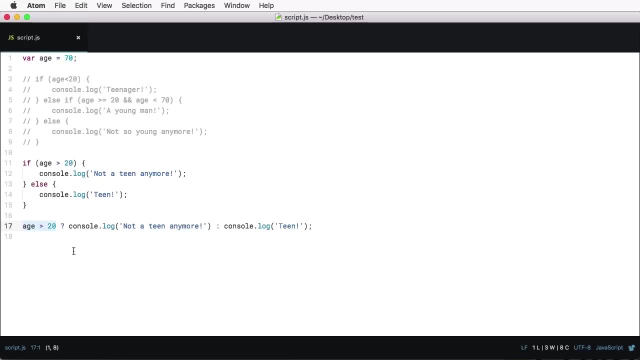 colon consolelog teen. And let's see, it does exactly the same thing. And this is the way it works: The expression- the expression here or the condition- is evaluated And if it's true, we're gonna execute the code after the question mark. 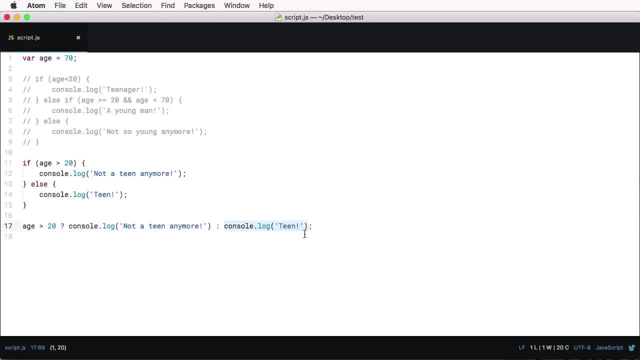 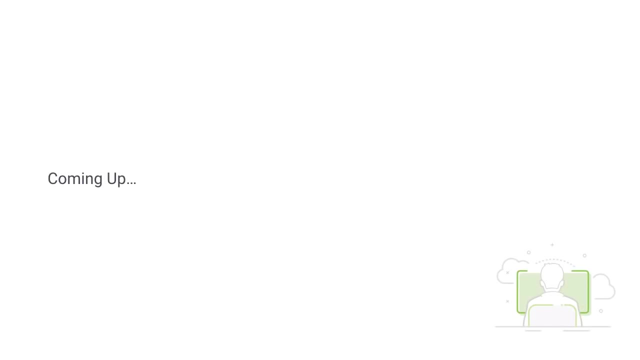 If it's not true, we're gonna execute this code. So a more simple version would be this: condition: val1, val2.. So if this is true, execute this. otherwise, execute this, And that's how you can use the if else statement. 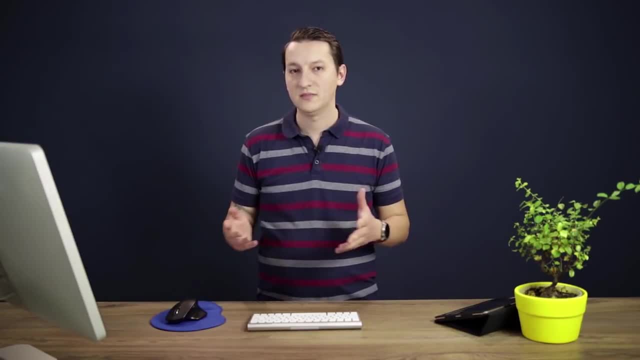 Now let's move on and talk about loops. That's coming up next. Hello and welcome to lesson number eight, where you'll learn about loops in JavaScript. Well, a loop is a piece of code that executes repeatedly, either a set number of times or until a certain condition is met. 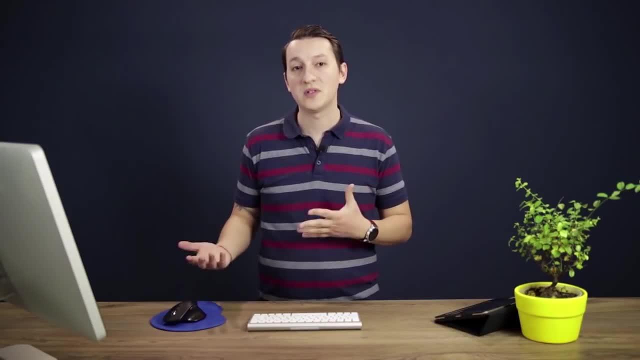 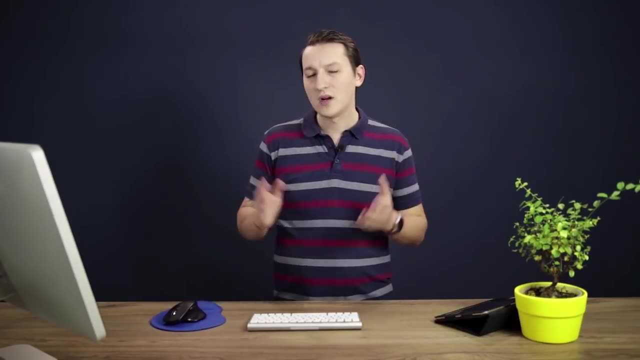 And if you've worked with Sass and you've used the, the for each and while directives, then you already know what loops are all about. Now, when it comes to JavaScript, we have three types, well, three main types of loops. 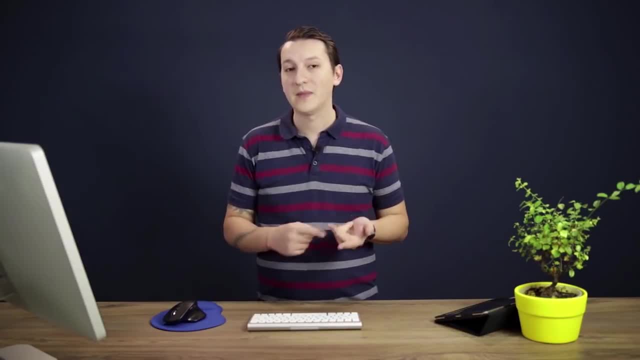 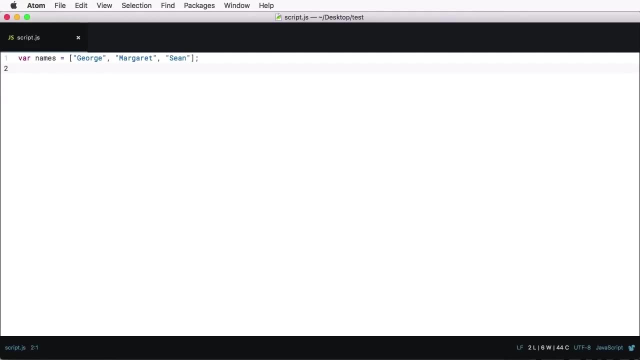 We have the for, we have the do while and we have the while. So let's begin with the for loop. A for loop will repeat until a specified condition evaluates to false And we go something like this: for We open some parentheses, then we'll have an initial expression. 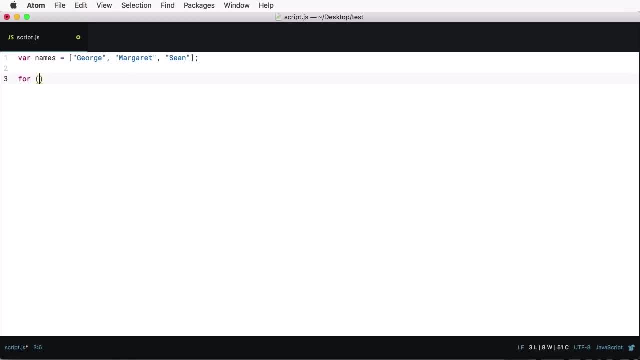 Now the initial expression can be or is mostly used to initialize a variable or a counter. So for example, I can say: var x equals 1. And then I'm gonna do a semicolon and that follows the condition. Now the condition is the thing that's gonna be evaluated. 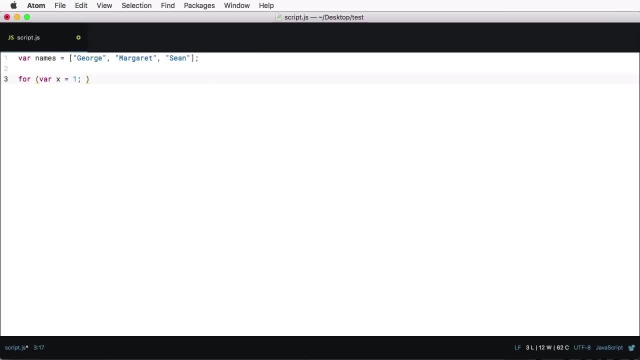 And if that value of the condition is true, then the loop will execute, or the loop statement. If the value is false, then the loop terminates. So, for example, let's say x is gonna be smaller than 10, and I'm gonna do a semicolon again. 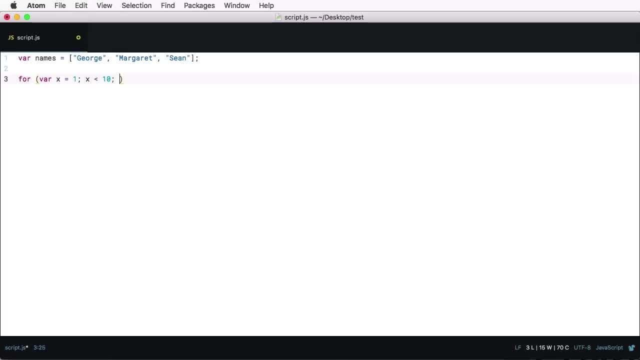 And then, third, we have the incremental expression, And this is usually used to increment the counter. So I can say, for example, x++. we're gonna open some curly braces and we're gonna have the main statement or the block of code that's gonna be executed. 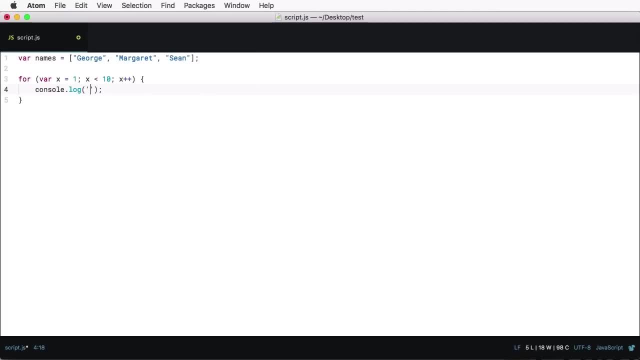 So let's say, for example, that I'm gonna do a consolelog for x and that's gonna be printing nine numbers in the console, from one to nine. Now if I say x smaller or equal than 10, it's gonna print 10 of them. 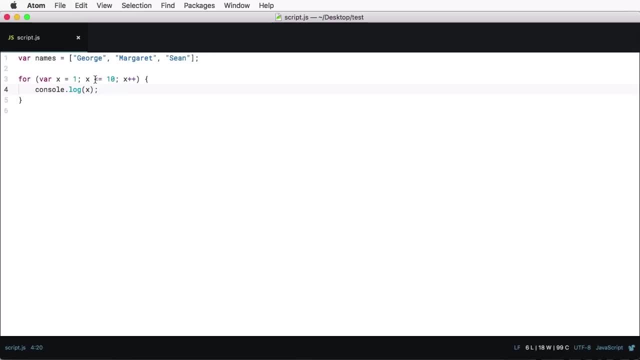 because the condition evaluates to true when we reach number 10.. Now if you're wondering: well, what can I use loops for? Well, you can use them for a bunch of different things. For example, we have that names array. 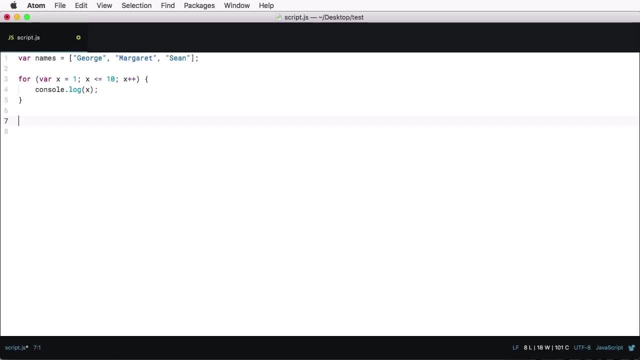 What if we want to print all of the names in that array? Well, we can do something very simple. For example, for var x, or you can call it whatever you want- y equals 0. We're starting from 0, because an array's index is 0 based. 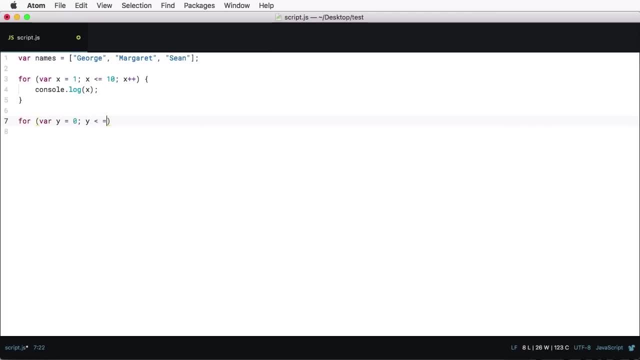 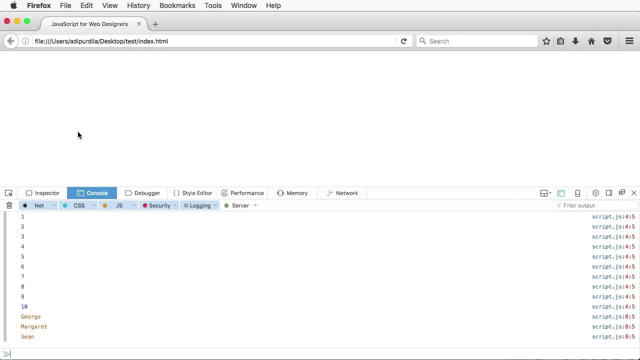 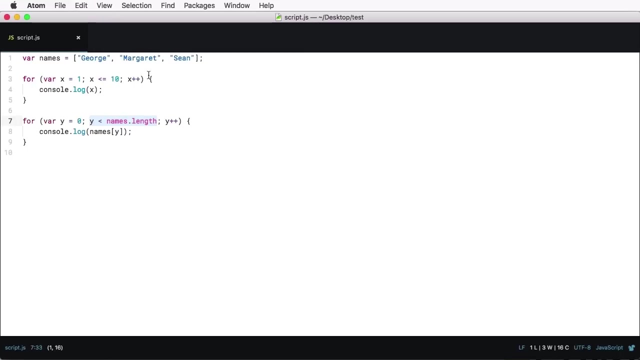 So we're gonna say y is smaller than nameslength y++, And then we simply do consolelog names of y And that's gonna print George, Margaret and Sean. So what I did here: I started from 0.. I'm going up until nameslength, which in my case is 3.. 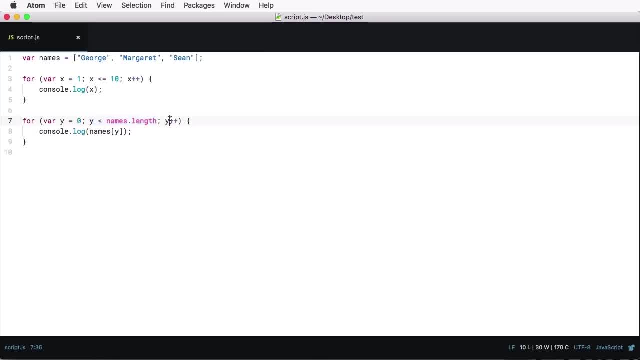 So we're going 0,, 1, and 2.. We're incrementing y as we go along and we're outputting those names to the console. Next let's move on to the do-while statement, And the do-while statement will repeat until a specific condition evaluates to false. 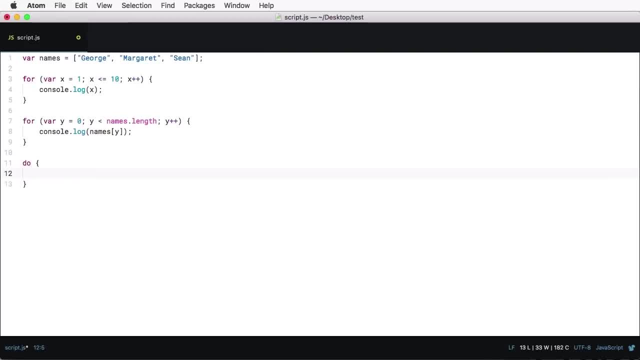 And a do-while statement looks something like this: Do, and we'll have the statement here while and we'll type our condition. So, for example, let's declare a variable here called x equals. now let's actually delete the 4.. 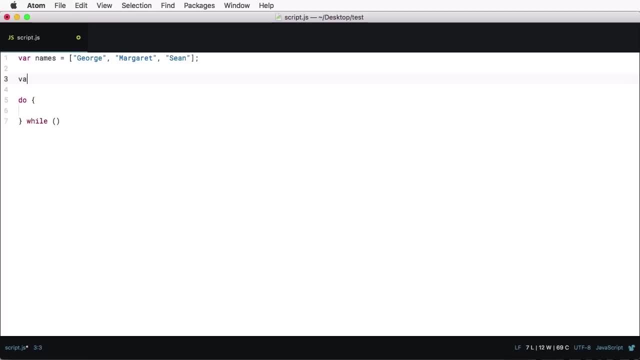 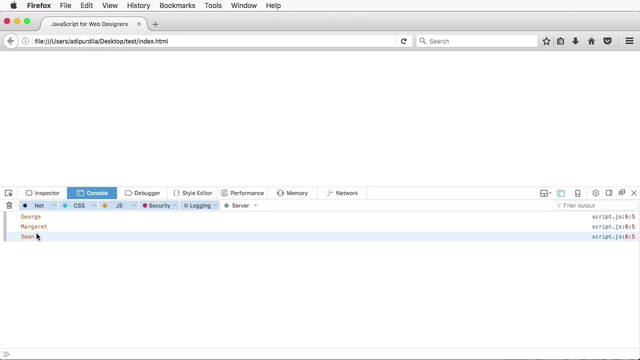 Yeah, we're gonna do var x 0.. So we're gonna do consolelog names of x, we're gonna do x++, And we're gonna do this while x is smaller than nameslength, And this will print George, Margaret and Sean. 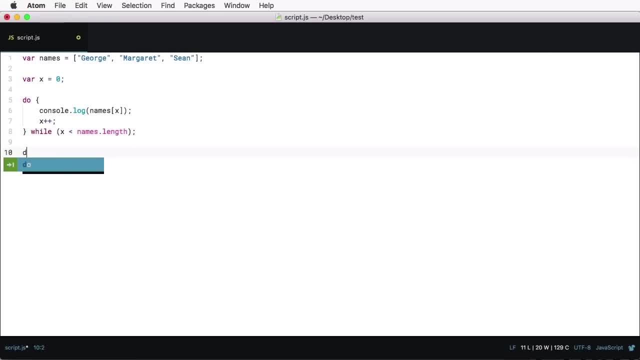 But let me show you another example. Let's say that we have x. Let's say that we have x. Let's say that we have a do-while statement that looks something like this: Do consolelog x, while x is higher than 0.. 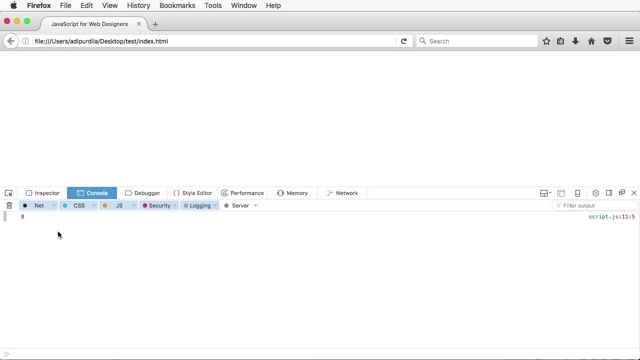 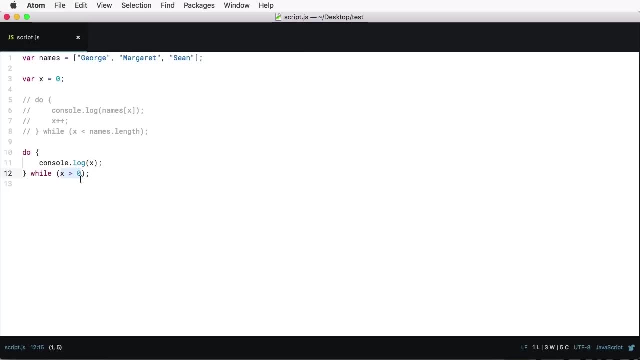 And let's actually comment this bit And refresh it- prints 0.. Now why is this happening? Because x is 0, so this condition here is not met. Well, that's what do-while does. The statement is executed, at least. 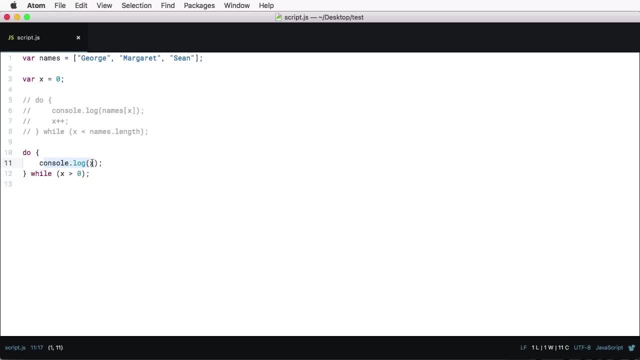 once, regardless of how the condition is or to what the condition is evaluated to. Now, on the flip side, we have the while statement, which is very similar to this. The only difference is the while statement will execute or the while loop will execute the statement only if the condition is met. 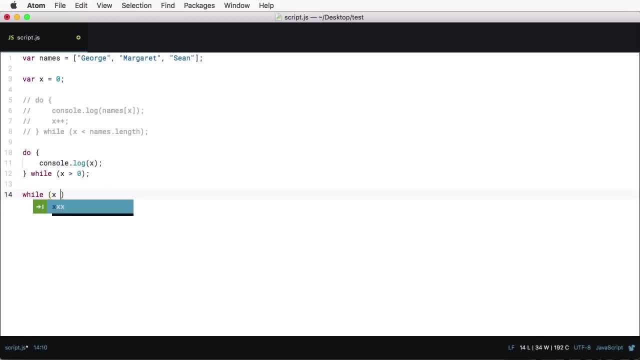 So, for example, we have while x higher than 0.. While x higher than 0, we're gonna consolelog x And if we're gonna comment this and refresh, we have nothing. That statement, consolelog x, has not been executed. 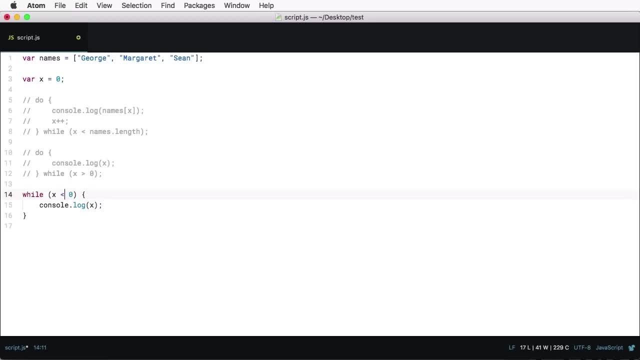 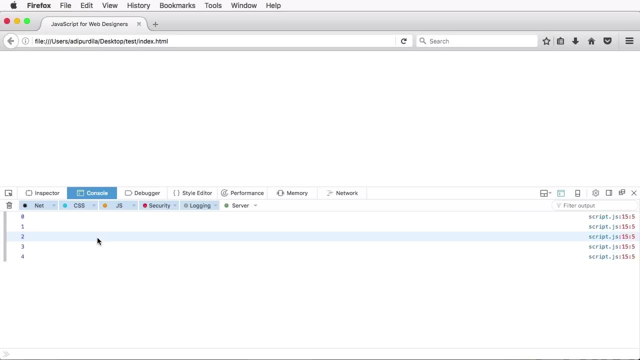 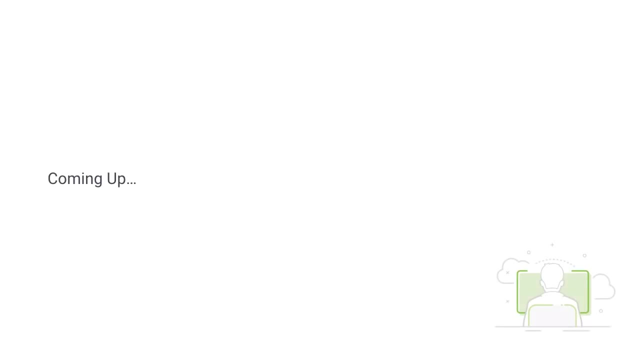 But if we do, while x is smaller than 5, and we do consolelog x++, we're gonna get this result. That's the difference Between do-while and while Now. have you ever heard of mixins and CSS preprocessors? 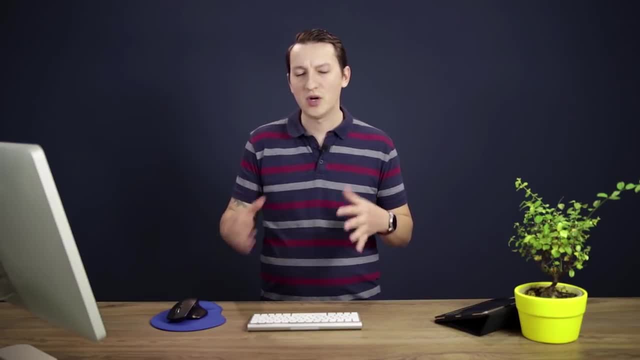 Well, if you have, then you should know that JavaScript and pretty much every programming language out there has something called functions, And functions are very interesting, very cool. You can do lots of things with them, and we'll learn about them in the next lesson. 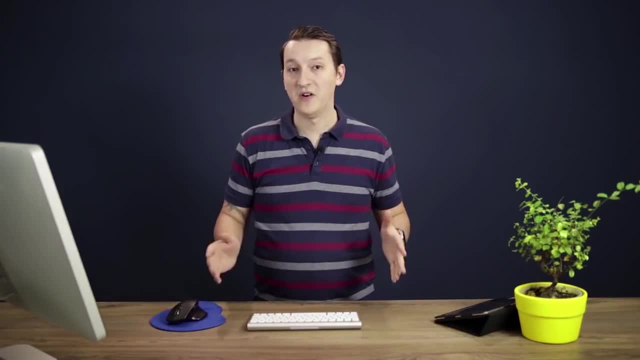 Hello and welcome to lesson number two, Lesson number nine, where we'll talk about functions. You can think about functions as sub-programs that can have their own name, can be called any time, they can receive parameters and they can also return values. 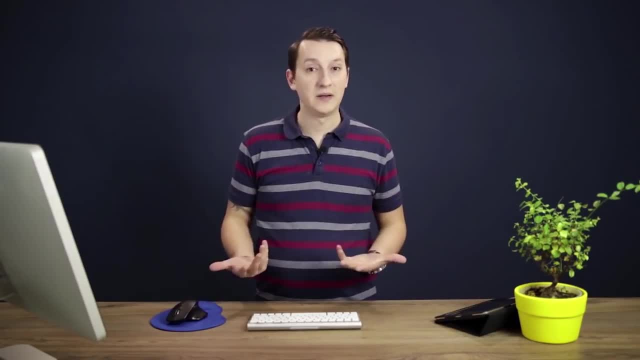 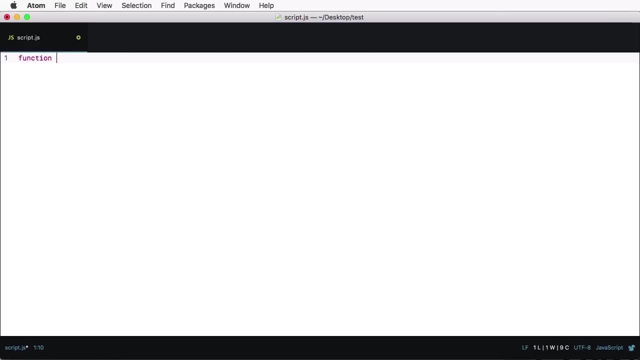 Now, to work with functions, you must first declare a function, And you do that with the keyword function. then you would give that function a name. So to give you a very simple example, here's two of those You're gonna find. say: this is a function. 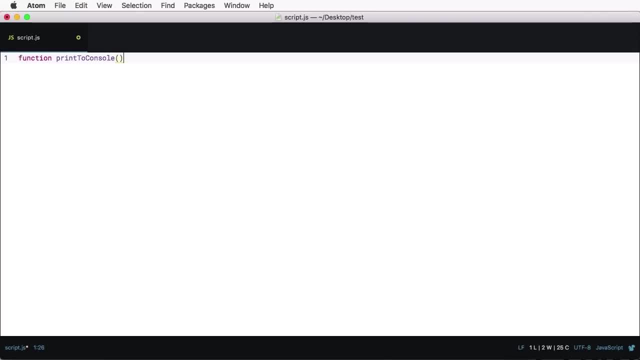 let's say print to console, and then you would open parentheses And in the parentheses you can specify a list of parameters that it can then pass on to the function. So let's for example, say: message here, And we can open our curly brackets and then inside 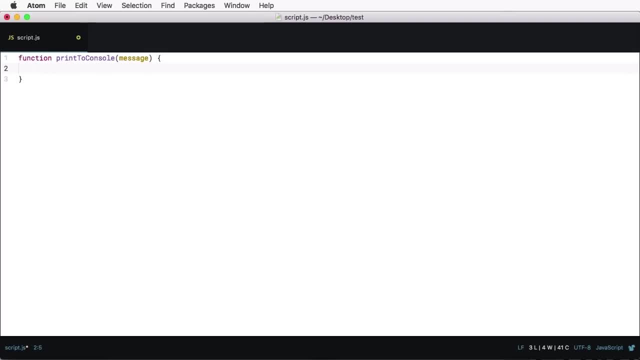 you would put the code that's gonna be executed by the function. Let's do, for example, console log message, right? So then what I can do is say print to console and I can pass in hello, and that's gonna print hello. 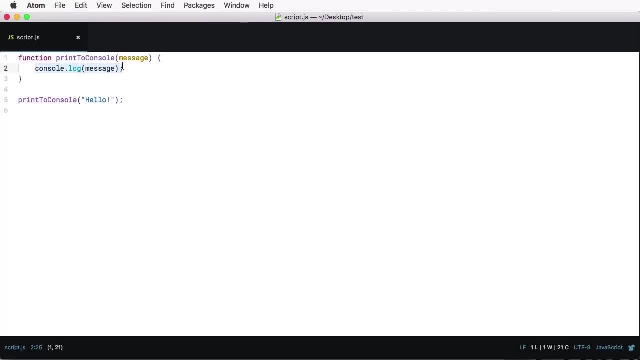 Of course this is redundant, because console log can already do this. We don't need an extra function for that. but I just wanted to show what you can do with that function. I can also do something like this. I can, for example, function add and: 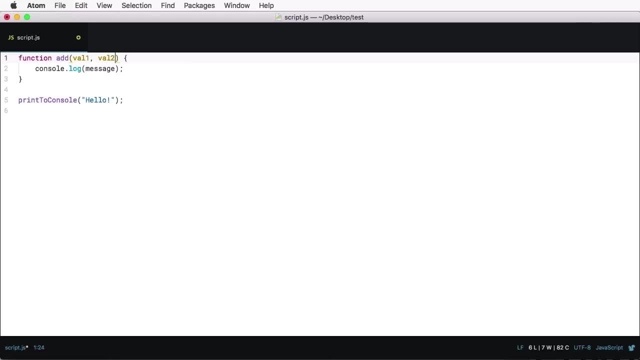 I can say value right, Value 1,, value 2.. I can do a console log of val1 plus val2.. And in here I can pass: for example I can say add 45 and 2. And that's gonna print 47 to the console. 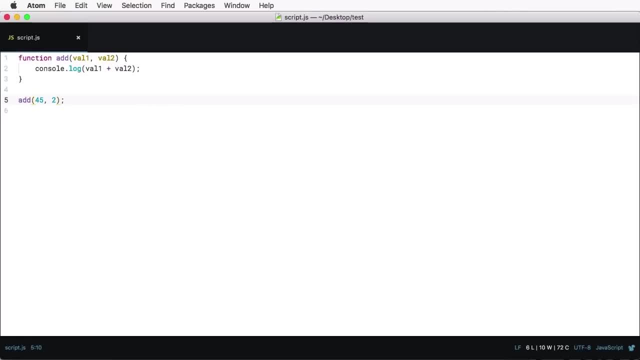 As I was saying, functions can also return values. So, for example, instead of doing a console log here, I can simply return val1 plus val2.. And then what I can do is say console log: add 45 and 2. And that's gonna print the exact same thing. 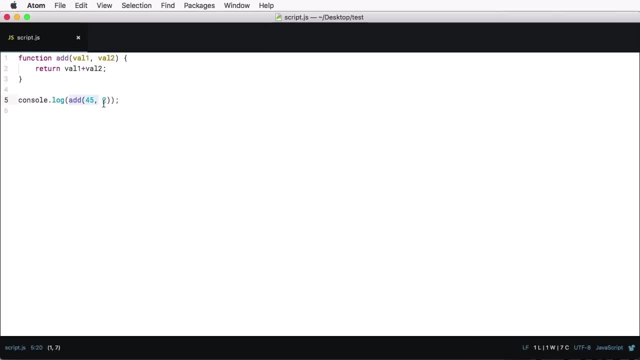 So I'm basically saying console log, I'm calling this function, I'm passing in 45 and 2. And then I'm using the value that the function returns And I'm gonna print it to the console. So that's how functions work. 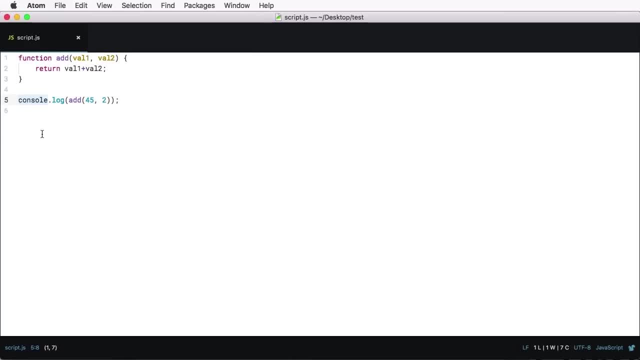 Really, it's very, very simple. Now. functions can also be declared like this: For example, let's do the square of a number, So we're gonna say square equals function And we're gonna pass in a number, And then we're simply going to return number multiplied by number. 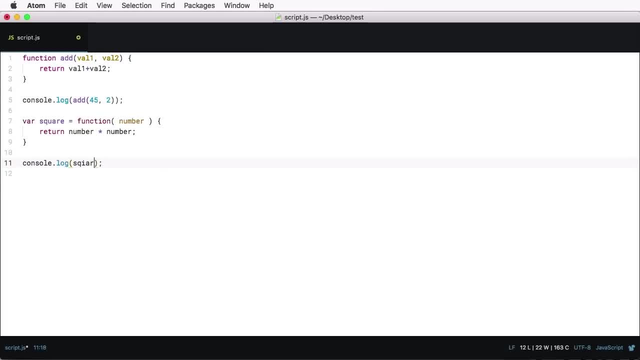 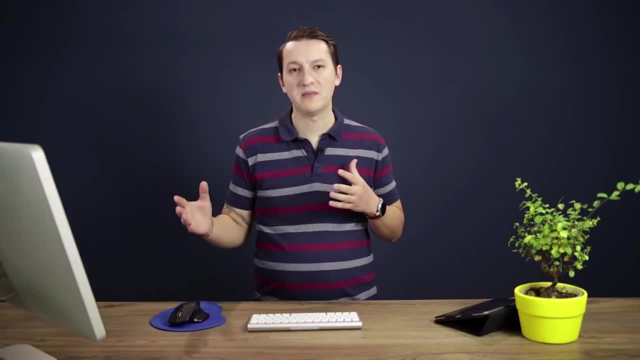 So, for example, if we say console log Square two, it's gonna print out four. Now, before we wrap things up with functions, I wanna talk about something that I mentioned when we talked about variables, And that is variable scope. Back then I said that variable scope means the context in which 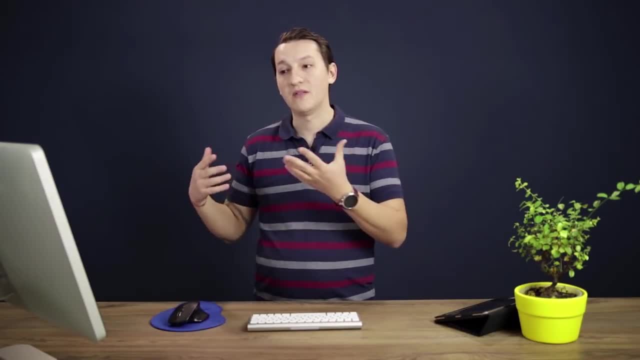 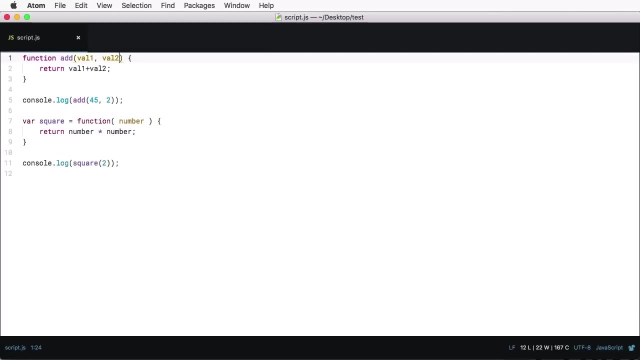 that variable is available, And we have global variables and we have local variables. So now that we got to functions, I think this is a pretty good time to do that, So I'm gonna go ahead and do that. So, for example, let's say, var x equals 3.. 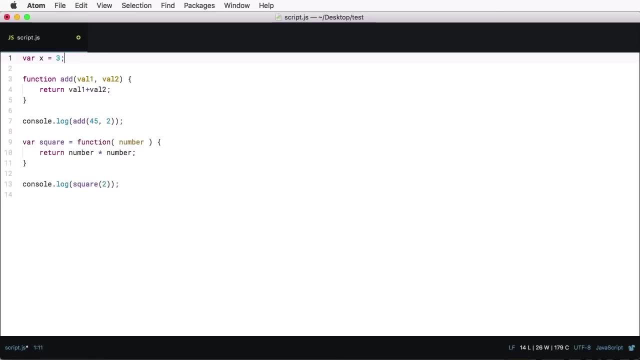 Now this is defined in the global scope, It's not inside any kind of block code And that means the variable x is available anywhere. So, for example, if I say a function test and I will simply do a console log of x. 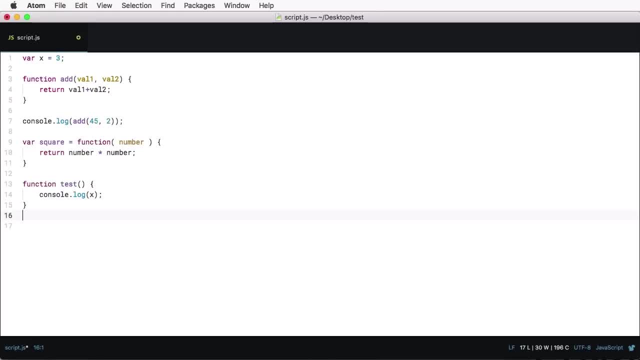 And then I call it- let me actually clean this up a little bit here- And then I call test, that's gonna print 3.. Now let's say I have another function here and we're gonna call this test2.. And let's declare a y variable in here. that's gonna be equal to 5.. 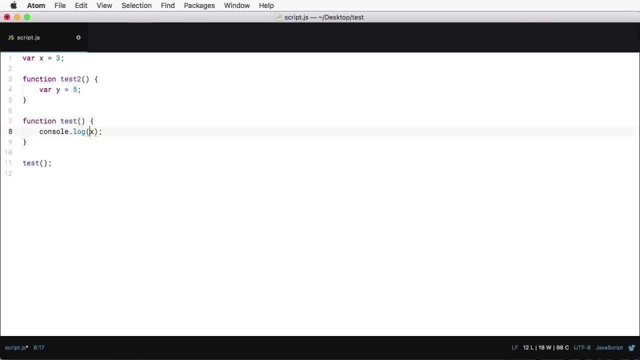 Well, if I'm gonna go into test and I'm gonna say consolelog, It's gonna tell me that y is not there, It's not defined. But if I do the exact same test in the test2 function, Let's uncomment this and let's call test2.. 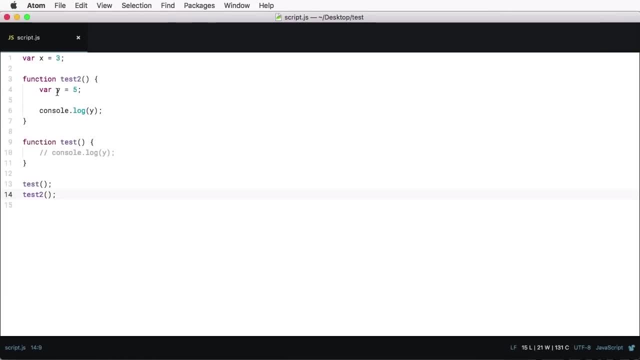 It's gonna give me 5.. So the variable y is only available in the scope of this function. It's not available anywhere else, like the x variable, which is global. Also, let's do something like this: We're gonna say: var x equals 3.. 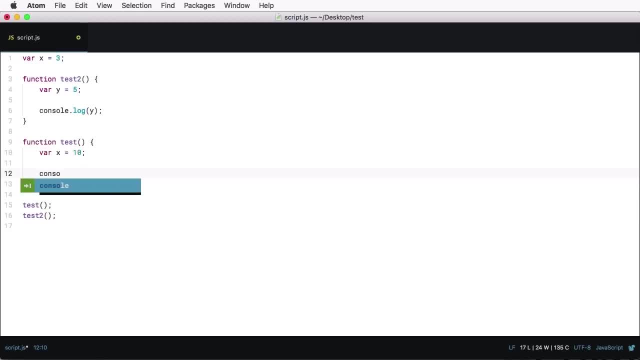 And we're gonna do a consolelog of x here And also a consolelog of x here. So first we're executing test and we're doing a consolelog of x And then we're doing a consolelog of x in the global scope. 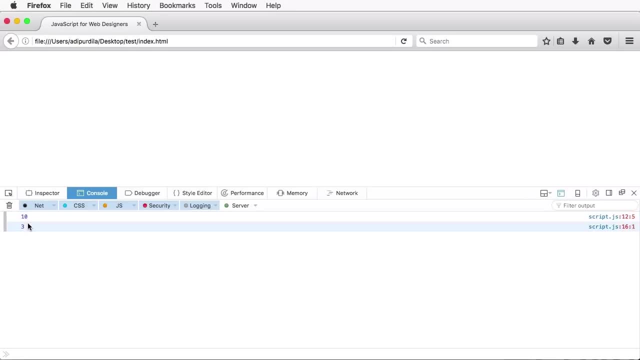 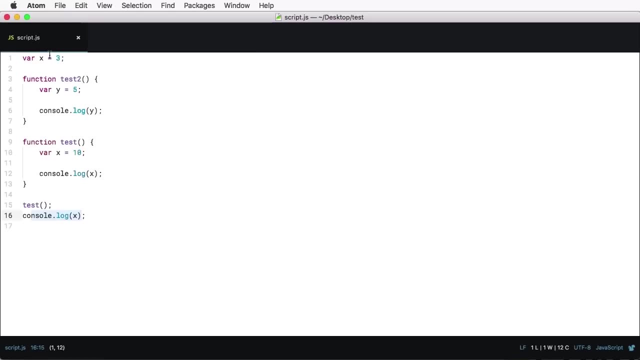 So now, if we refresh, we have two values: 10 and 3.. Even though the variable is called x, it has different values in different scopes. The global variable is called, has the value of 3, and it's only available here. 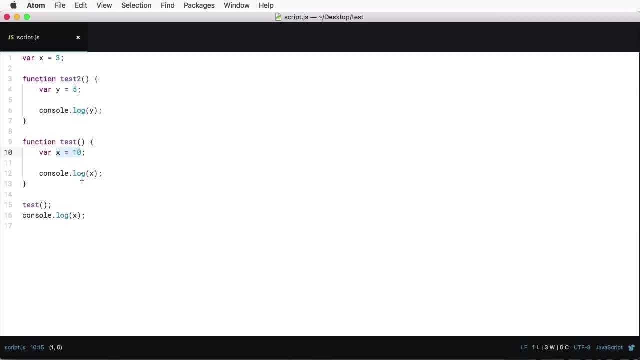 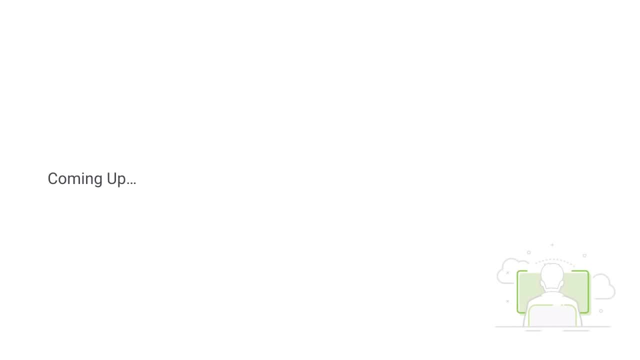 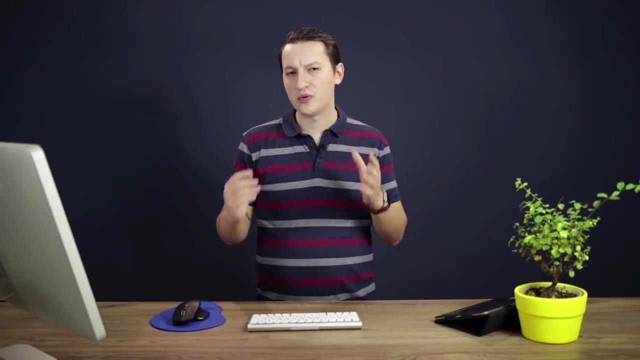 And this x variable has a value of 10.. So this consolelog actually prints this one, not the global one, And that's a very quick introduction to functions. Now, as a web designer, probably one of the main things you'll be using JavaScript for is to manipulate the DOM. 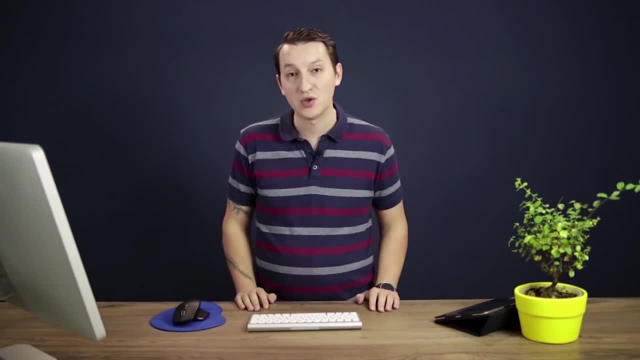 or the Document Object Model- essentially your web page- And the easiest way to do that is with the help of selectors. That's what we'll be learning in the next lesson. Hello and welcome to lesson number 10, where we'll talk about selectors. 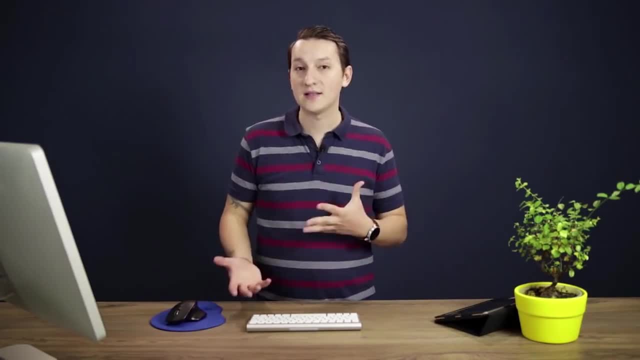 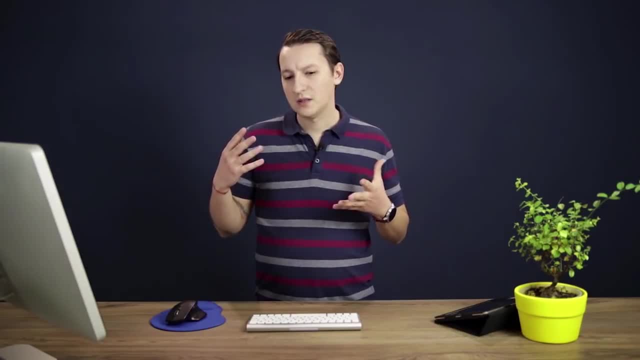 they also give you access to the DOM and allow you to manipulate it even. And these selectors are tied really well into the document and window objects And if you remember from the objects lesson, an object is a collection of properties, basically of properties and methods. 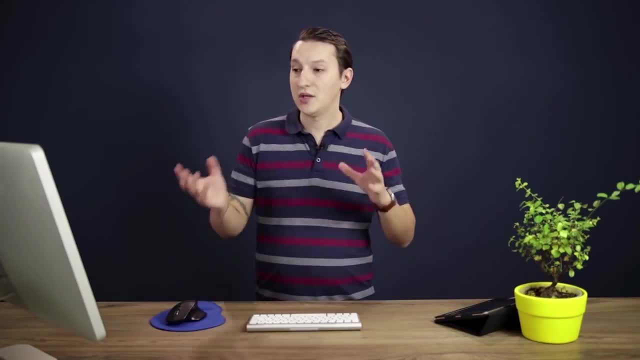 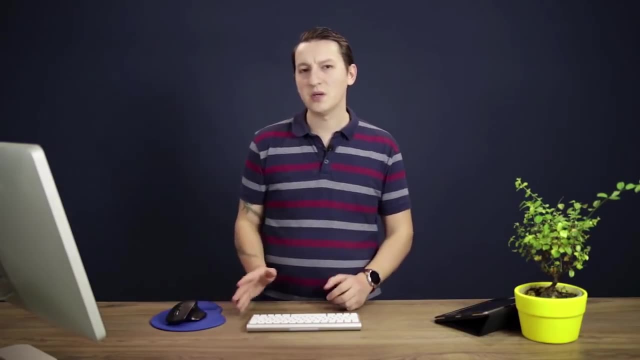 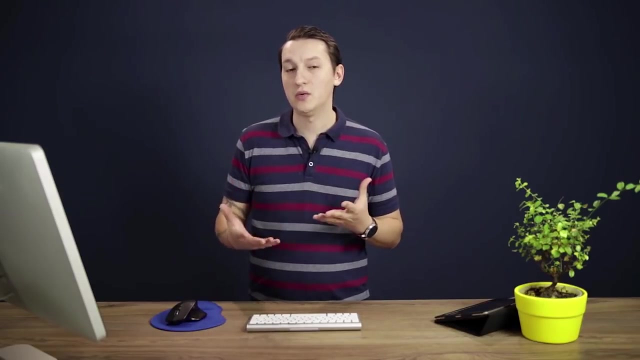 And by using these properties and methods, you can gain access to various elements in your DOM and do various things with it. Now, in this lesson, I'm going to show you some of the layers in this DOM and the more popular or well-known selectors that you'll find yourself using as a web designer. 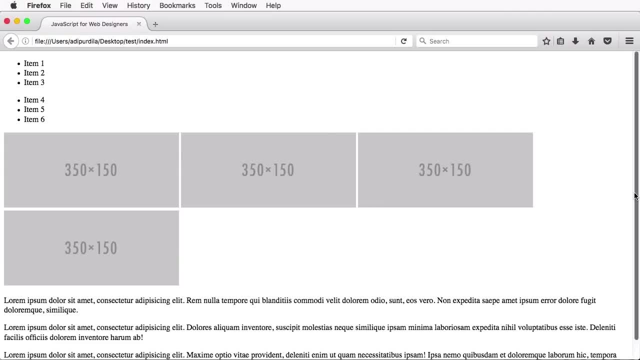 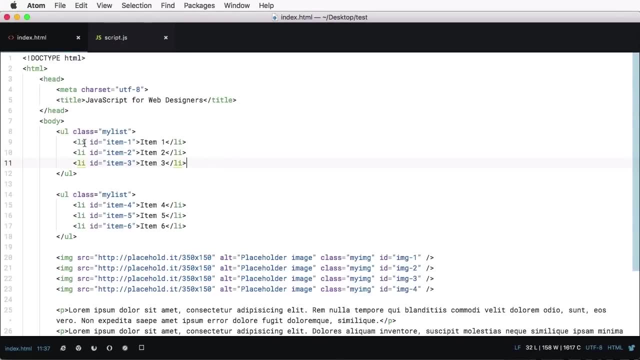 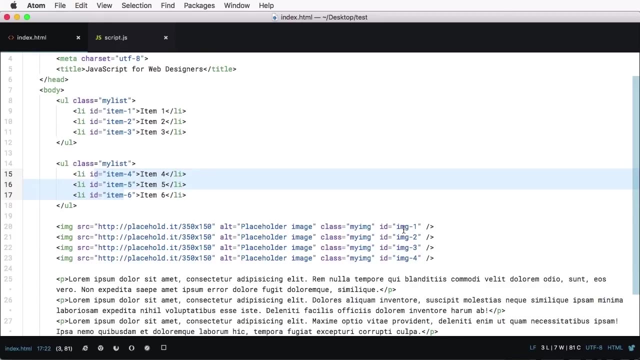 So the first thing, let's actually show you the page I have here. It's a simple demo page. We have some unordered lists, a bunch of IDs. on both of these We have four images, all with a class of myimg. 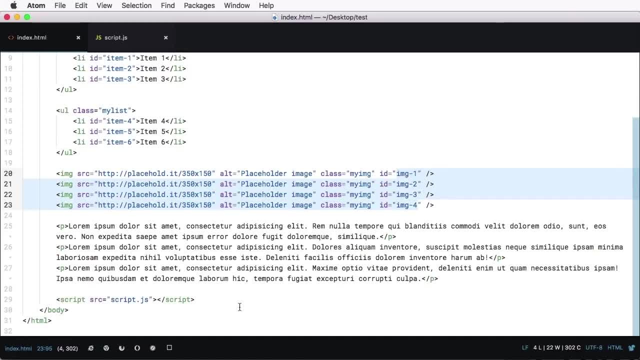 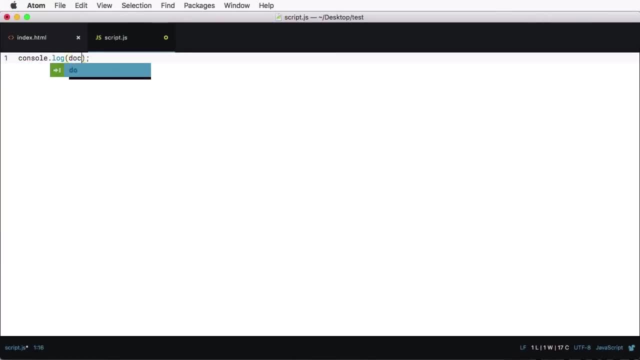 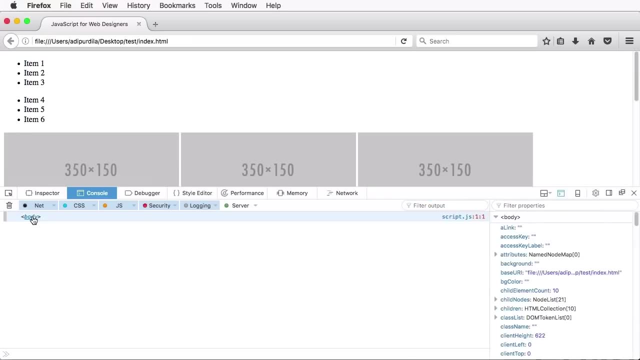 and each one with its different ID, and then a couple of paragraphs. Now let's start with this. I'm gonna do a consolelog for documentbody And let me actually open the inspector here, right, And this gives me body. 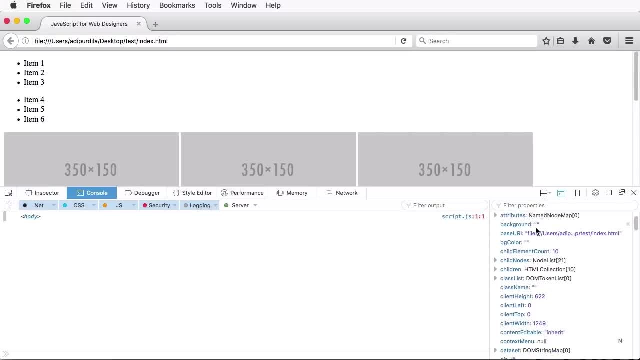 Now, body is an object and you can see all of its properties. You can get a lot of information about this, For example, client height, client width, the inner text, the inner HTML. Down here we have events. We'll learn about those in the next lesson. 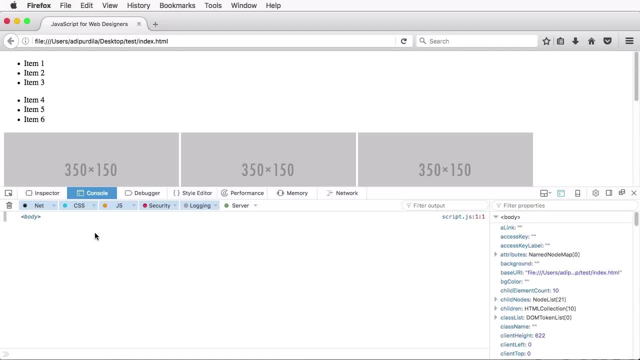 But basically this is a very simple way to access these properties, Or document images, for example. Document images is gonna give you this HTML collection right, So we have your images here And you can learn various properties for them, like the base URI. 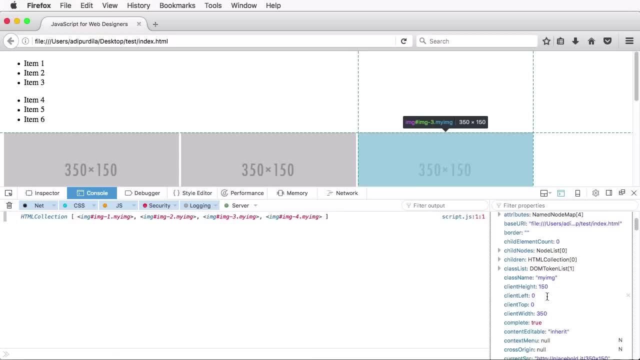 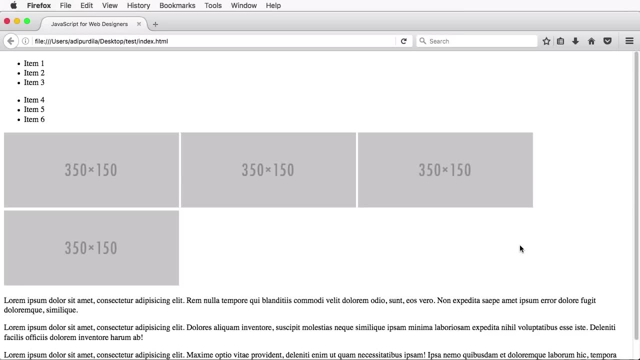 You can learn the alt, the class name, width, height, the SRC and so on. So by having access to these, you can actually start using selectors and manipulate them, do various things with them. So let's see a couple of examples. 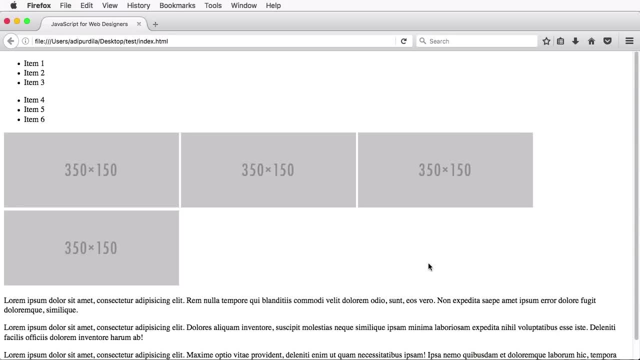 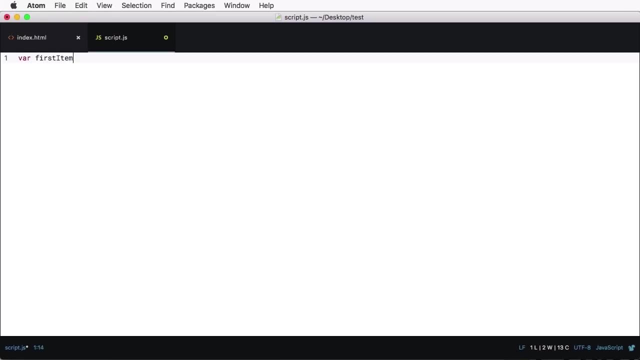 Let's say, for example, that I want to grab the very very first item, which is this item1.. How exactly would you do this? Well, we're gonna go right here and I'm gonna say this var firstItem equals, we're gonna get the document object. 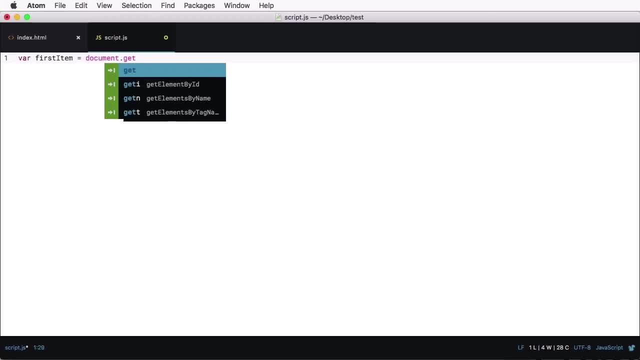 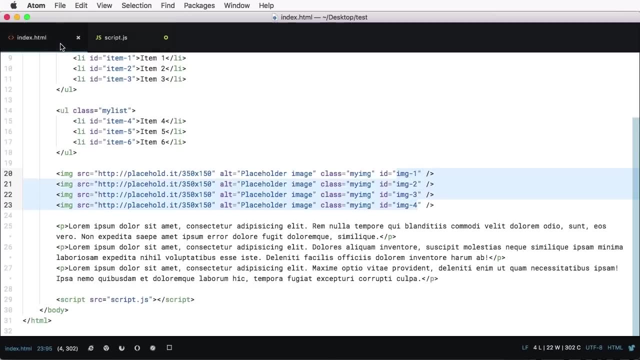 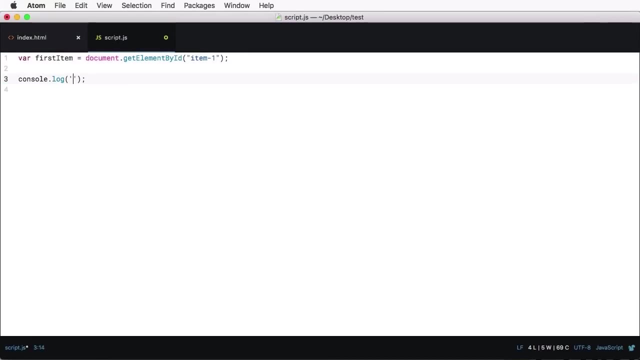 And we're gonna use the following method: getElementById, And in here we're gonna put the id of item-1, because that's what we have in the DOM, as you can see here: id item-1, right, So if we do a console log for this first item, 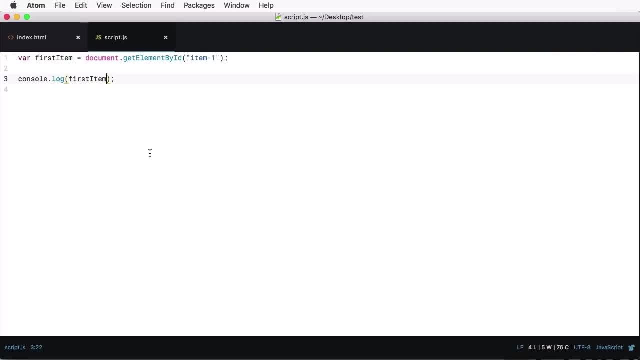 it's gonna give us the item itself, right? So that's the first method that I want you to remember: getElementById. It returns the first element that it finds in the DOM with that particular id. Now, this will just return one element. 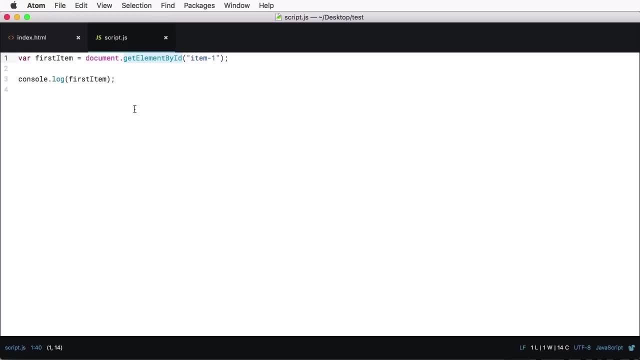 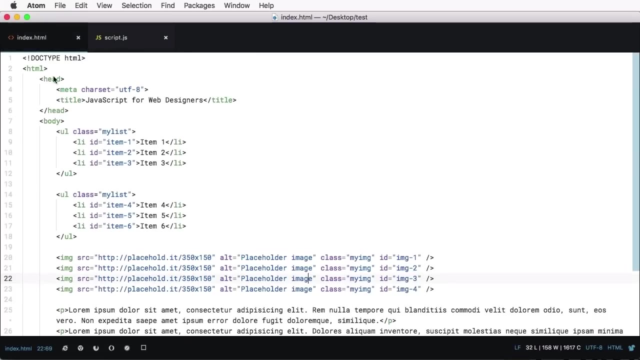 because, if you want your HTML to be valid, ids are unique, So you cannot have two elements with the same id. So that's why this method, this function, basically returns a single element. Okay, now, let's say that you want to get access to these two ULs, right? 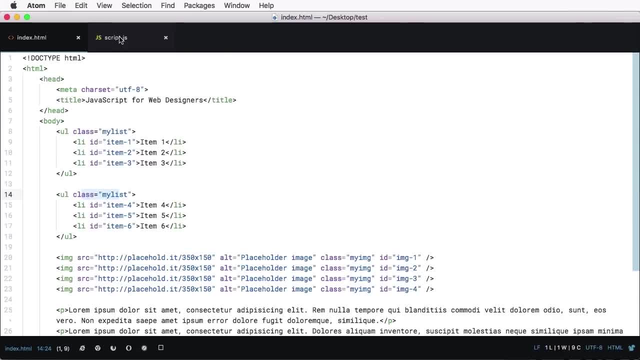 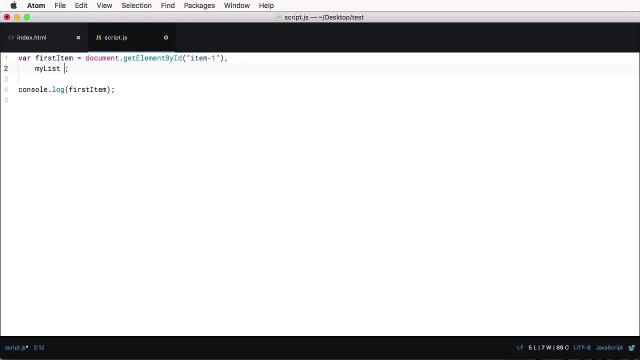 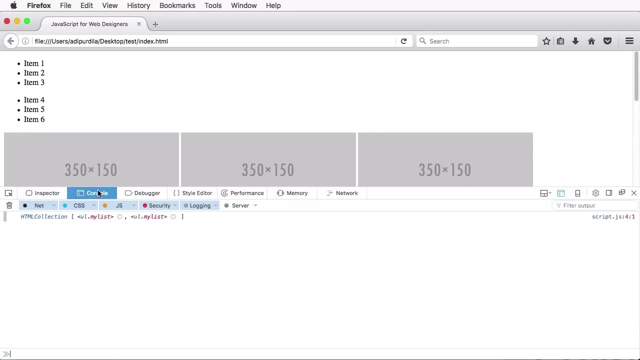 So they both have the class of myList. Well, to get elements with the same class, you would do document GetElements, plural byClassName, and we're gonna say myList, Yeah, so now myList gives me these two unordered lists. 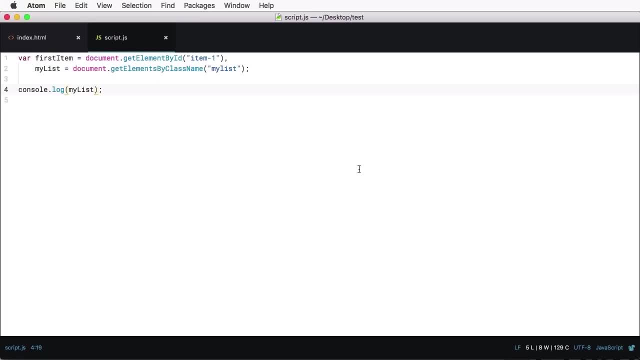 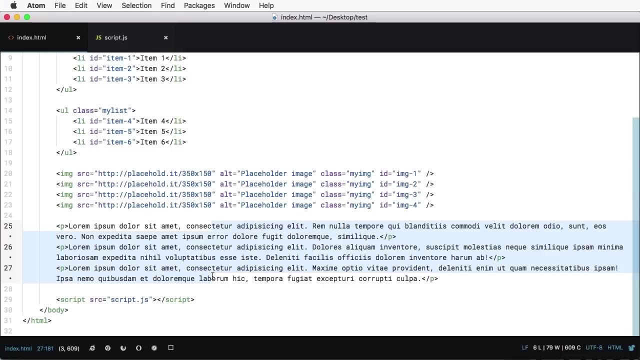 What about getting elements by their tag name, which means get all the images, all the paragraphs? Well, that's also easy to do. You can say, for example, paragraph paragraph equals document. getElements byTagName paragraph. And that's gonna select these three paragraphs here. 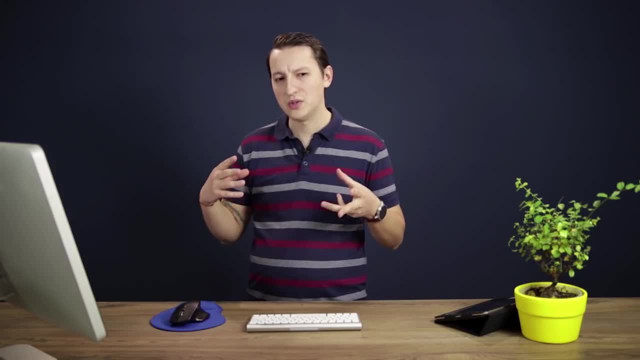 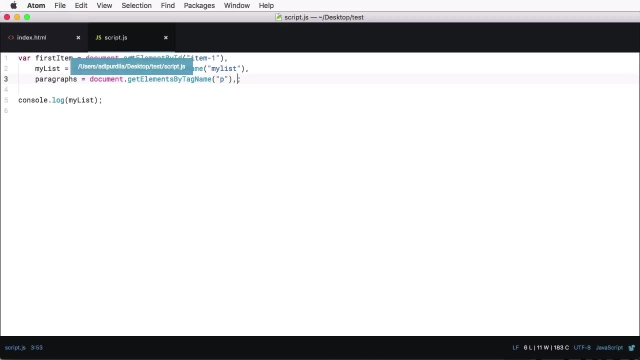 Now, if you've used jQuery, you remember how you would do selectors there. You would do something very close to CSS selectors, right? Well, you have something similar in vanilla JavaScript, and that's with a method called querySelectorAll. So, for example, let's say that I wanna select all the images. 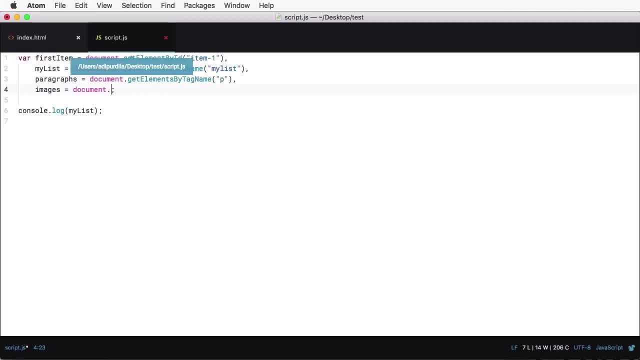 Well, I can just say: images equals documentquerySelectorAll, And I would pass in a CSS selector- in my case it's img- And that will select all the images. Okay, so now you have all of these variables which reference objects or elements in your page. 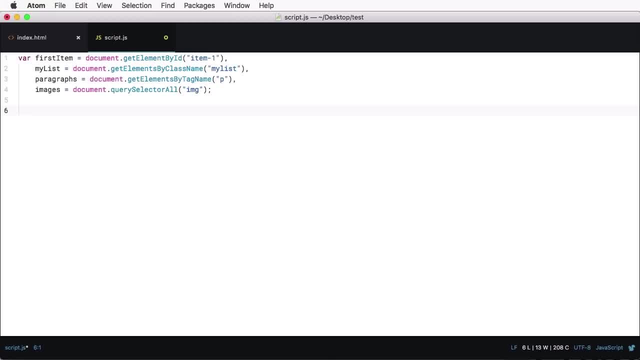 How do you manipulate them? Well, first of all, you can start with the CSS properties by using the style property. So you would say something like, for example, firstItem, You would say style and then color, And you would change that to something else, for example red. 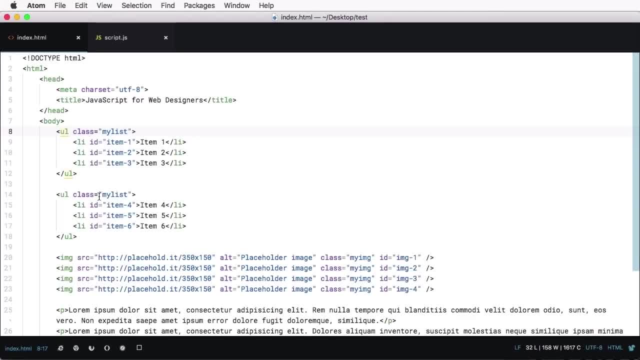 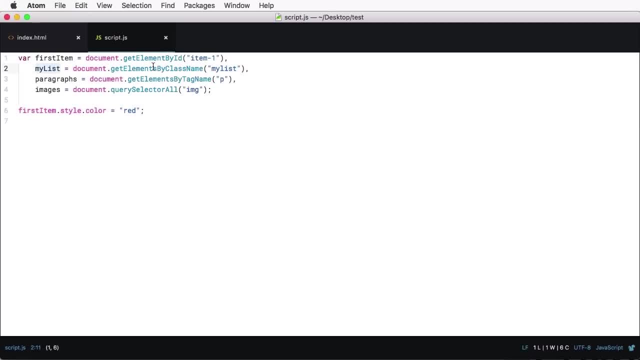 So now the first item is red, Then what if you wanna hide this second list? Well, let's think about it. MyList is actually an array. that's what getElementsByClassName returns, So it's an array. you're gonna access it like this myList. 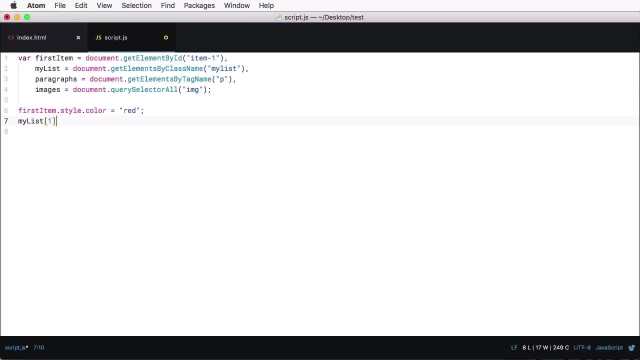 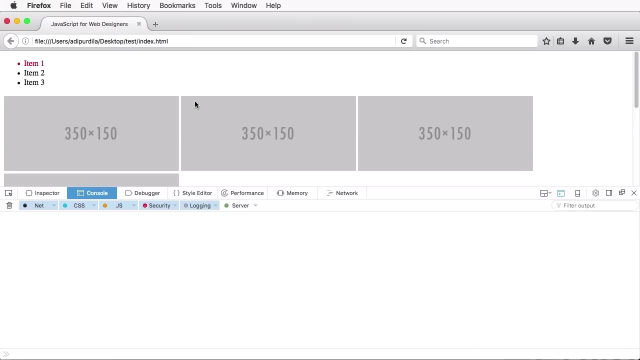 You're gonna pass in an index. I'm gonna say one, because we have two items And it's a zero-based index, so we have zero and one. So myList. one style display equals none And that will essentially hide my second list. 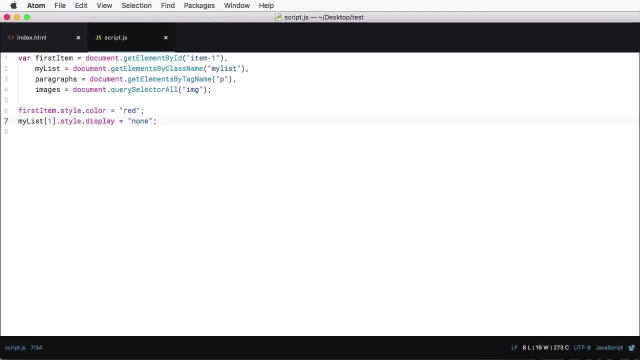 Then let's say that I wanna change the color of all of my paragraphs to green. Well, you can actually use. you can do it by hand or you can use a loop. So, for example, we're gonna say for var i equals 0,. 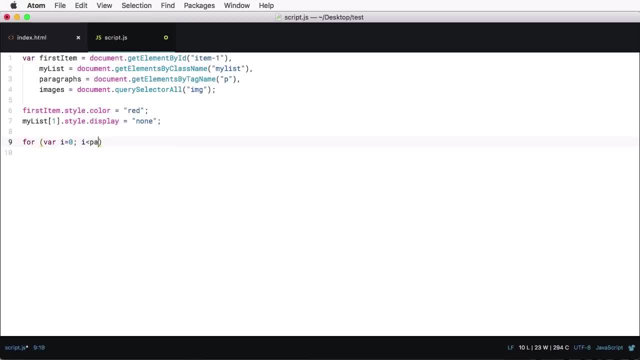 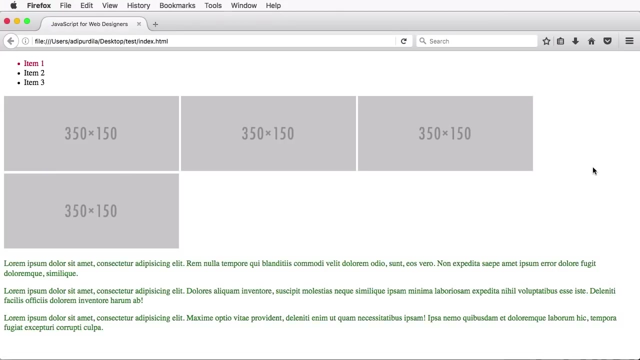 i smaller than oops, smaller than paragraphslength. Paragraphslength works here because paragraphs is an array i++ Paragraphslength. We're gonna say paragraphs i style color green, So now all of these paragraphs are green. 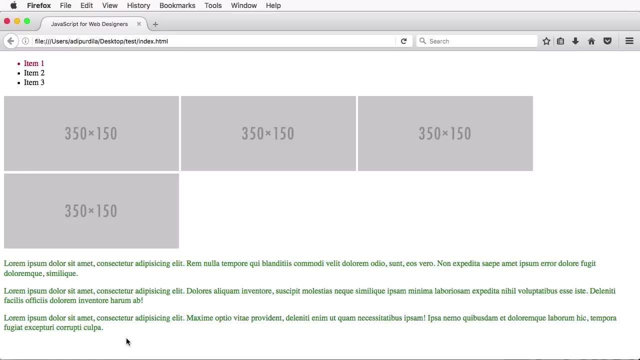 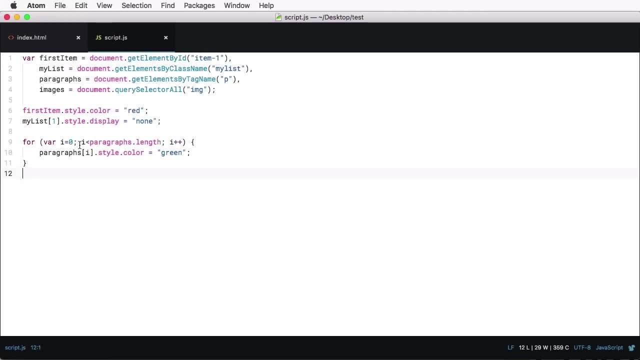 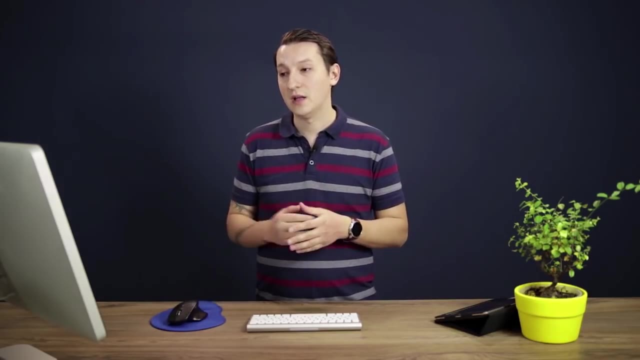 And that's how you can manipulate the DOM using selectors and a loop. Now, the list here can go on and on, but these are the basics. This is what most people use. This is what you'll mostly be using To access elements in your DOM. 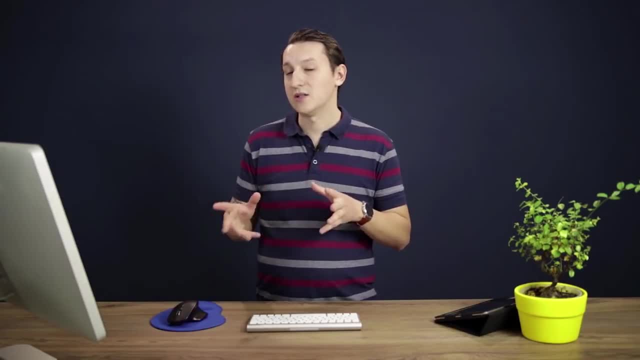 And we're gonna leave it at this. You're gonna see more complex examples when we get to the demos at the end of this course. Now, JavaScript also allows us to work with events, And that's what we'll be learning in the next lesson. 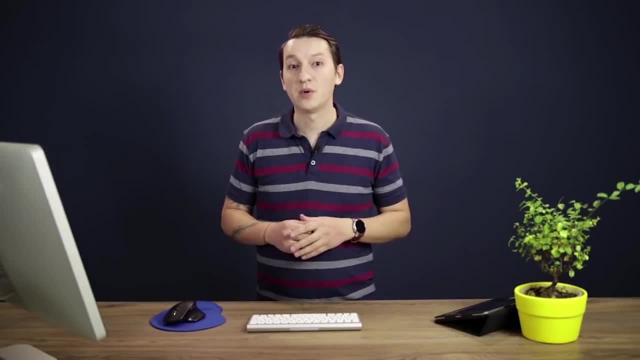 See you there. Hello and welcome to lesson number 11, where you'll learn how to use JavaScript to learn about JavaScript events- And actually JavaScript events is a bit improper, because the events are happening on the HTML side. All you can do in JavaScript is listen to these events and react accordingly. 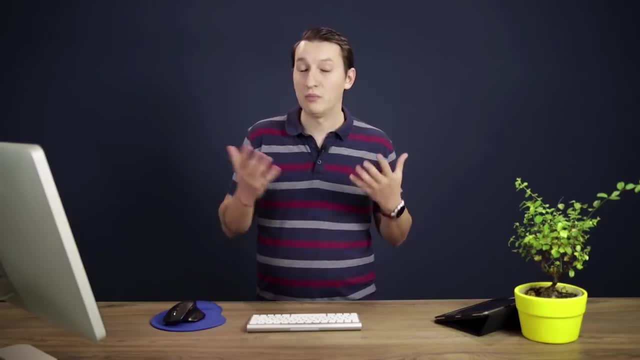 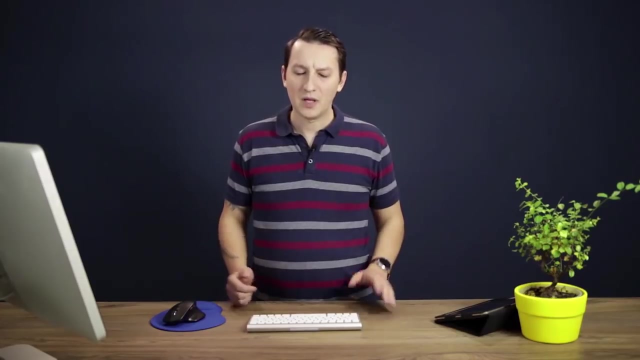 Now, an event can be something triggered either by the browser, like, for example, when the page has finished loading, the browser triggers an event, Or when an image has finished downloading from the server, then the browser triggers another event. Or they can be something triggered by the user, like for example: 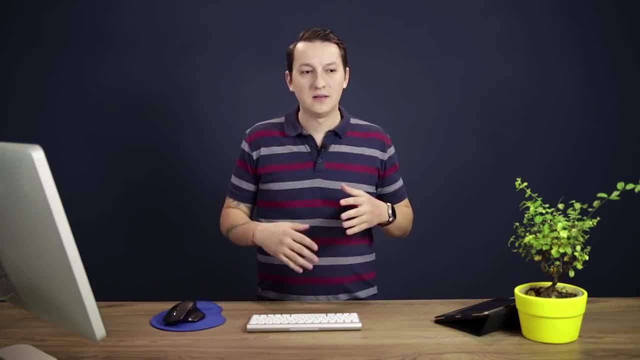 when you click a button. Now, the list of events is like a mile long And we're not gonna go through all of them. Instead, we're just gonna pick four, which are probably the ones that you're gonna be using the most. 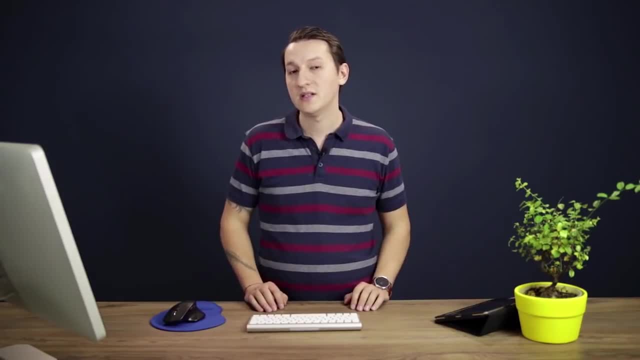 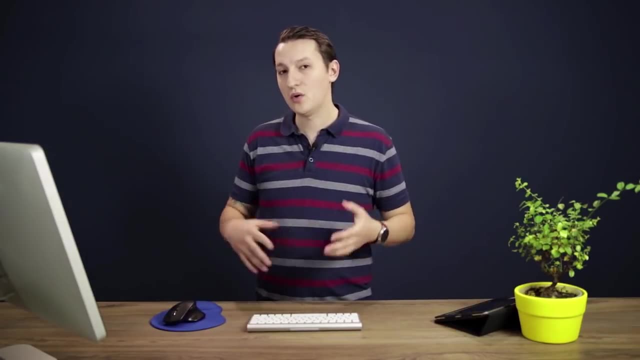 And I'm gonna show you how to listen to these events and how to react to them. And there are two ways to do this: One is in line and the other is in JavaScript. and the other things are two ways you can listen to them, either in HTML, in line. 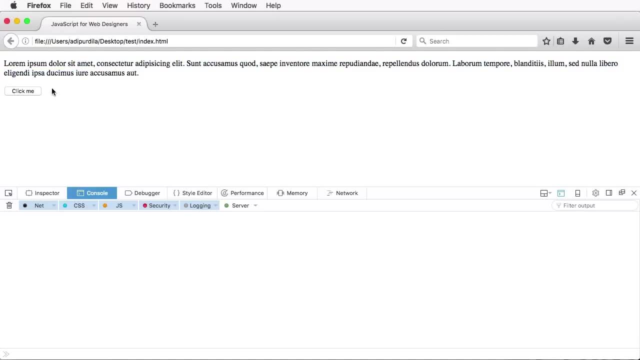 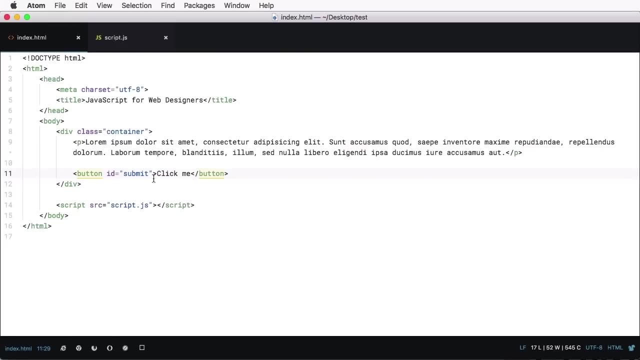 or in JavaScript with Add event listener. Now the test page I have here is very simple. We have a paragraph in a container and a button, And of course, clicking this button does nothing for now. But what you can do is say unclick and you can execute some JavaScript code. 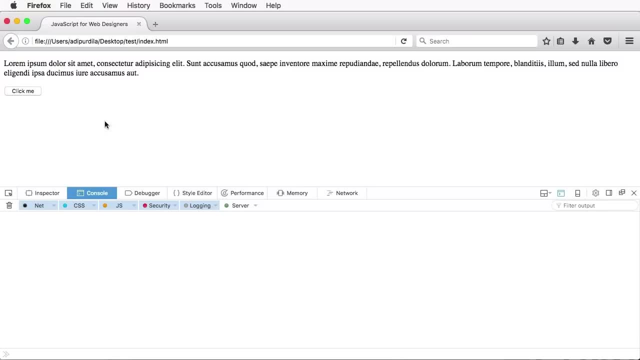 So, for example, you can say something like consolelog: button clicked. So now, let's do that. So now, when I click the button, I get a console log. So that was a piece of JavaScript that you just executed. This is the simplest way to tie into an event like click, for example. 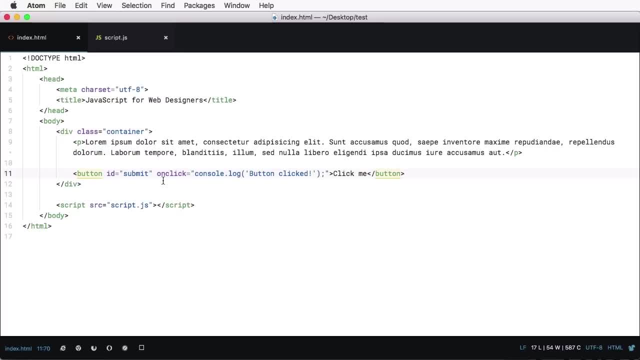 There are other events, for example like onLoad, onMouseOver, onKeyUp. These are just a few examples. Now let me show you how to listen to these events from JavaScript or using JavaScript code. So in my scripts file here I'm gonna declare some variables. first, 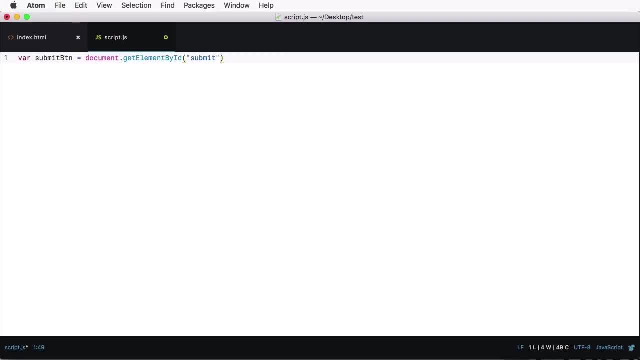 Submit btn. it's gonna be document: getLnById submit And then I'm gonna target the container: equals document. I'm just gonna say querySelectorContainer. Now I'm gonna get the submit button and I'm gonna use the function addEventList. 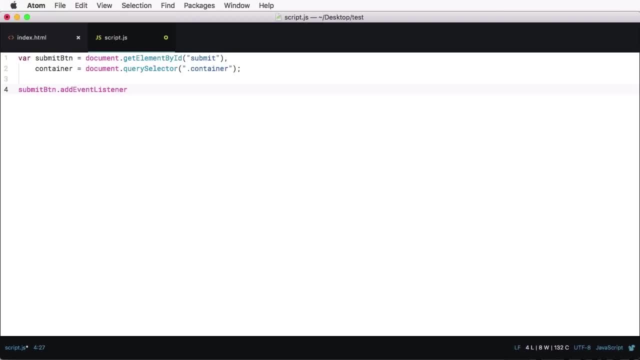 It looks like this: addEventListener: We're gonna pass in the name of the event that we want to listen to. In our case it's click, And then we're gonna specify what happens when that event is being triggered. We can pass in a function name or we can declare an anonymous function here. 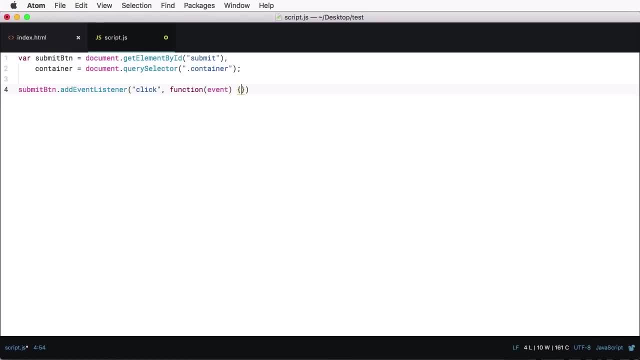 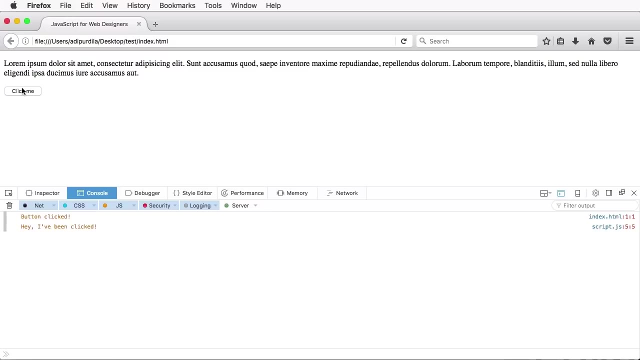 So we're gonna say function, we're gonna pass in the event parameter, And then we're gonna say consolelog: Okay, I've been clicked, I'm just gonna escape this character right there. Okay, so now, if I click this, we get two different console logs. 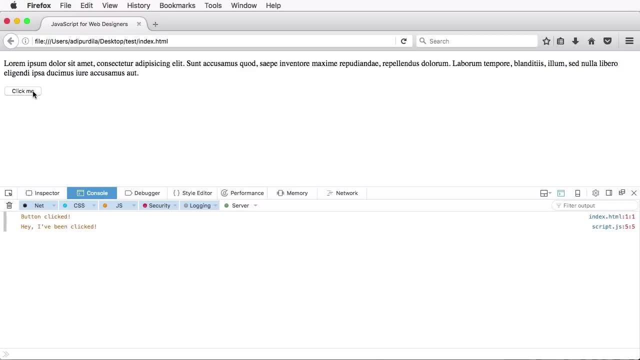 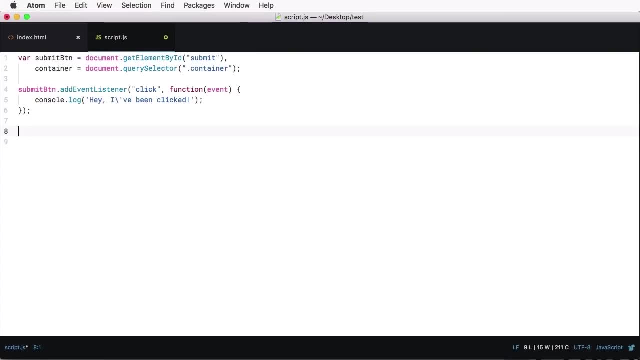 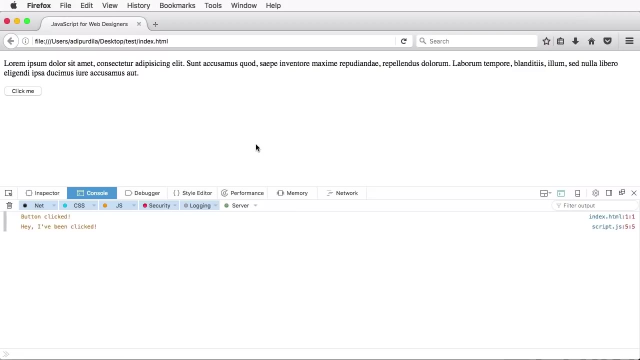 One is from the onClick in the HTML and the second one is from the addEventListener from JavaScript. Now let's see an example of another event, for example, mouseEnter. And let's say that when I enter with my mouse cursor in the container area I want to do something, do a console log, anything? 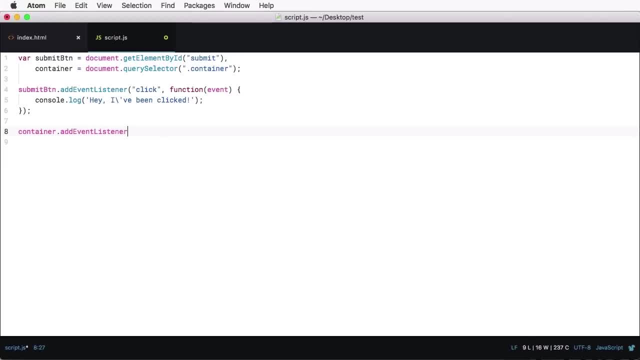 So I'm gonna say container addEventListener. We're gonna pass in the event name- in our case it's mouseEnter- and the function name or the function that we wanna execute. In my case I'm gonna say mouseEnter container. 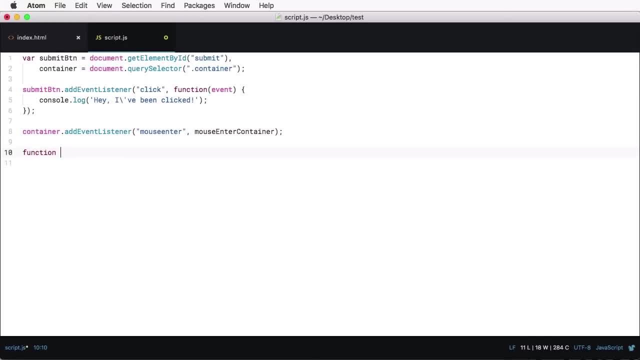 Now, this is a function that I'm gonna create right now. So function name: In mouseEntercontainer. it does not receive any parameters, But instead it does a console log that says: hey, there was a mouseEnter event triggered. 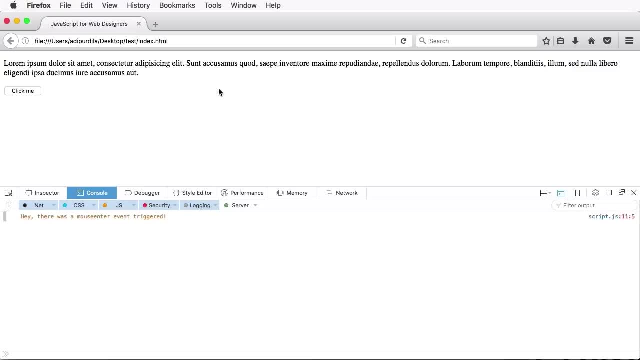 So now, whenever I take my cursor and I enter the boundaries of my container element, I get that console log. you can see by the number. here We already have ten logs, But let's say that I want to do this just once, right? 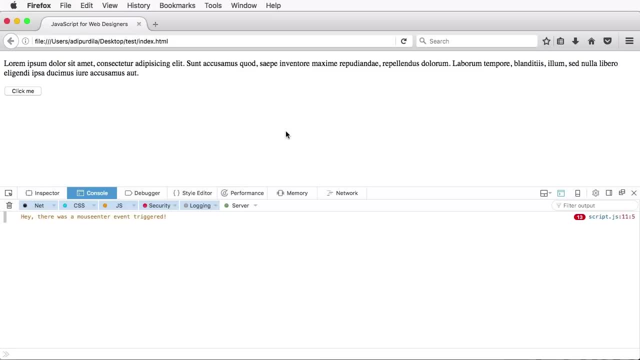 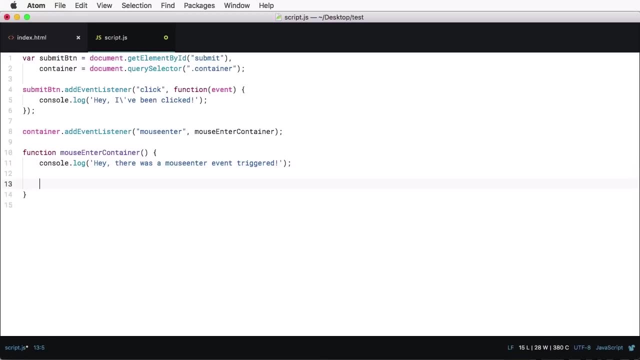 So do the console log just the first time the event is triggered. Well, to do that, I can simply do the console log and then remove the event listener. So I can say: container remove, event listener, mouse enter and then the name of the function. 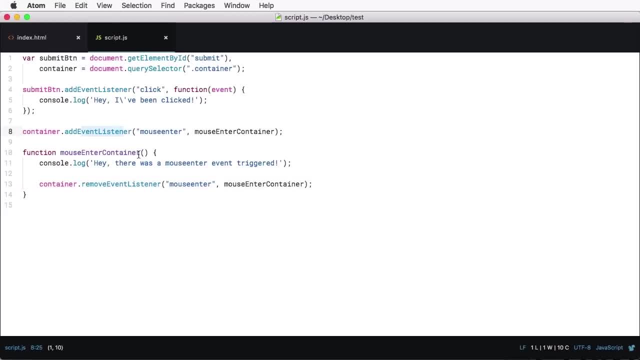 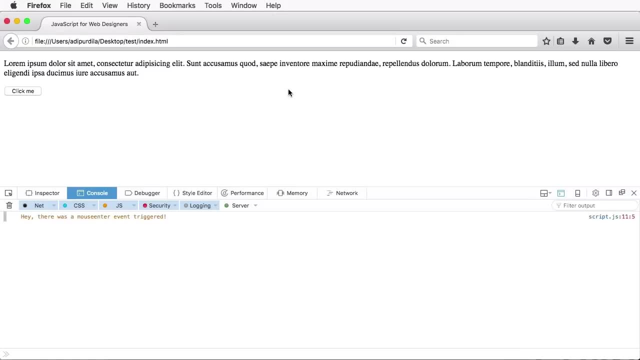 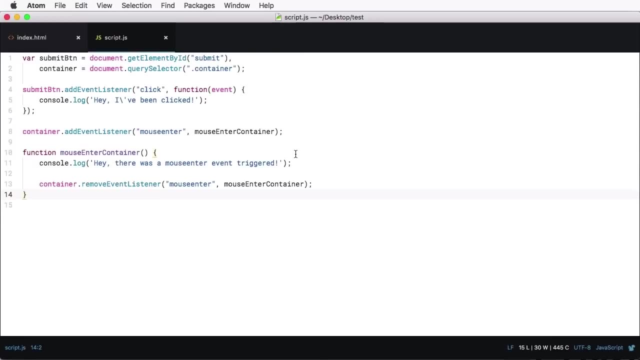 So the syntax is exactly the same as addEventListener, but we change the name of the function here. So now I enter the boundaries of the container, I get the console log, but I only get it once. All right, let me show you another example real quick for the event key up right. 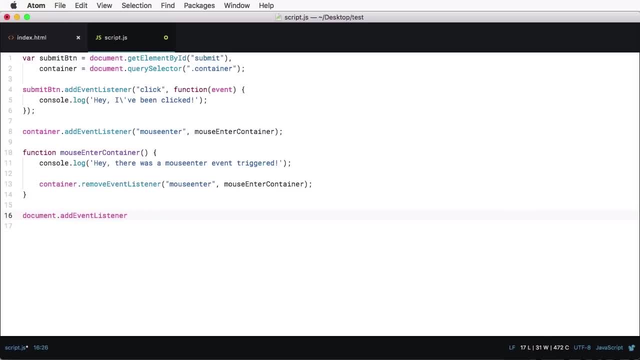 So we're gonna say: document addEventListener- key up function event. Now this is a function that's called function. This is a great way to show you what that event is doing. I'm gonna do a console log event key code. Now, event is an object that's being transmitted to this function. 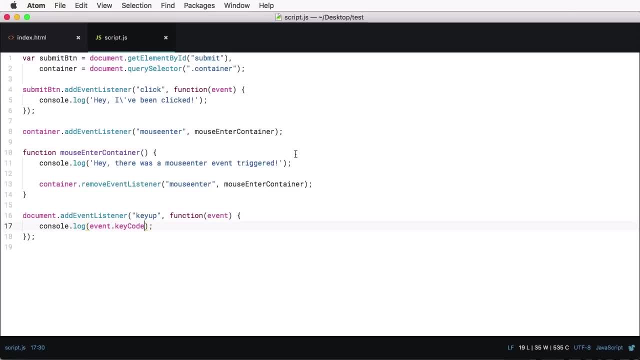 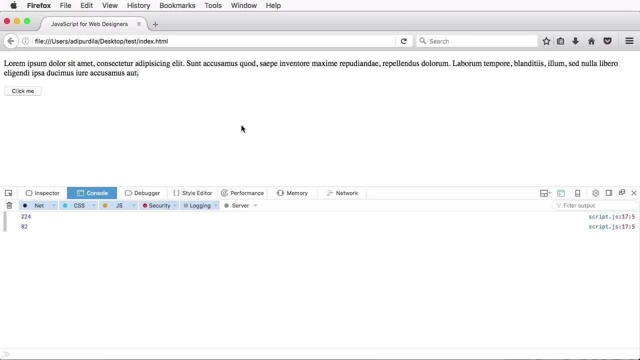 And you can access various properties for that object, such as key code, which is the code of the key you just pressed. So, for example, if I start typing, you'll see that we get various codes. If I do an enter, we get the code 13.. 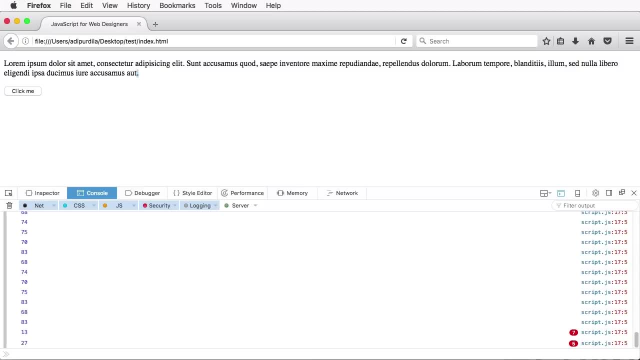 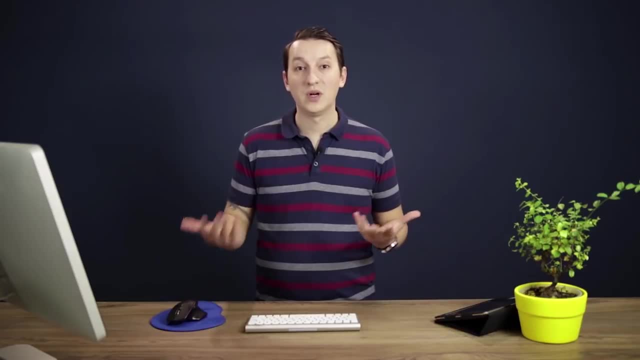 If I do escape, I get 27.. So this is a really great way to listen for key presses. To give you an example of what you'll be using this for, or what you could be using it for: you make a slider, an image slider. 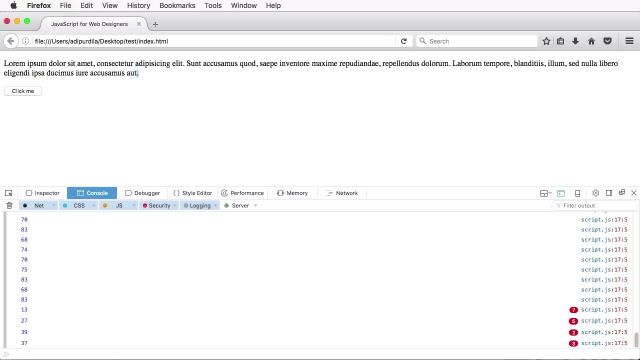 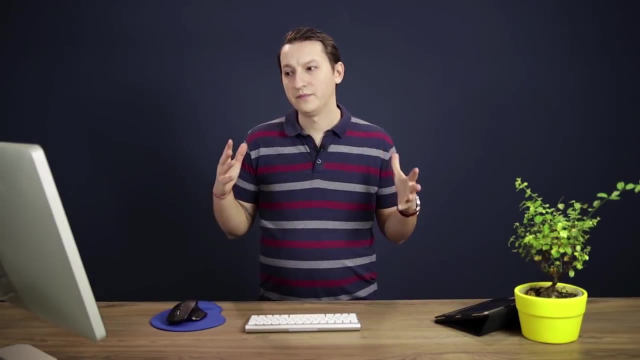 And you would use the right and left arrow keys. You can see their codes pop up just right there: 39,, 37, to switch slides right, To move, To move between slides. So that's one use for them. But yeah, basically that's about it for JavaScript events. 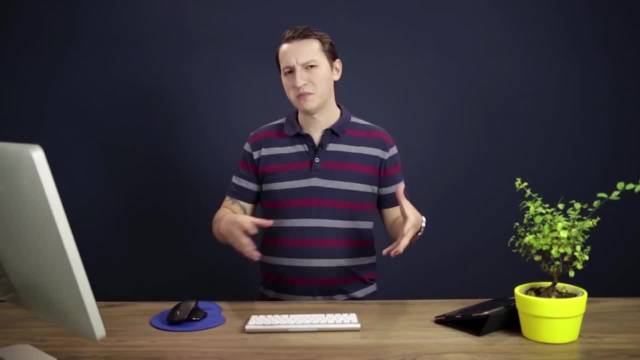 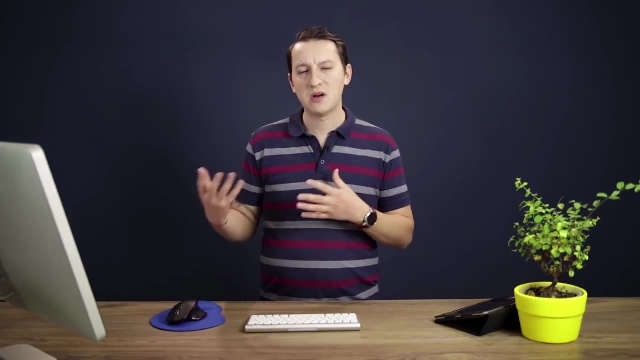 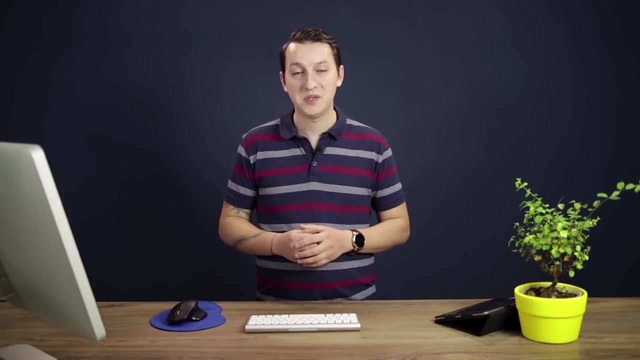 Now you've learned the basics of JavaScript, So it's time to put this knowledge to good use by creating some demos for some of the most common coding patterns in JavaScript, And we'll begin in the next lesson with a back to top. See you there. 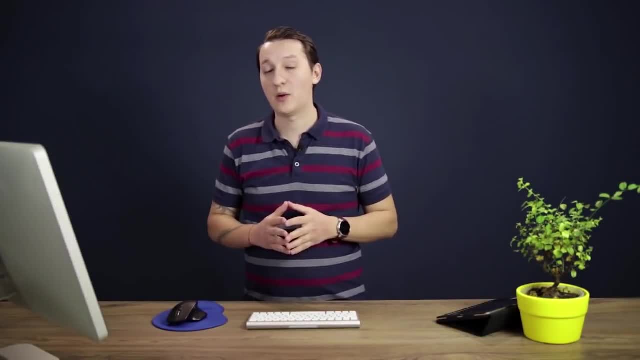 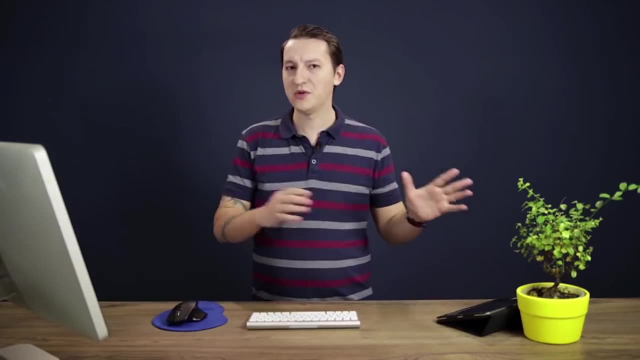 Hi, welcome to lesson number 12.. This is the first of our five demos, And in this lesson we're going to create a back to top button. Now, I'm sure you've seen this around. it's a very common pattern. 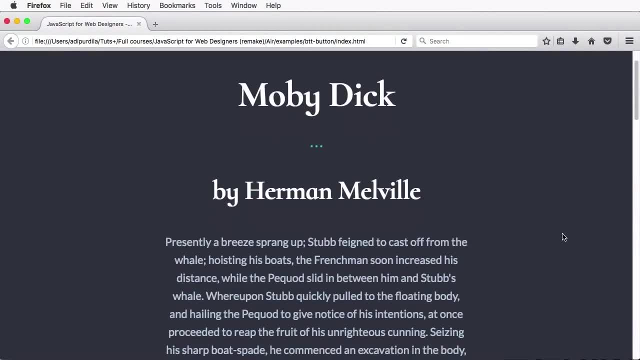 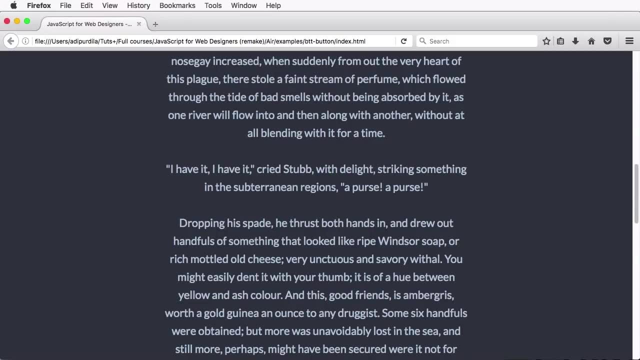 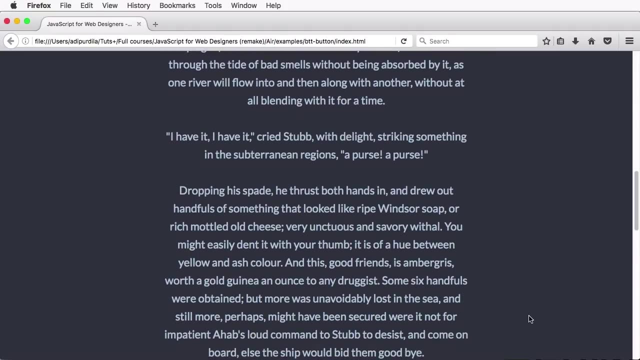 And the way this works. basically, you have a web page And when you scroll past a certain point you'll get a little back to top button somewhere on the page. Usually it's on the bottom part of the page And when you click it you're taken back up to the top of the page. 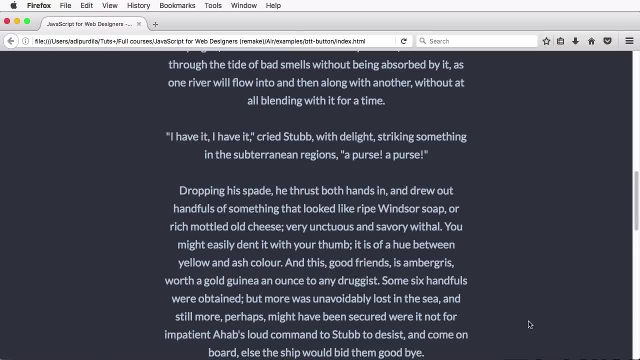 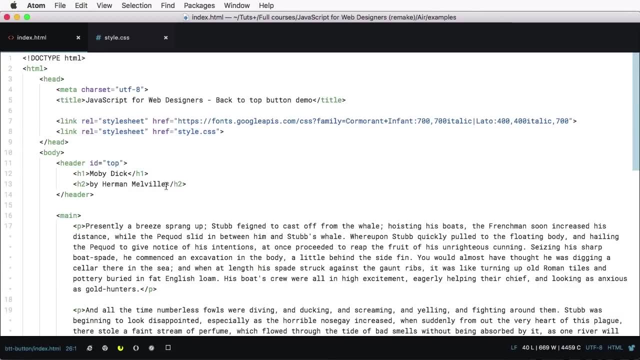 So let's go ahead and see how we can create something like that using Pure or Vanilla JavaScript, if you want. Now, taking a look at the markup: here we have a header with an ID of top. We're gonna use this ID to tell our script where we need to go back to. 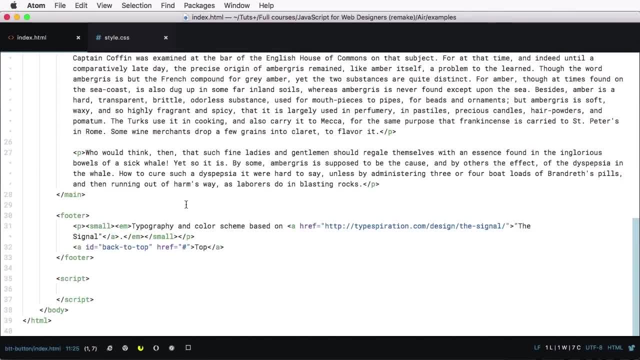 Then we have our main content. We have our main content with a bunch of paragraphs and finally a footer, And in the footer we have an anchor tag with an ID of back to top. This is our button. As far as styling is concerned, we just have some generic demo style here. 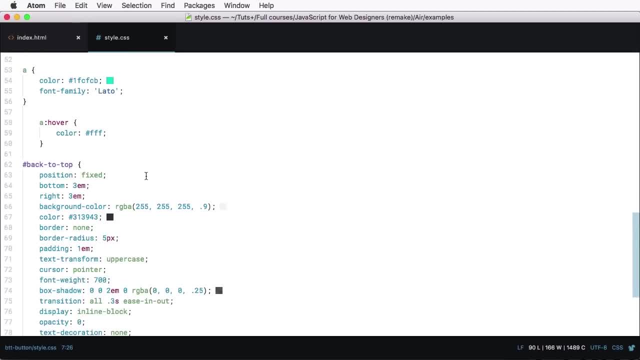 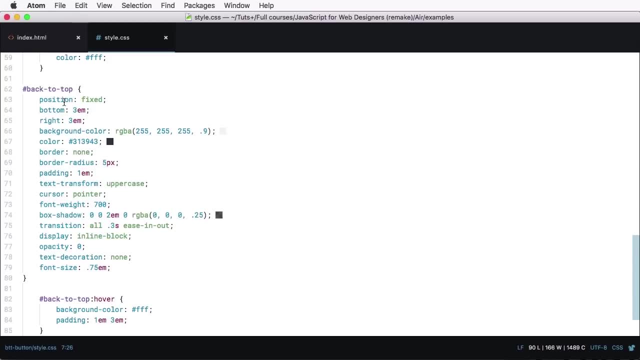 Nothing fancy really, But what we're interested in is this: back to top button right. So its position is fixed. So no matter where we scroll, it stays in the same position. It's in the bottom right corner, three M's from each side. 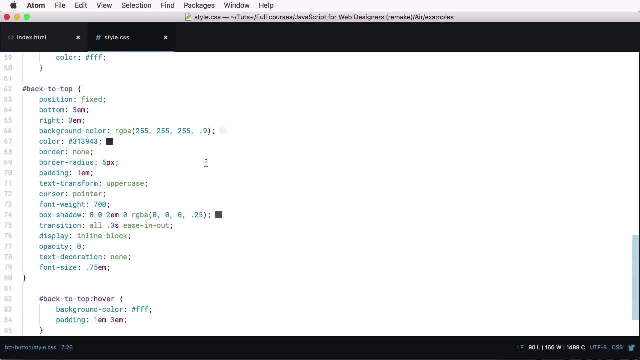 It's white with a 0.9 in the alpha channel. It's set to inline block. Currently it has an opacity of zero, so we cannot see it, And we also have a class visible which gives it an opacity one. 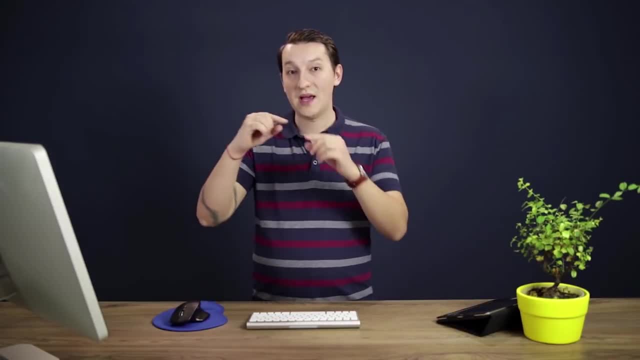 So what we need to do basically is, when we scroll past a certain point in our page, we're gonna add that class to the button making it visible, And we also have to listen to the click event on the button and make our page scroll all the way back to the top. 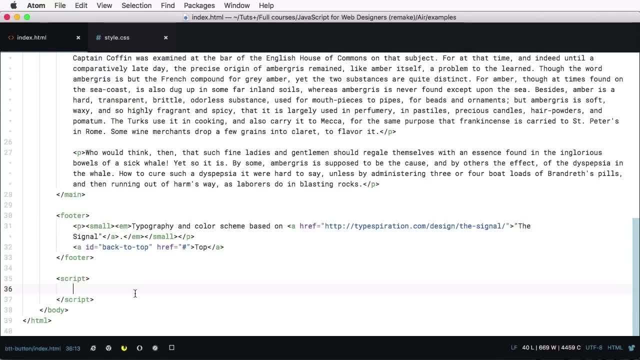 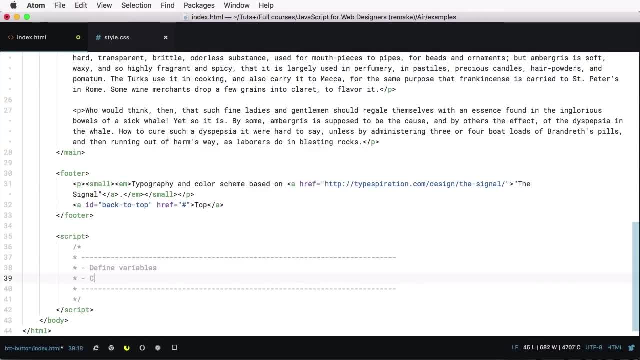 Now I'm gonna write this script right here on the bottom of the page And I'm gonna start by defining some variables, And then what we're gonna do is calculate the document height and we're gonna say: we're gonna set the offset to a quarter of that value. 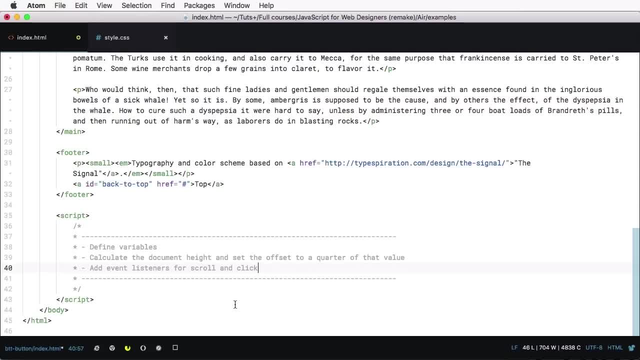 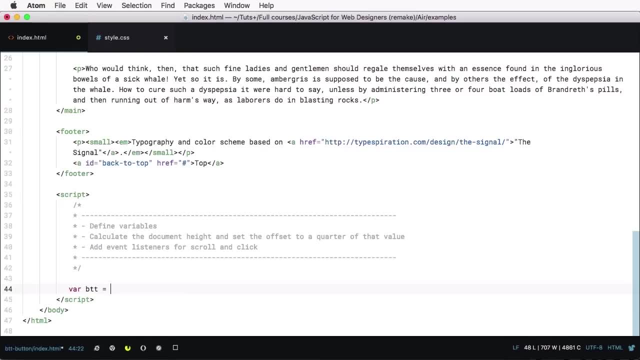 And finally we're gonna add EventListeners for scroll and click Right now for variables. we're gonna target the button, So btt back to top. We're gonna say document getElementById back to top. Then we're gonna get the body to document body. 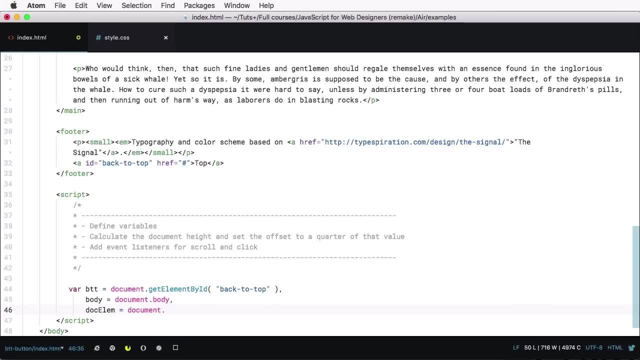 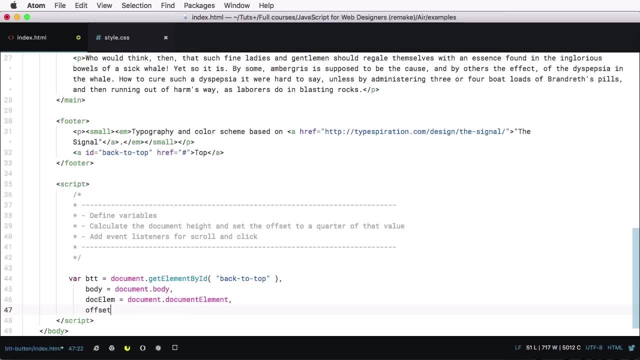 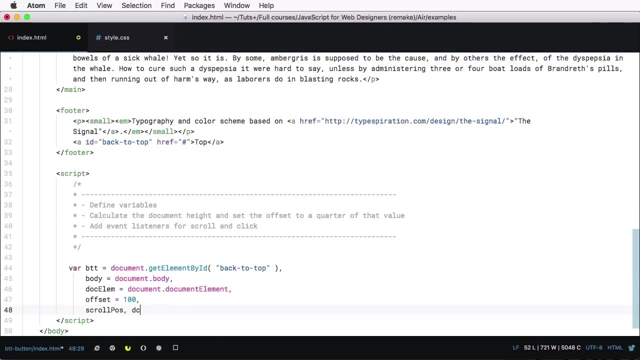 DocElem- that's gonna be document DocumentElement. we'll be needing this when we calculate the height of our page. Then we're gonna set the offset to 100,, for example, And two more variables we'll declare scrollPosition and docHeight. 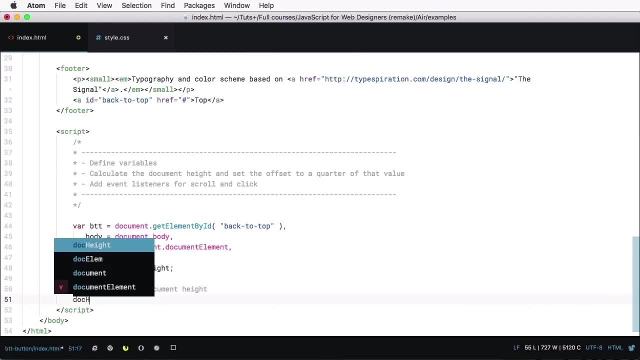 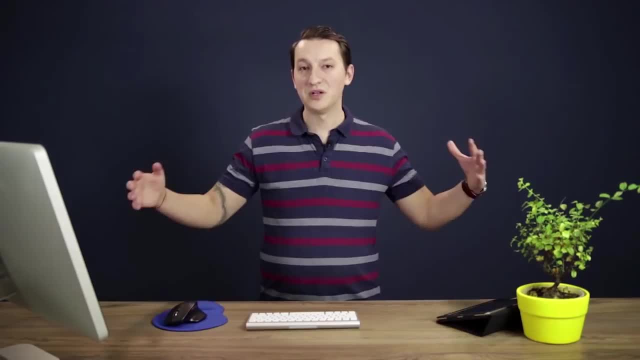 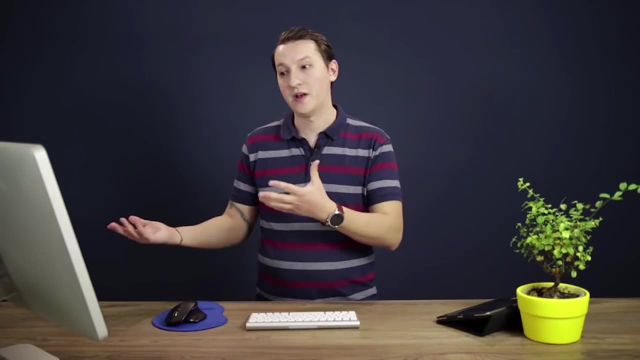 Now let's calculate the document height. We're gonna say docHeight equals Mathmax. Basically, Mathmax will take a bunch of values and it's gonna return the value of the document, The biggest one, the maximum of those values. And the reason we're doing this is because different browsers will 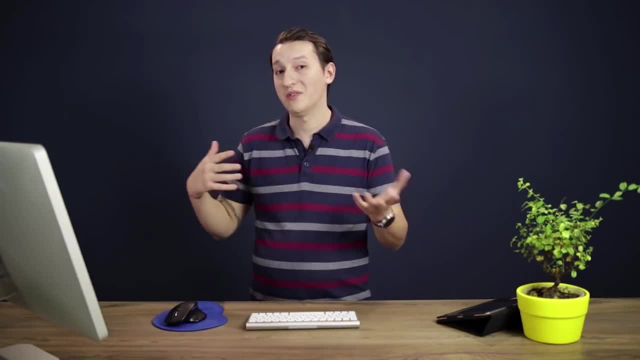 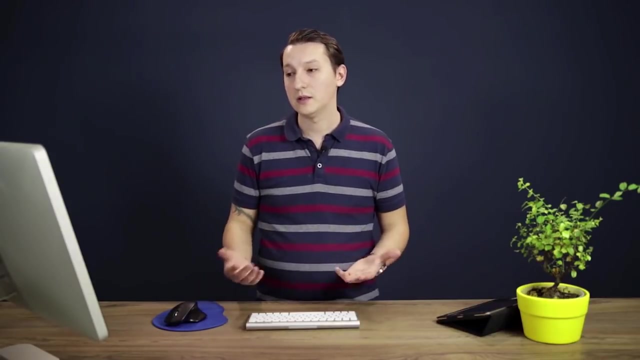 look at a document height differently. So, for example, Firefox is gonna have a different syntax to get the document height, WebKit is gonna have another one. So just to make sure we cover as many browsers as we need, we're doing this Mathmax. 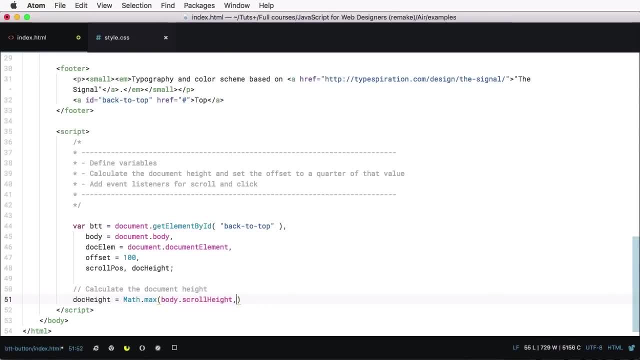 And we're gonna have a little bit of time to do that, And we're gonna have a little bit of time to do that, And we're gonna have a little bit of time to do that. So we're gonna pass in the following values: bodyscrollHeight. 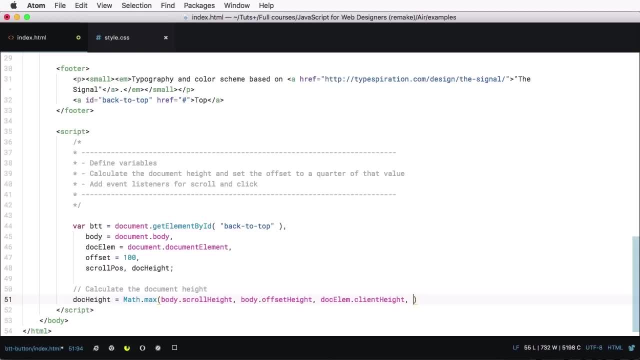 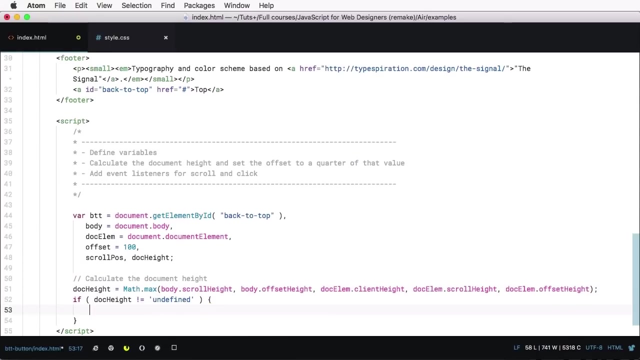 bodyoffsetHeight, docLmClientHeight and scrollHeight And finally we're gonna get the offsetHeight. Now we'll do a quick check: if documentHeight is different than undefined- which means if Mathmax actually returned something, which means if we actually have a height value- then we're gonna say: 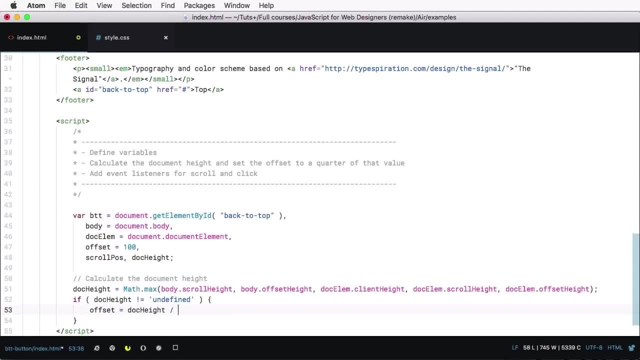 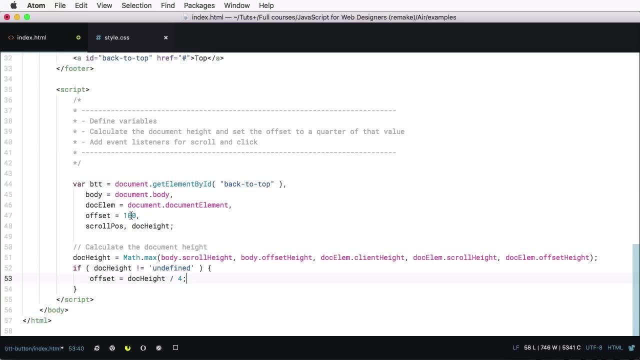 we're gonna set the offset to docHeight divided by 4.. This value- 100, is just a fallback, right In case docHeight actually turns out undefined for some reason, then we do have something to fall back on. Next up, we're gonna add the scrollEventListener. 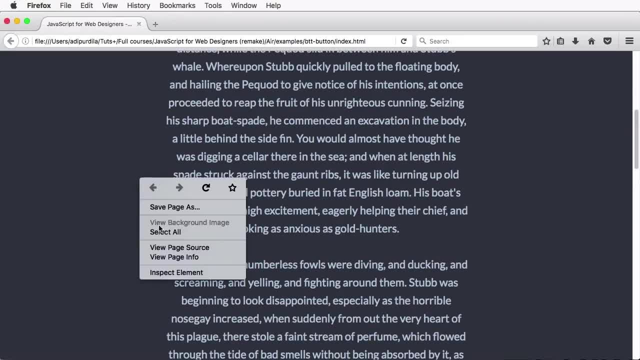 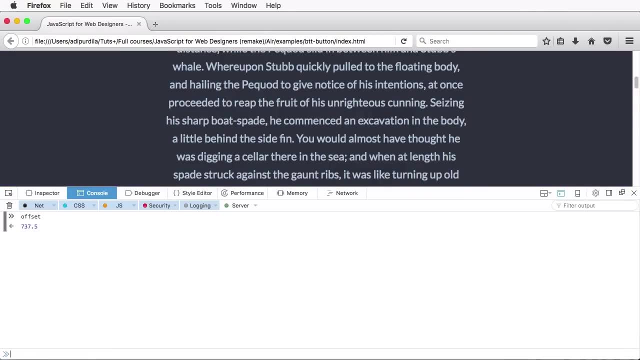 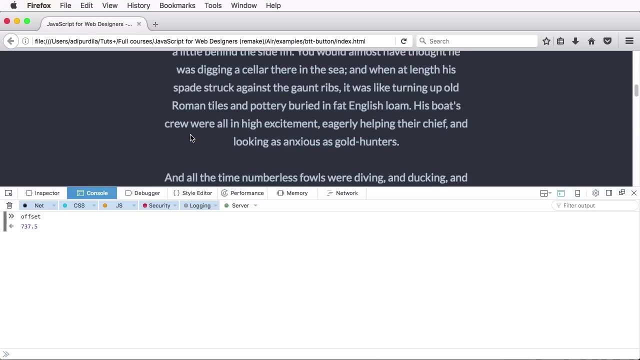 And actually, before that, let's go ahead and do a quick refresh here And go to our console and call the offset And, as you can see, the offset is 737.5.. Now, which means our script will be executed after we scroll past 737.5.. 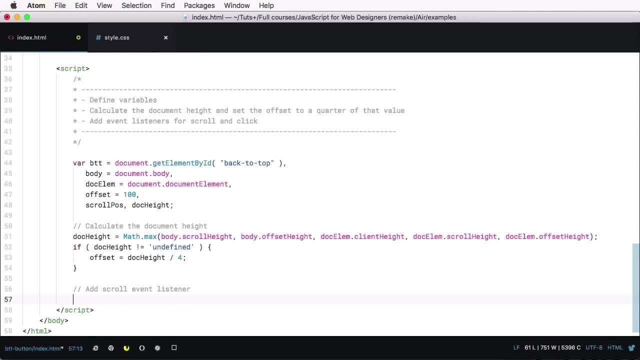 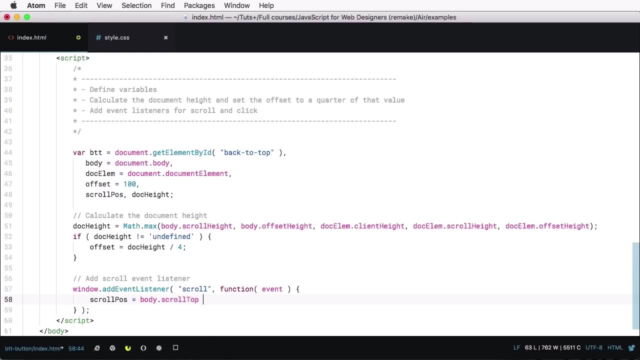 Now for the scrollEventListener. we're gonna do window addEventListener. Now we're gonna listen for scroll and we're gonna have a function. We're gonna get the scrollPosition equals to bodyscrollTop or, in case that's not valid, docLmscrollTop. 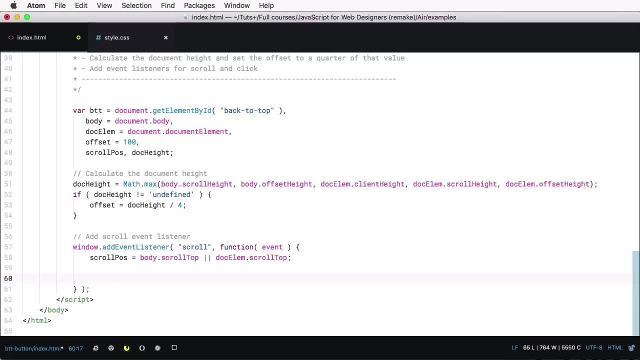 Again, this is for various browsers. And then we're gonna say btt className equals to: If the scrollPosition is higher than the offset, then we're gonna add the class of visible- Oops, sorry, the other way around, Otherwise we're gonna add nothing. 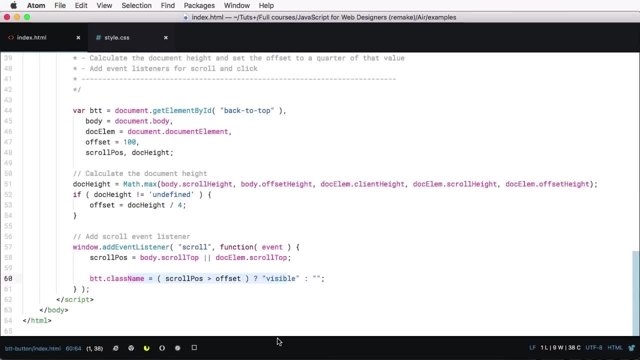 So that's what we're doing here. basically, This is the ternary operator, if you remember, or the conditional operator. We're checking if the scrollPosition is higher than the offset. So basically, if we passed that threshold when we scrolled, 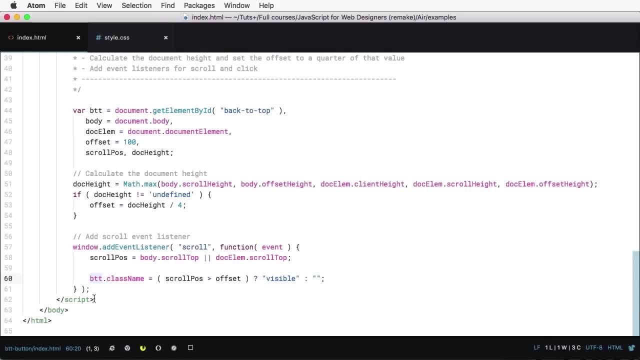 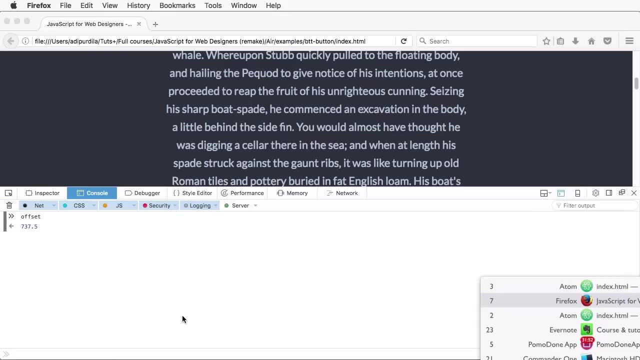 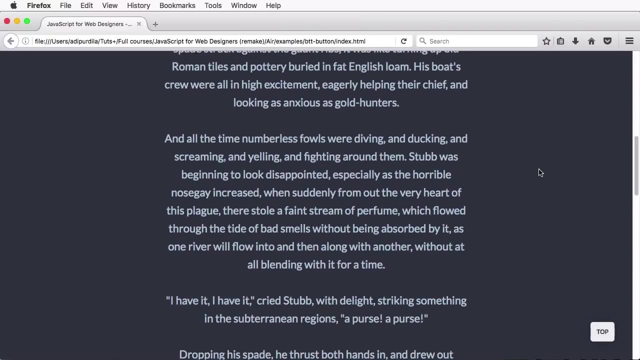 we add the class of visible to the button, to the btt. Otherwise we add nothing to the class name. Okay, so let's have a quick look, Refresh and let's see there it is. So when we scroll, yeah, past that point, we make the button visible. 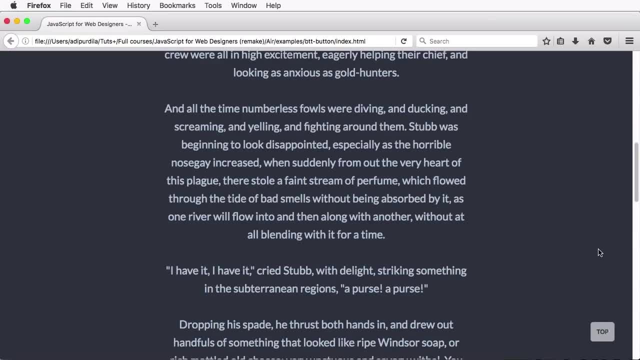 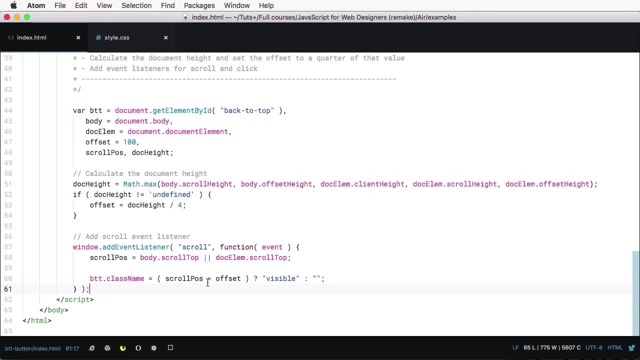 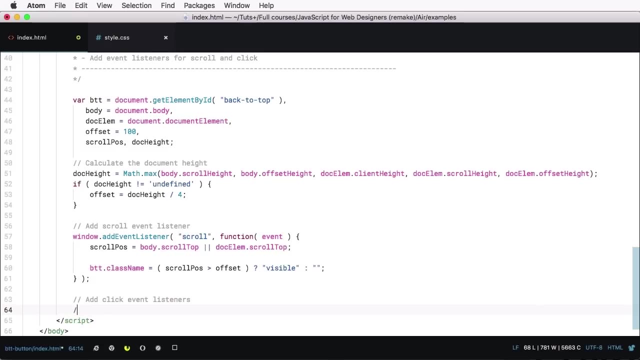 And when we go back up we're hiding it. Okay, now let's actually make this button work. So when we click it, we want it to go to the very top. So we're gonna say: addClickEventListener btt. addEventListener click again. function event. 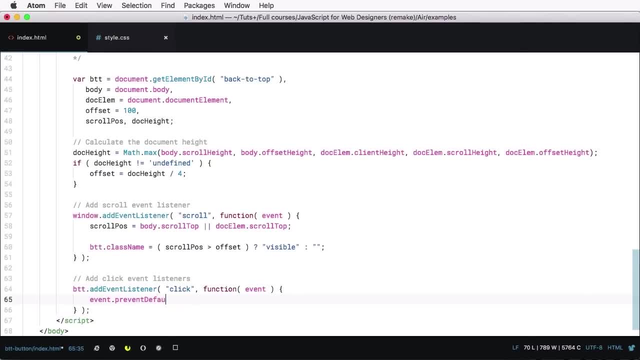 First thing we'll do is say event preventDefault, and that's to make sure that the function is there. Okay, The button- or in our case it's an anchor tag- it doesn't go anywhere. That's what this function is doing. 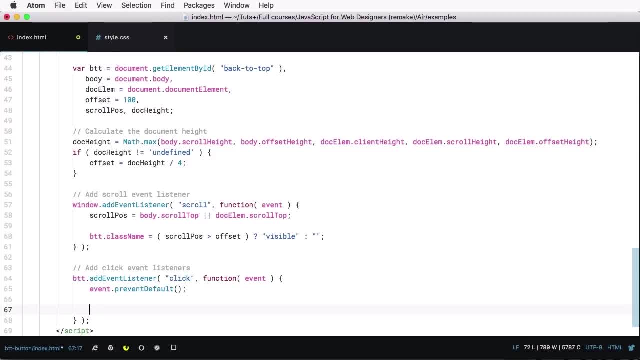 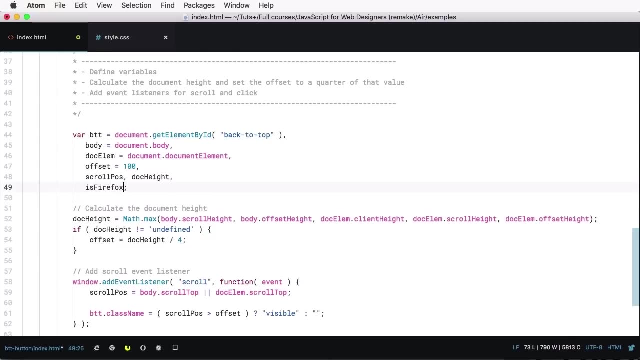 And then we're going to check: if our browser is Firefox, then we need to set the scroll top value in a different way. So what are we gonna do here is define another variable called isFirefox And isFirefox. actually, this is very, very easy to do. 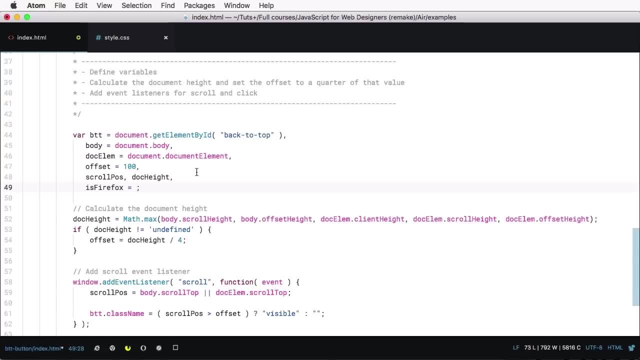 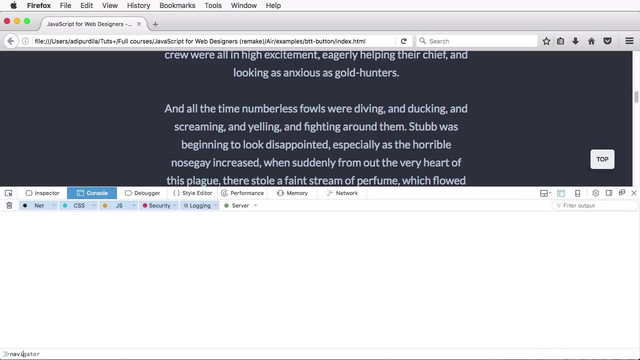 We're gonna check for the NavigatorUserAgent. So let me, actually I'm gonna say true here, just so we have valid code, But I wanna open the inspector here And what I'm gonna do is say NavigatorUserAgent, And NavigatorUserAgent is gonna give us this bit. yeah, 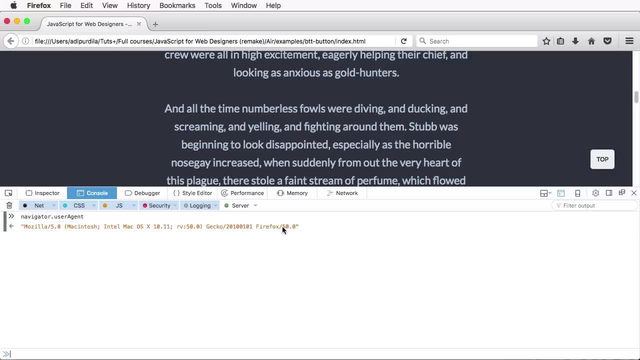 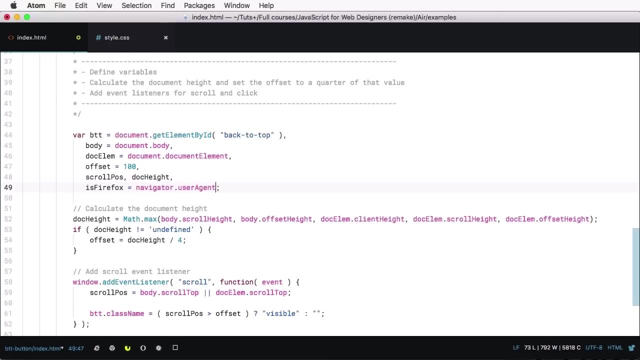 And an easy way to check if this is Firefox. well, it says Firefox Right here, So all we gotta do is compare that string to the word Firefox. So isFirefox will be equal to the following NavigatorUserAgent dot. we're gonna use a method called toLowerCase. 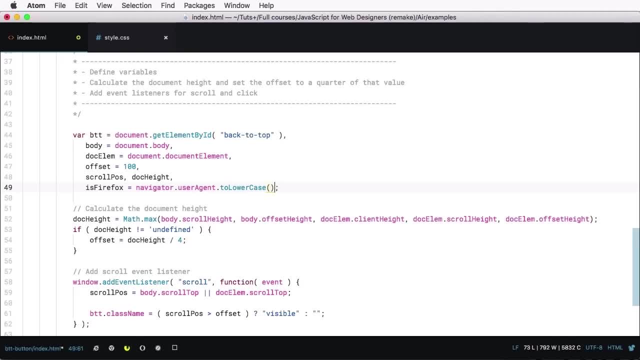 which will take a string. it's gonna make it lowercase, And then I'm gonna say IndexOfFirefox is higher than minus one, Okay. And then I'm gonna say IndexOfFirefox is higher than minus one, All right. so if you don't understand what happened here, let me tell you. 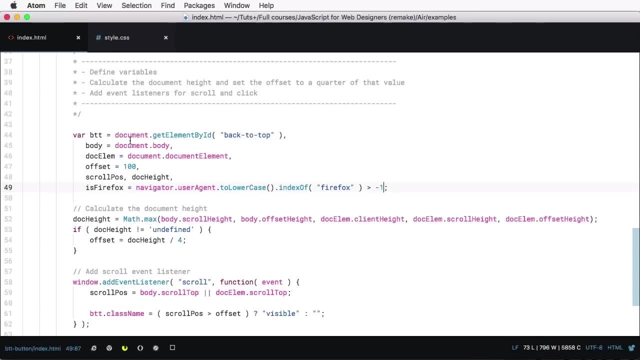 Navigator user agent will give us that string you saw in the console. Two lower case is gonna make everything lower case. And then index of Firefox basically means at which position is the word Firefox in that string And if it returns a position that's higher than minus one. 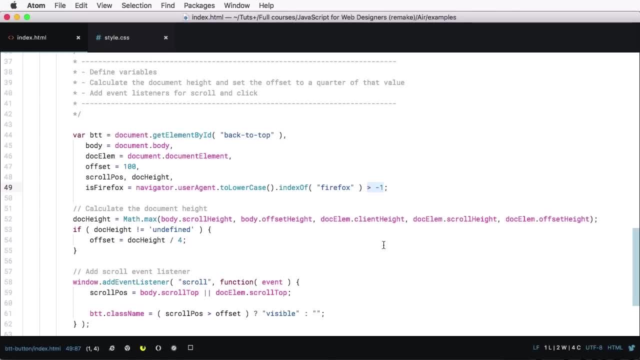 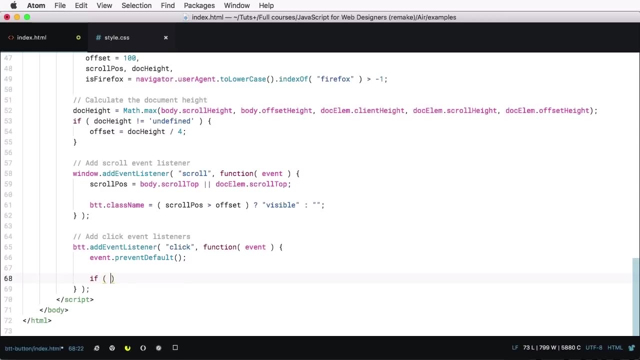 it means the word Firefox is within that string. Otherwise it isn't there. And this is a comparison. So it returns true or false. So, coming back down here, we're gonna say if is Firefox. Then we're gonna say scroll top equals zero. 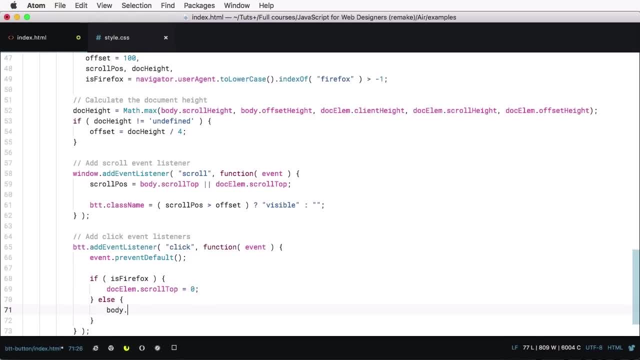 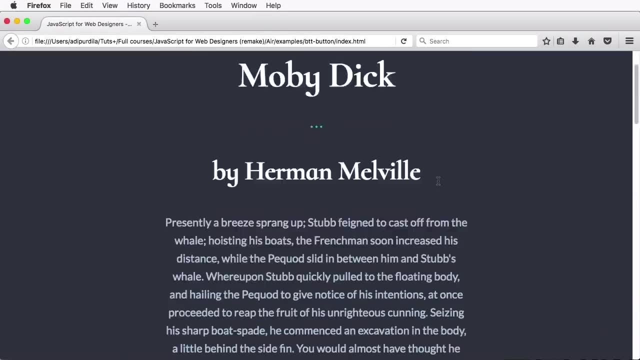 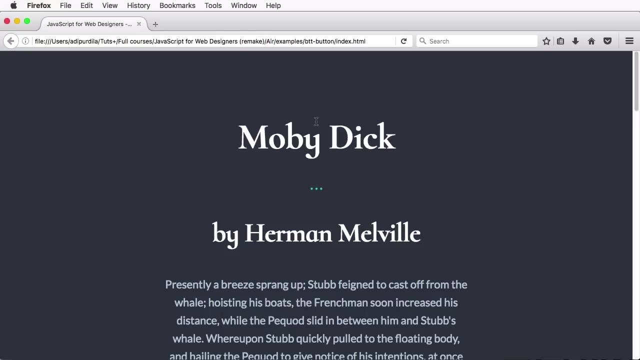 Otherwise we're gonna set body scroll top equals to zero. So now refresh, and when I'm down here I click the button. It's gonna take me back to the very top. And now that I think of it, I actually said in the beginning: 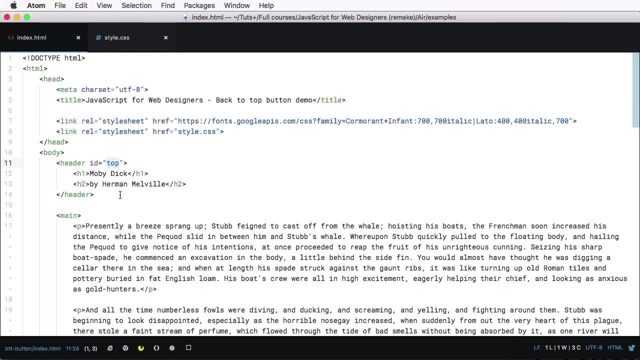 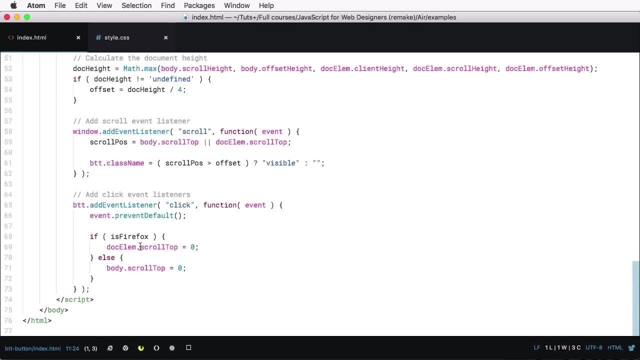 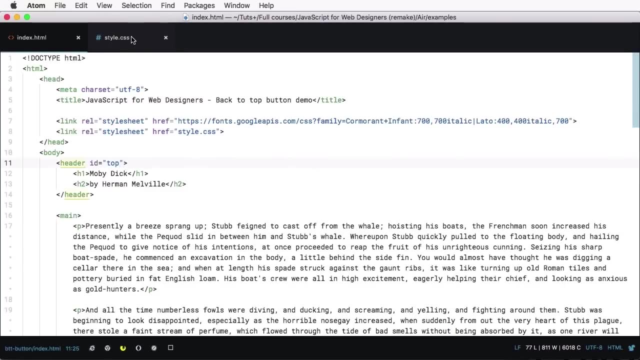 that we're gonna use this ID to bring us back to the top. Not really necessary, To be honest, because the way we're getting to top is we're setting this property here. scroll top equals zero, So we might as well just get rid of this. 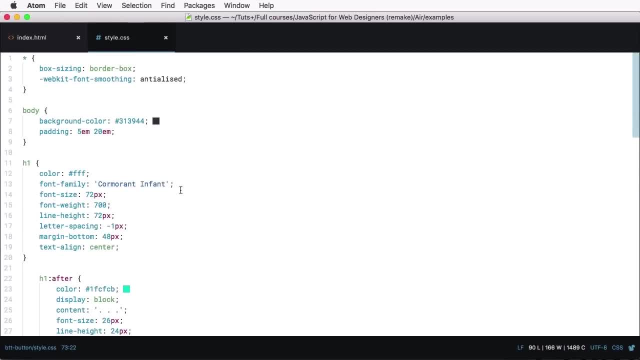 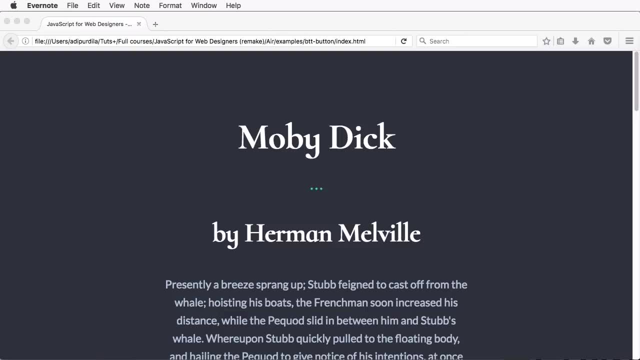 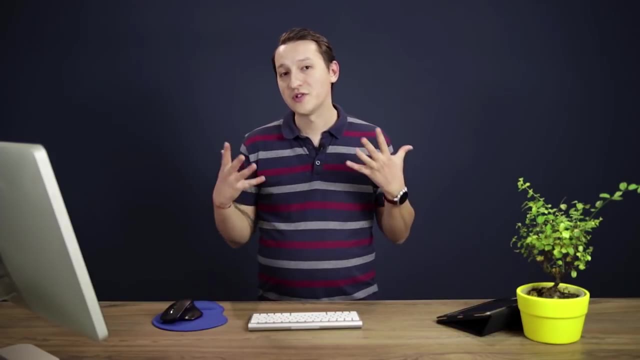 unless it has value in styling, which I don't really think it does. No, it doesn't. Okay, so we can actually get rid of this. That's about it for our button Now. a small but interesting project, Okay. 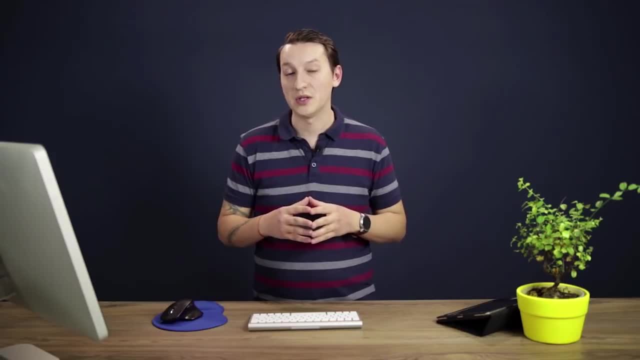 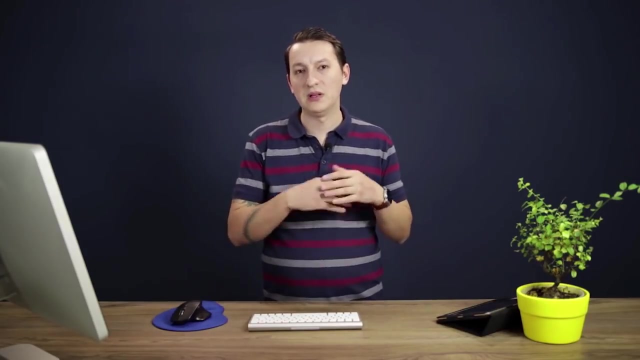 Is a text box that supports auto-completion. That will be demo number two and will be coming in the next lesson. Hello and welcome to lesson number 13,, where we'll create a text box that supports auto-completion. Now this can be used for lots and lots of different things. 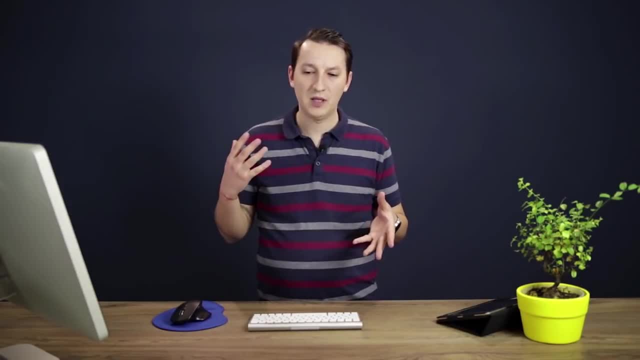 But usually auto-completion is a feature that really helps out with the user experience when it comes to filling in forms, right. So imagine you have to fill in your country, right, And you start typing and it would be useful to immediately. 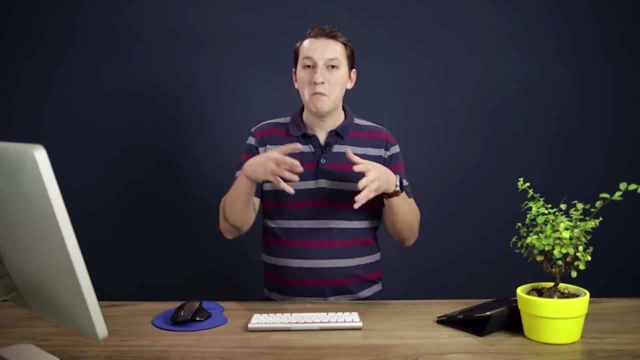 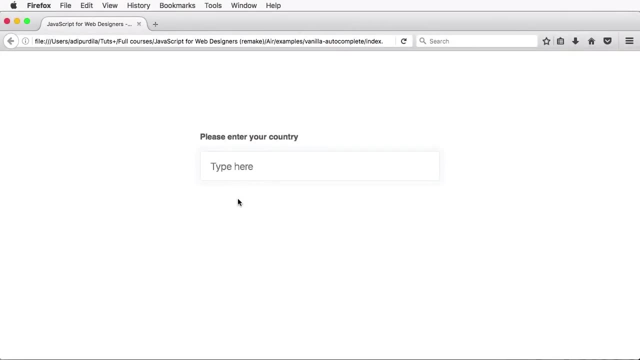 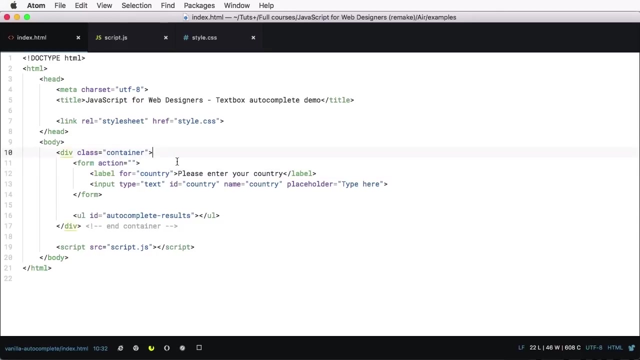 as you type, get a list of countries that match whatever it is you typed. Well, this is what we're gonna create in this lesson. So here we have our text box. currently it doesn't do anything And, coming back to the markup, we see that it's very simple. 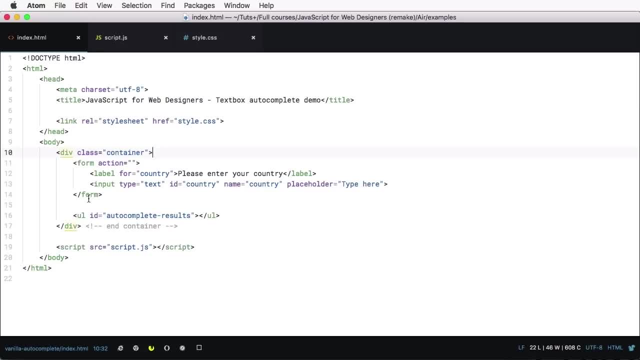 It's an input type text in a form. It has an ID, a placeholder, And below that is an ul with an ID of autocomplete results. This is the element that we're gonna populate with the various results we're gonna get from auto-completion. 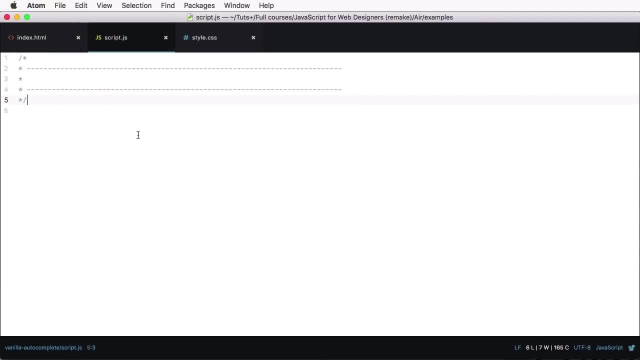 So let's start our scripts file by declaring a couple of variables. We're gonna get our actual input, we're gonna get the results And then we're gonna specify our country list, and that's about it for now. So let's actually document our step here. 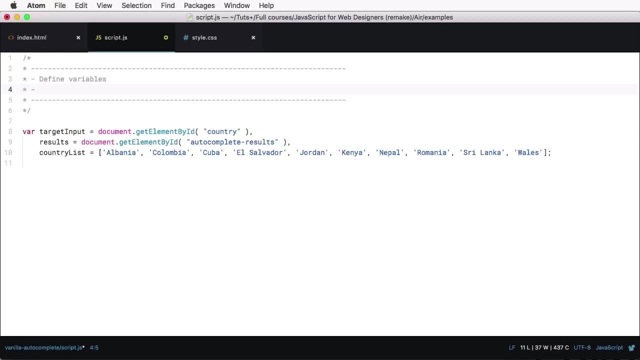 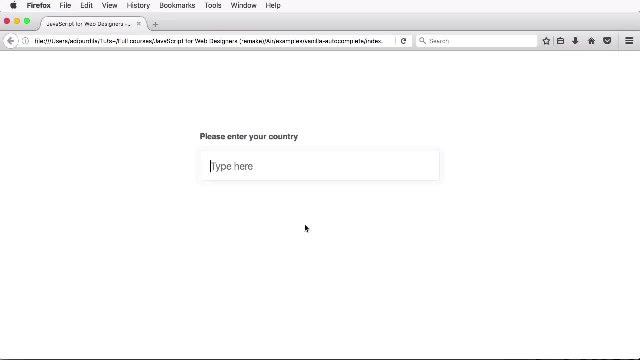 Next up, we should focus the input when the page loads, So we say targetInputfocus And that whenever we refresh now the cursor is always in there. Next up, we have to add an event listener for the key up, So whenever we press a key into the input. 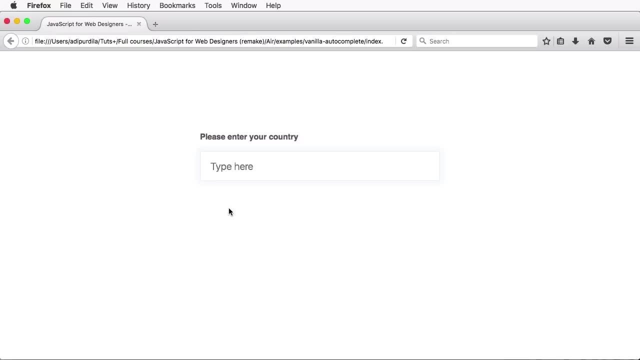 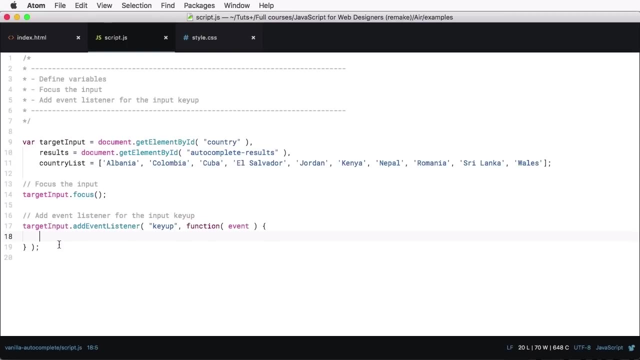 we start comparing what we typed with what we have in our country's array. We're gonna say targetInputaddEventListener. on key up, We execute the following function: Now, before we move on, we're gonna need some useful key codes here, And these are: 13 for enter, 38 arrow up, 40 arrow down. 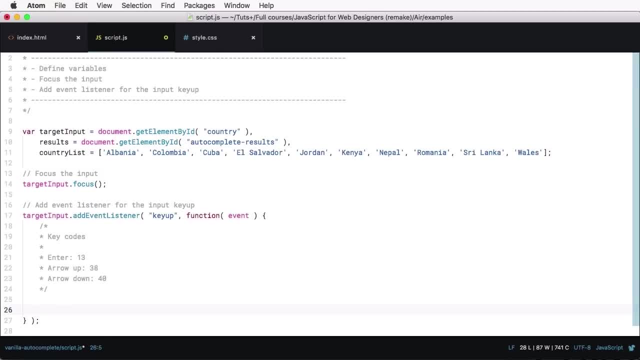 You'll see why we need these in just a little bit. Now we're gonna start by doing this resultsresult- PluralinnerHTML. now we'll reset this. So basically, if there were results previously shown, we're gonna remove those. 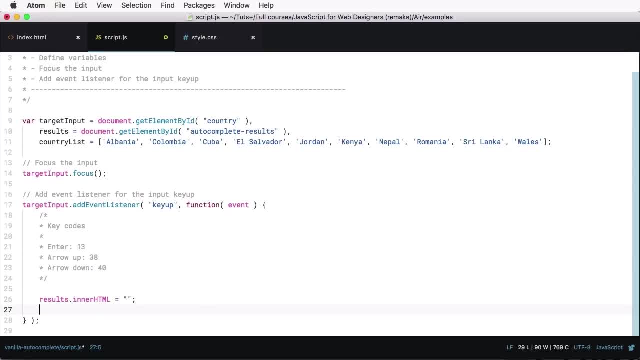 Next, we're gonna hide the results element And for that we're actually gonna write a function to which we can just pass in a parameter and it's gonna either show it or hide it, And the function is called toggleResults And we're gonna say hide. 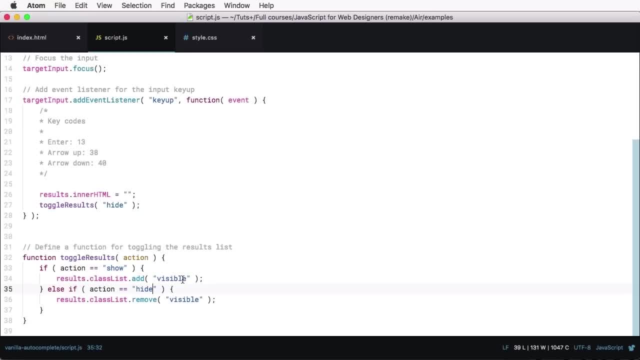 So let's go ahead and write that function, And that function looks something like this: So action is either show or hide, And if the action is show, then we're gonna get the results. We're gonna add the class of visible. Otherwise, if the action is hide, we're gonna remove the class of visible. 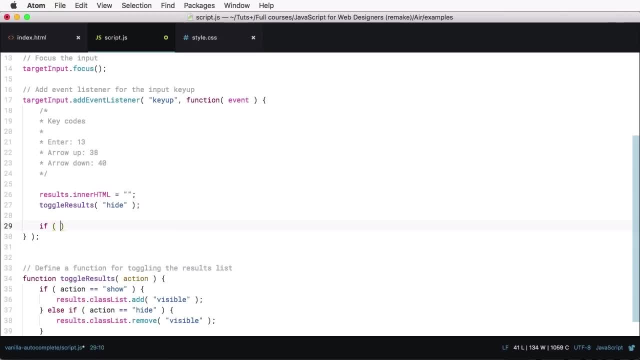 Very, very simple. Now we're gonna say: if thisvalue, and then we're gonna say: if thisvaluelength is higher than 0, then So what exactly does this mean? Well, this is an object and it refers to target input, in this case. 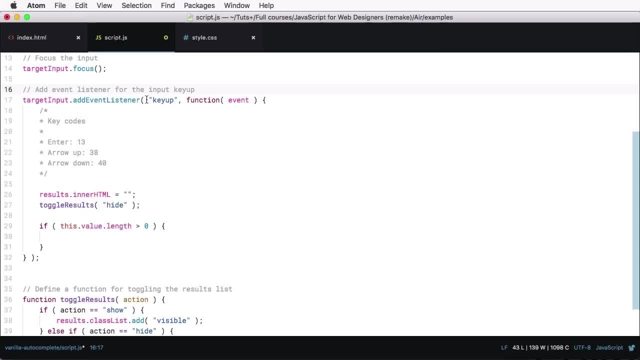 So when we're doing this target input addEventListener, we can actually use this object to reference target input And it allows us to write code more accurately. and it allows us to write code more accurately and more elegantly and more efficiently. 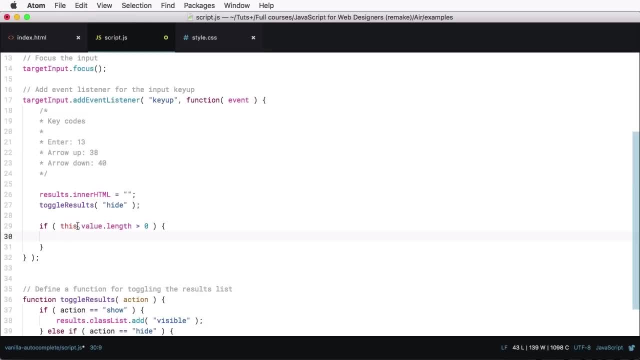 So if the value that we typed in that input has a length that's higher than 0, which means if we type something, basically, then we're gonna do the following: Matches equals to getMatches- thisvalue. Now we have two unknowns here. 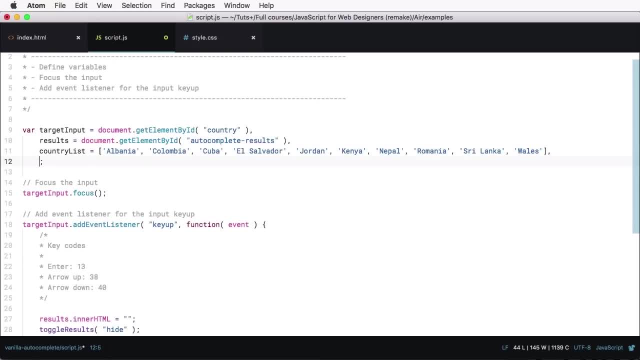 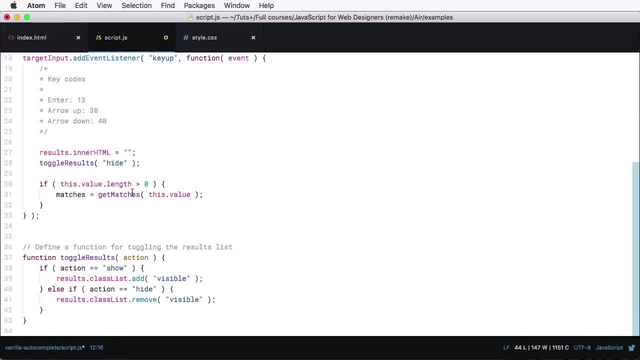 Matches is actually a variable that we need to define and it's an array, So getMatches equals array and getMatches is a function that we need to write, And that function will actually compare the value that we just typed with all the items in the array. 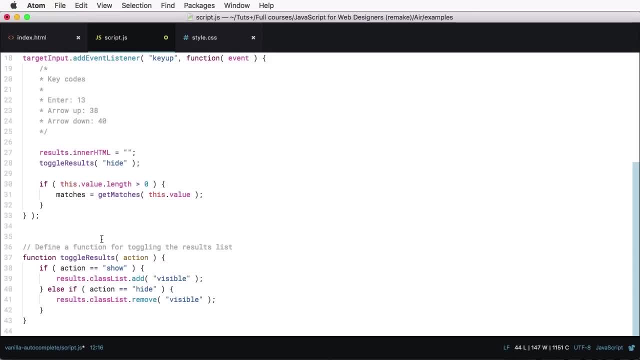 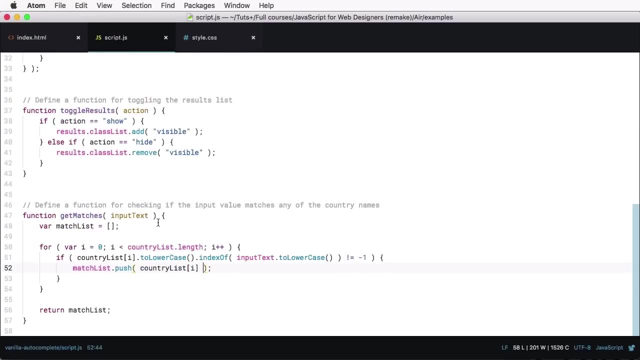 And it's gonna return an array of the items that match the value that we just typed. Maybe it sounds a bit confusing, but if you take a close look to the code, you'll see that it's actually very, very simple. So let's go ahead and write that. getMatches function. 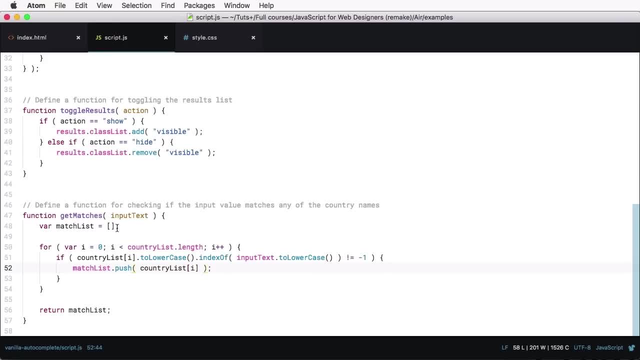 Now that function looks something like this: We're defining a matchList array and then we're parsing the countryList array, which means we're going in a loop, in a for loop, from 0 to the last item And then we're checking if the item to lowercase. 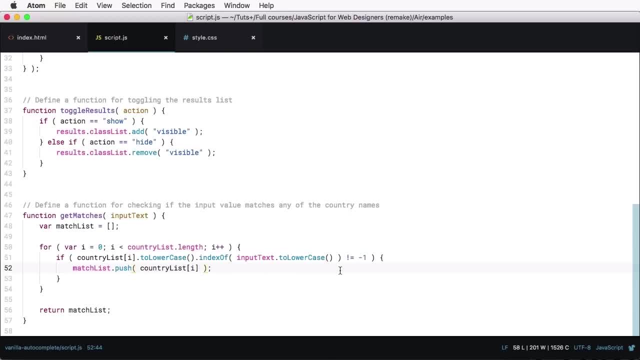 index of inputText to lowercase, inputText being this bit. So if the index of is different than minus 1, which means if the value that we typed in the text box is contained within that particular item from the country array, Well, in that case we're gonna do matchList, push that countryList. 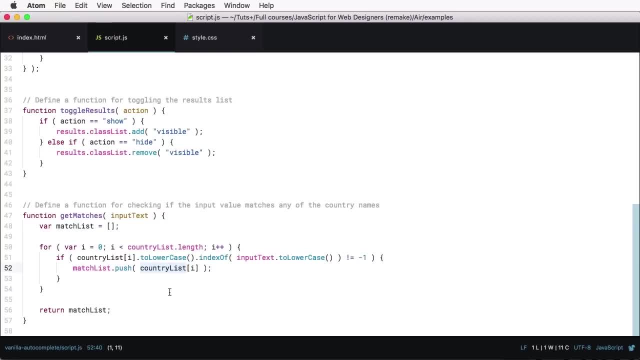 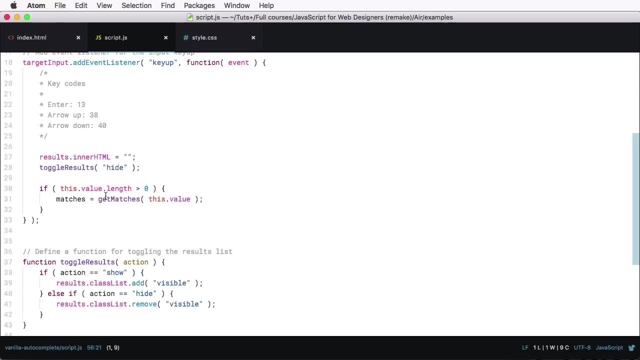 We're populating the matchList array with that country's name And then we return matchList. So now, coming back here, we'll do this: Matcheslength is higher than 0, which means if we have some country names returned by our function, then we're gonna say displayMatches- matches. 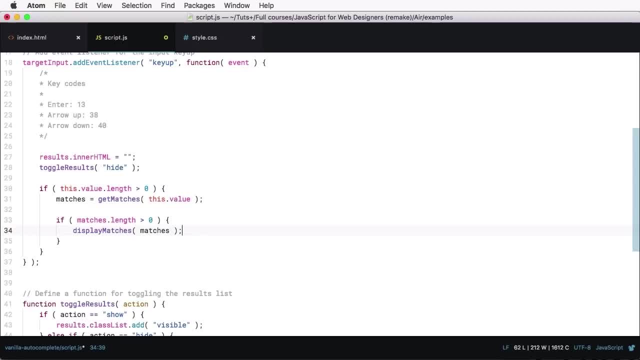 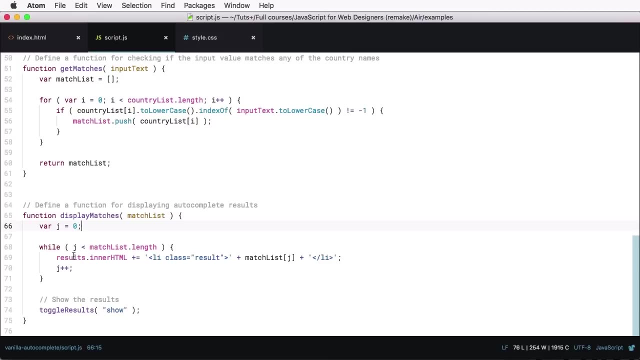 Now, displayMatches is a function that we're gonna write now, which will populate our autocomplete results And then show it. So what we're doing here, basically, is we're doing a while loop And we're going through the entire matchList array. 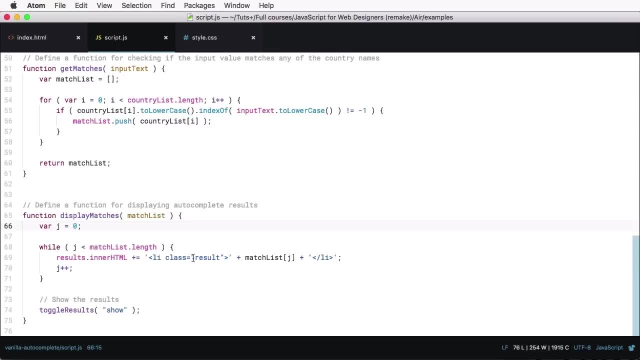 Every single item will be appended as a list item with a class of result to the results element, which in our case is this: UL. Then what we do is we toggle the results like this, or we show the results. So in this case, we're gonna show the results. 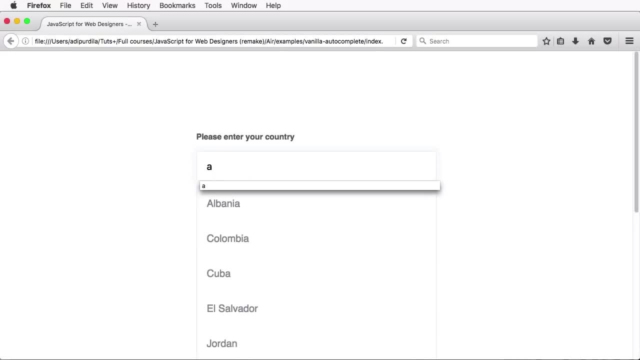 So let's see if it works. Okay, let's do A and you can already see that we have a few countries here: Albania, Colombia, Cuba, pretty much all the countries that contain the letter A. If I do AL, it shows me all the countries that have ANL. 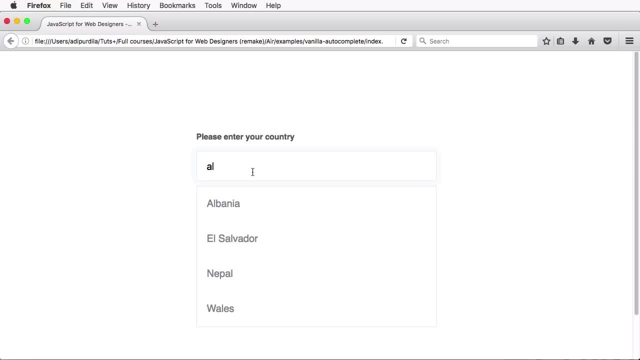 Albania, Nepal, Wales and so on. And if I do ALB, it just shows me: Albania, Let's do another one, Let's do Nepal, Let's do Romania. So, as you can see, the script works beautifully. 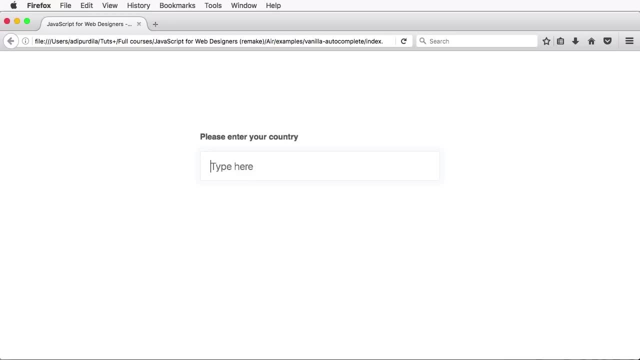 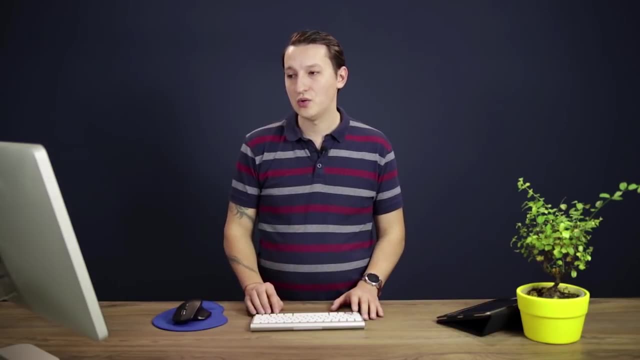 Now what I want to do is to have a little bit more control over that list when using my keyboard. So, for example, I want to be able to move through my results with the up and down arrow keys And then, when I hit Enter, I want to fill my text box with that value. 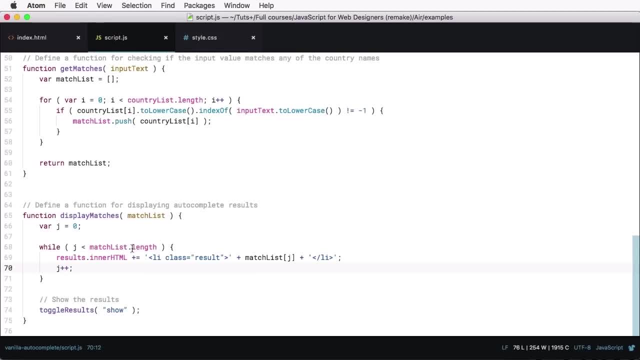 So let's make that happen And we're gonna start right here in our display matches function, We're gonna say: the first child gets class of highlighted And for this we're gonna say: move, cursor results, cursor Again. two unknowns. 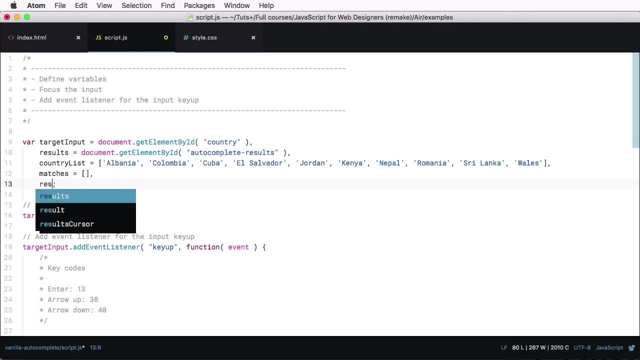 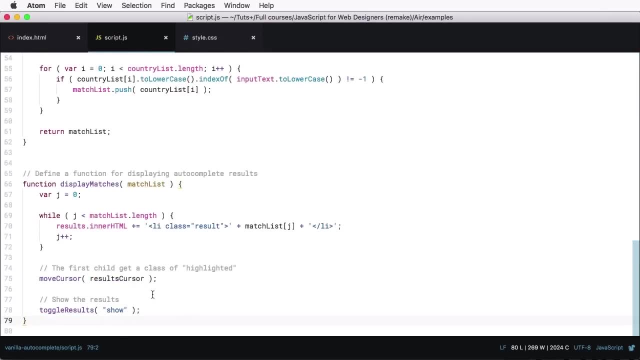 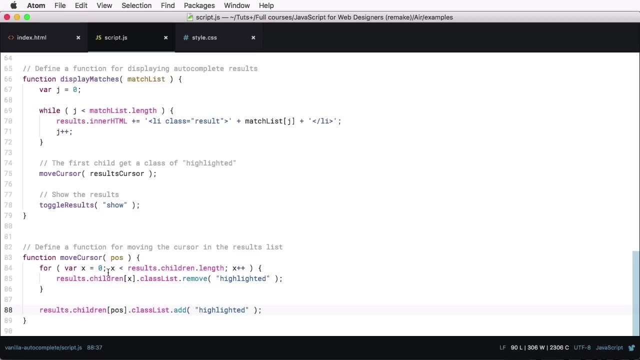 Now results. cursor is a variable that we're gonna initialize here That should be equal initially to zero, And move cursor is a function that we're gonna write now. Now the move cursor function will basically move that highlighted class up or down, depending on which key I press. 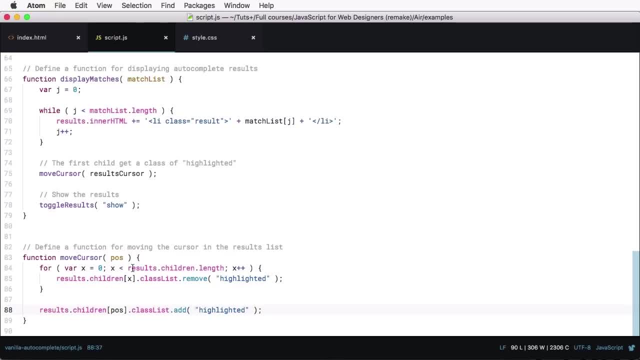 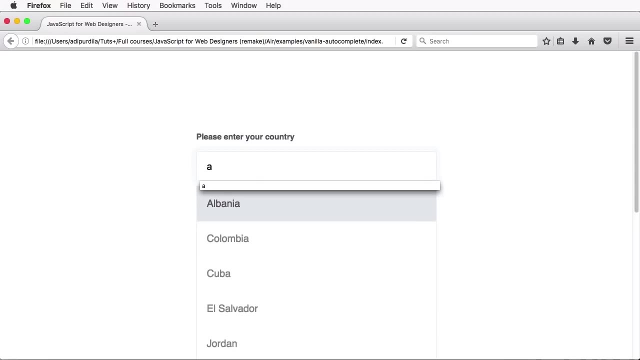 So what we're doing is basically we're going through all of our results, We're removing the class of highlighted from all of them and we're adding that one only on our position. So now refresh. You can see that when I type something. 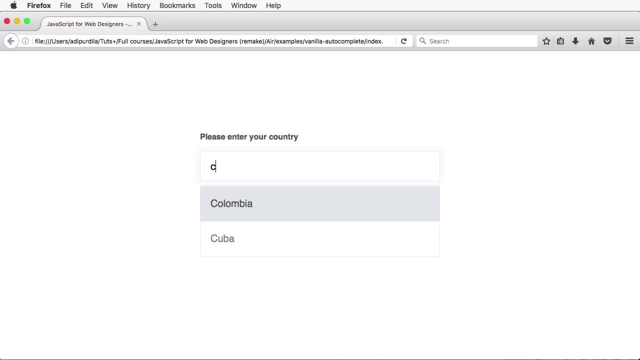 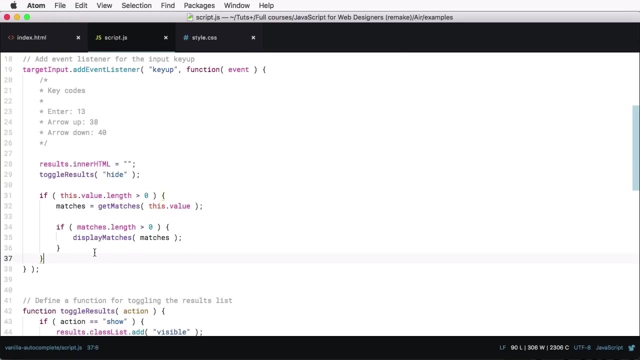 the cursor or the highlight is on the very first item. Now let's see what we can do about when we press the up and down arrow keys And the place to write that code is right here in the key up event listener. So here we're gonna say: if results class list contains. 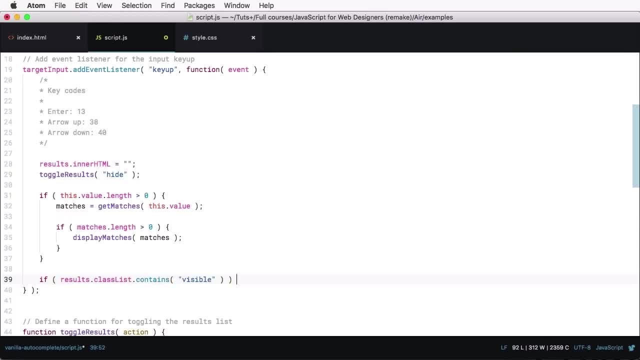 visible. So if there are results that are being shown, then we're gonna do a switch, And a switch is a much more elegant form of writing multiple if-else statements. So we're gonna do switch and the criteria is going to be eventkeycode. 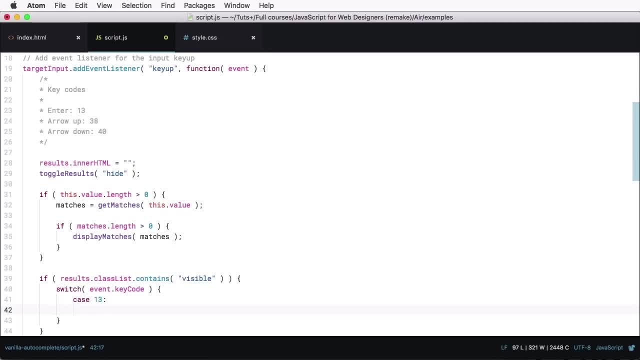 And then we're gonna say case 13, we're gonna have our block of code, and then we're gonna have break, Case 38, again block of code, and then break, And finally case 40,- same deal. 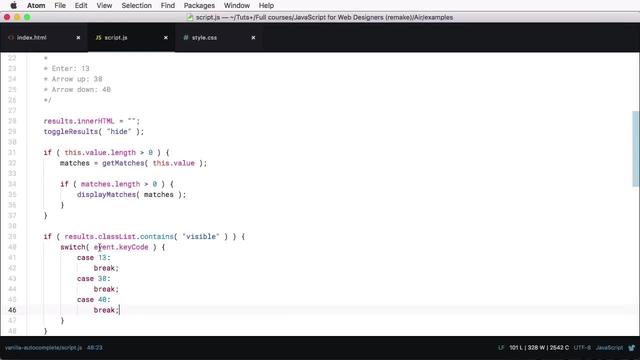 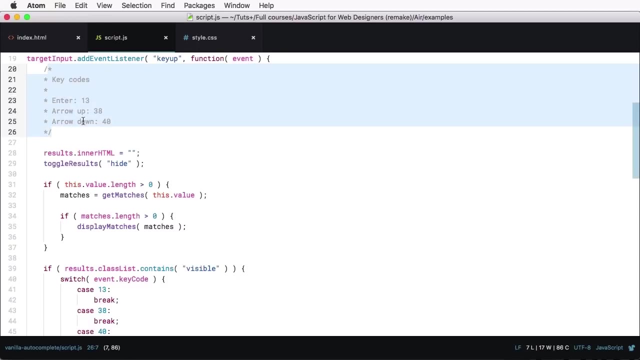 Okay, now what this means, basically, is check the event key code. If it's 13,, execute the following. If it's 38, execute the following, and the same goes for 40.. Now, this is where this comment comes in. 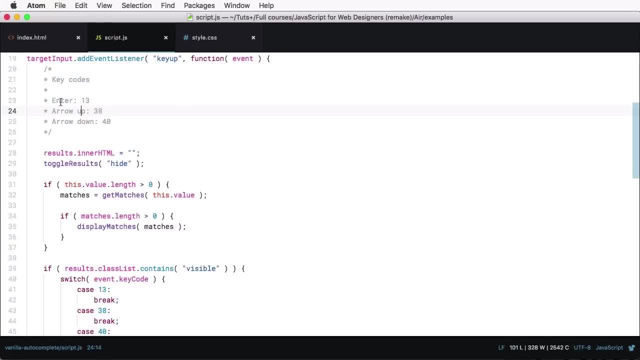 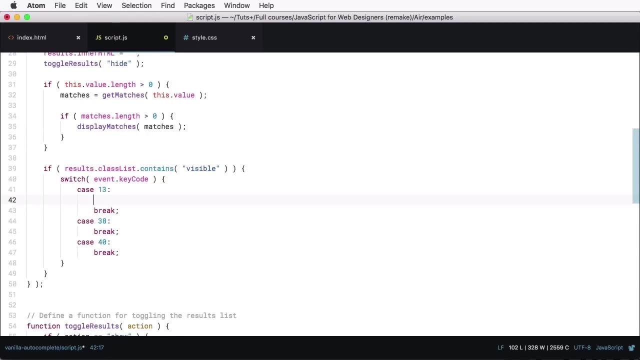 You can see that 13 means enter, in which case I want to copy or I want to fill in my text box with the value that I've just highlighted: 38 and 40 arrow up and respectively down. So, in the case of an enter, I want to do the following. 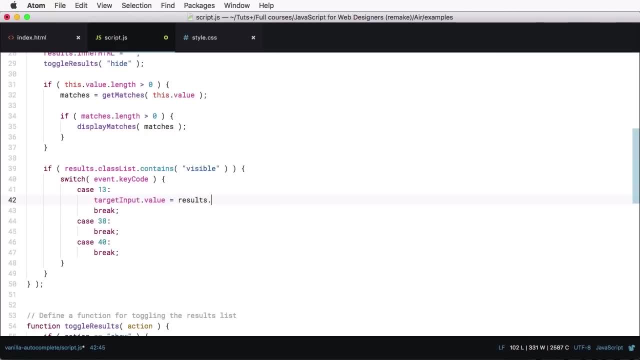 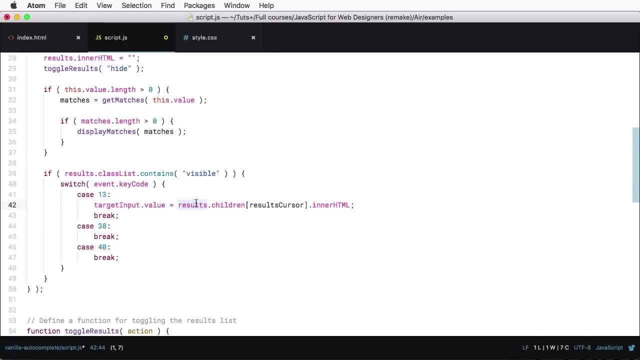 Target input value equals results, children, results cursor, inner HTML. Well, resultscursorinnerHTML Is our UL. Children means each individual list item, A result cursor is the position that's highlighted And innerHTML basically means the text within that list item. 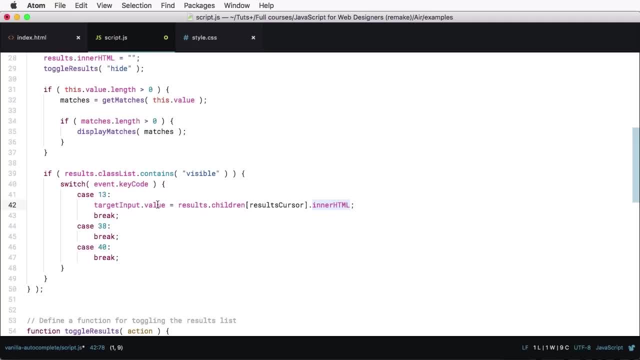 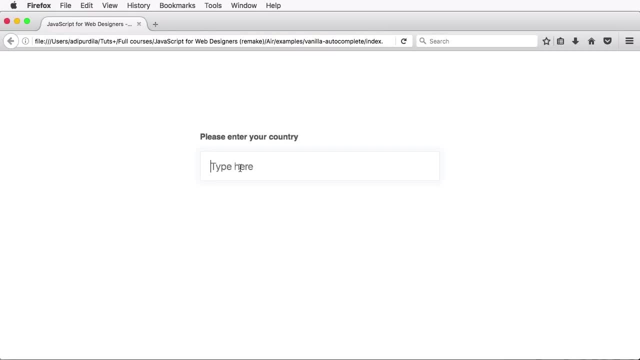 That's all there is really. So we're taking this value and we're assigning it to the target input value. So let's see that in action. Let's see, Let's type Romania. If I hit Enter, you can see that the page refreshed there. 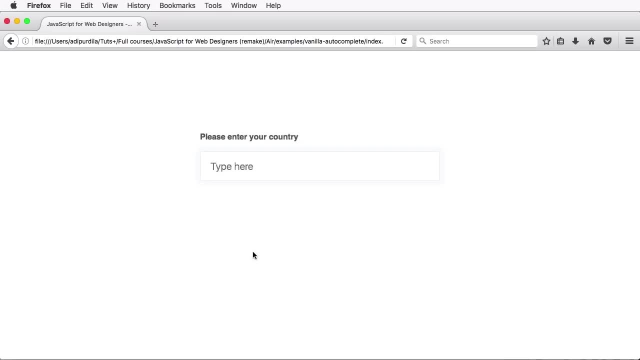 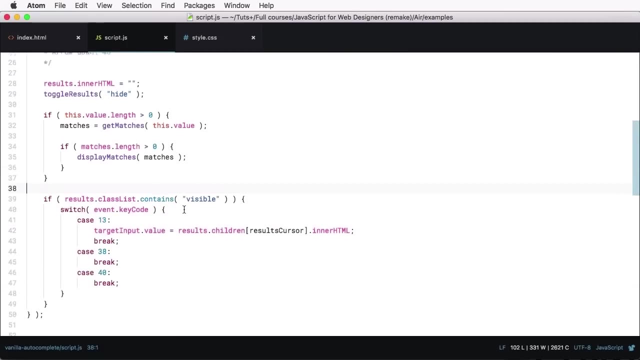 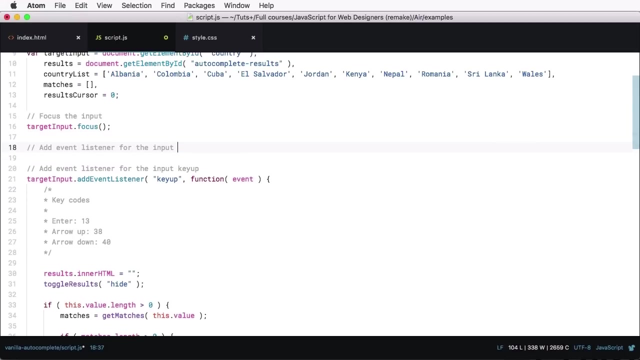 And that's because this is a form. Pressing Enter in that form will automatically submit it and the page refreshes. but we don't want that. To prevent it, we're gonna go right here and we're gonna add EventListener for the input key down. 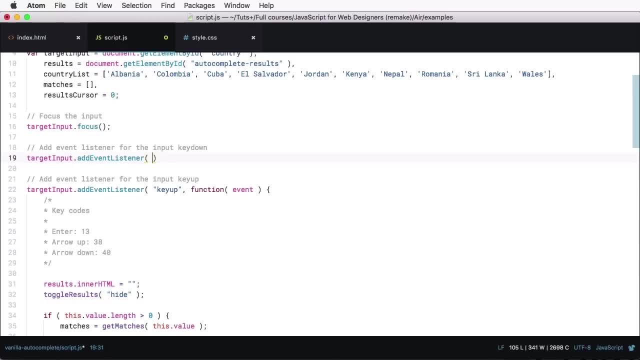 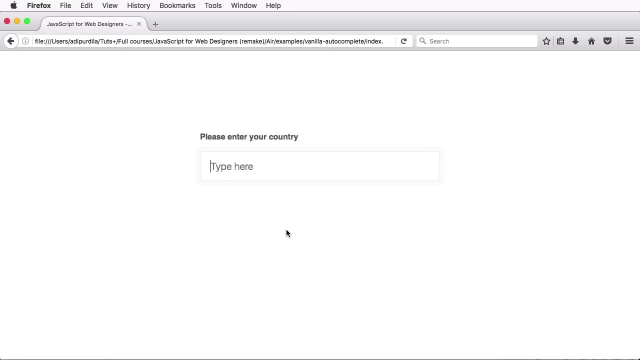 So we're gonna say target input, AddEventListener key down function And we're gonna say: if eventKeyCode equals 13, or if we press Enter we're gonna say eventpreventDefault And that if we type Romania again hit Enter. 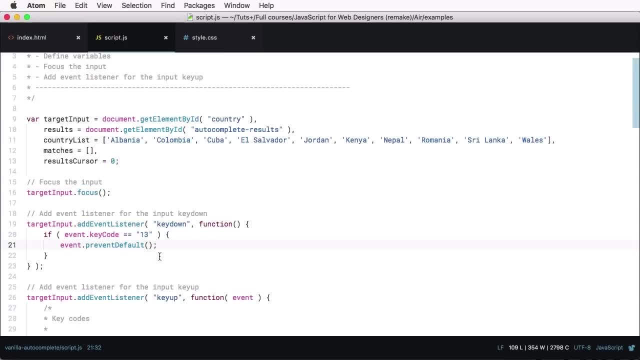 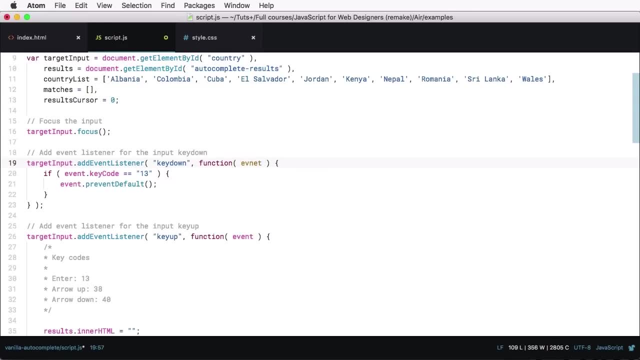 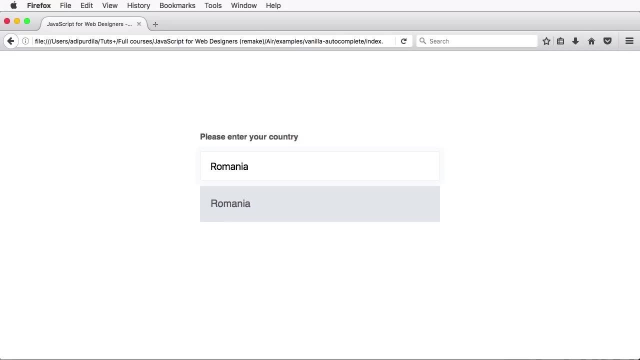 Hm. for some reason this still doesn't work. So what's going on here? So AddEventListener key down function. sorry, I forgot to include the event here. Okay, let's do a refresh. So Romania hit Enter and we now populate the text box. 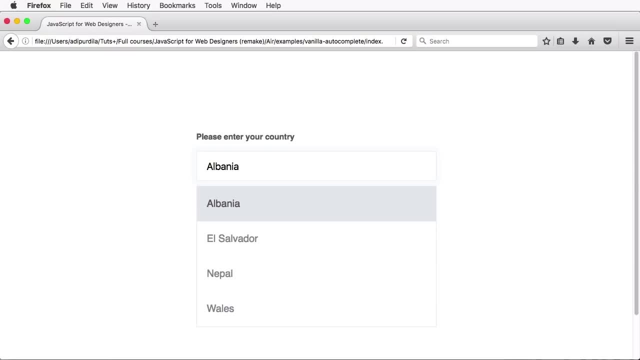 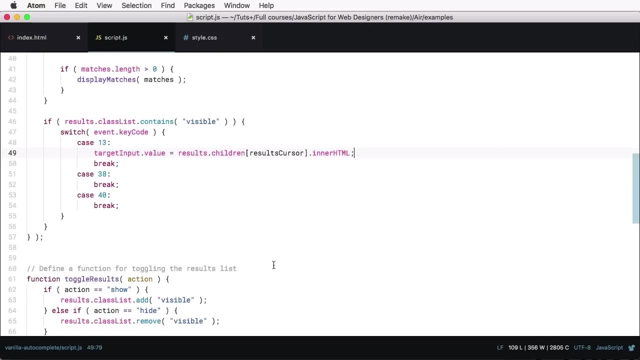 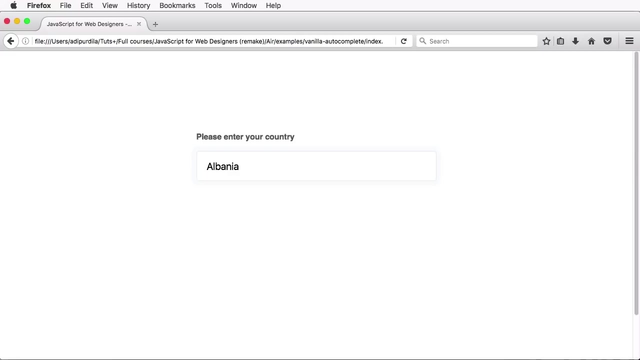 Let's do another test: Albania- Enter. okay, But when I hit Enter I want to actually hide this results element. So here we're gonna say: toggleResults hide. And also let's reset the cursor to 0.. Okay, refresh, let's try that again, perfect. 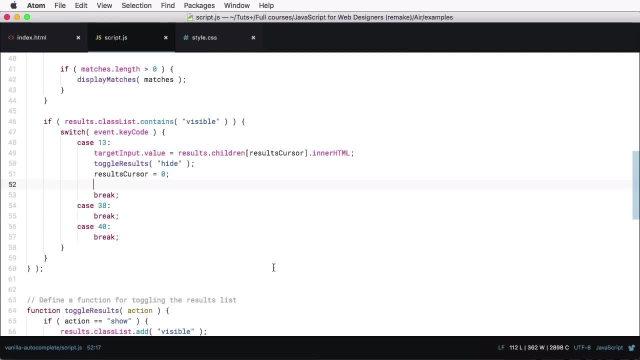 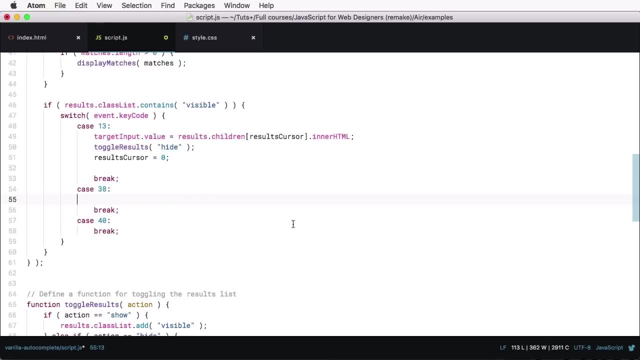 All right. now let's see about moving up and down in this list. On 38,, which is arrow up means we have to go up, We'll simply say: if resultsCursor is higher than 0, then we'll simply do resultsCursor minus minus. 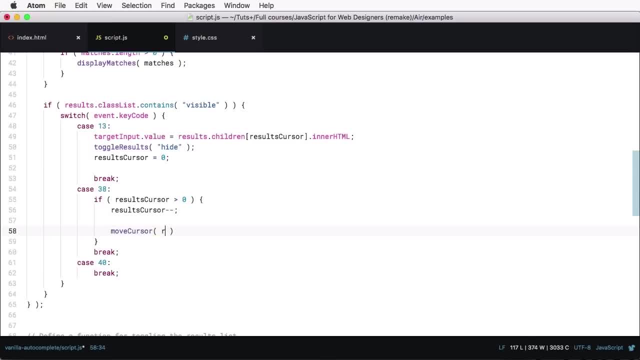 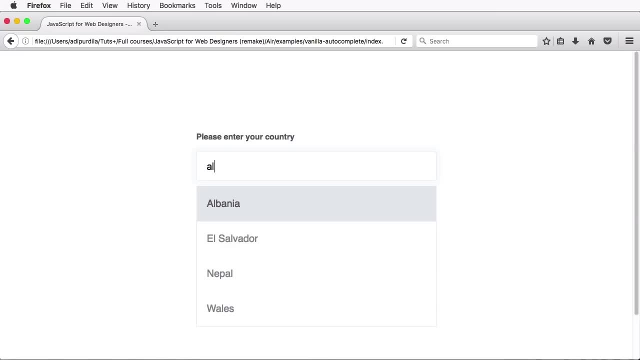 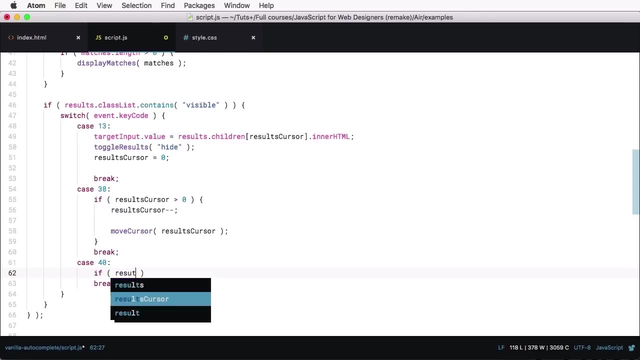 And we're gonna say: we're gonna move the cursor to the new resultsCursor. Let's see Albania arrow up. okay, Let's actually do the arrow down first. Here we're gonna say: if resultsCursor is smaller than matcheslength minus 1,. 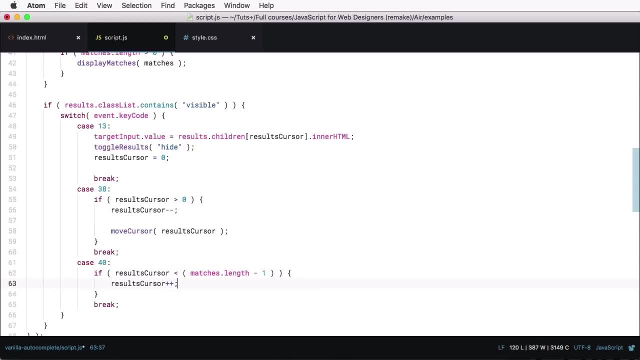 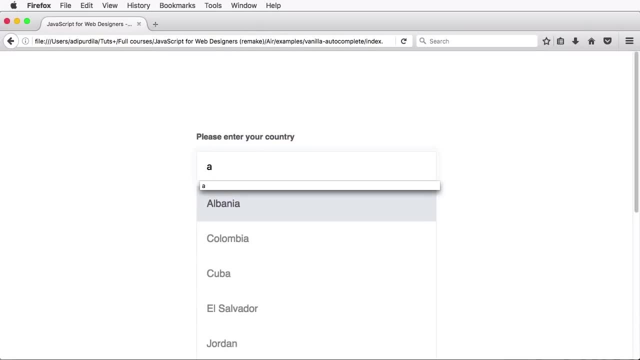 then we'll do resultsCursor++ and move cursor resultsCursor. okay, Let's do that again. So now when we hit the ArrowDown key, we can see that our cursor. well, apart from this pass key, auto, complete thing from the browser. 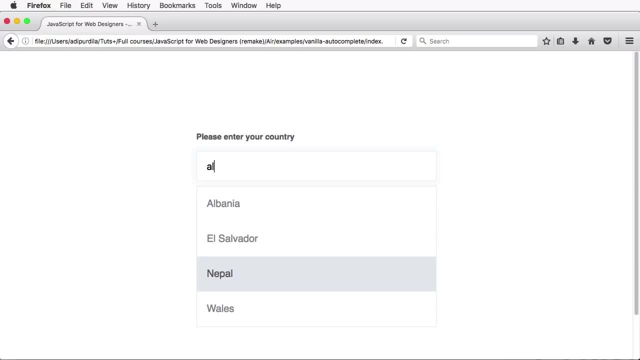 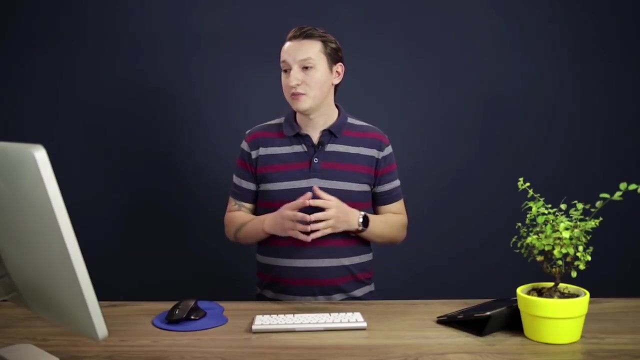 But when we hit the Up and Down arrow keys you can see that we can cycle between our results and hitting Enter on one of them. then we'll fill that into our text box And that's about it for this lesson. It's time to move on to our third demo. 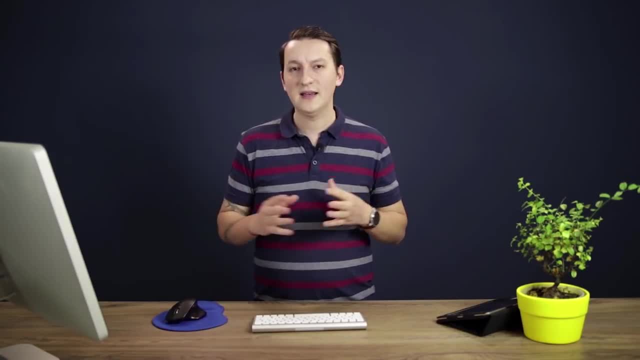 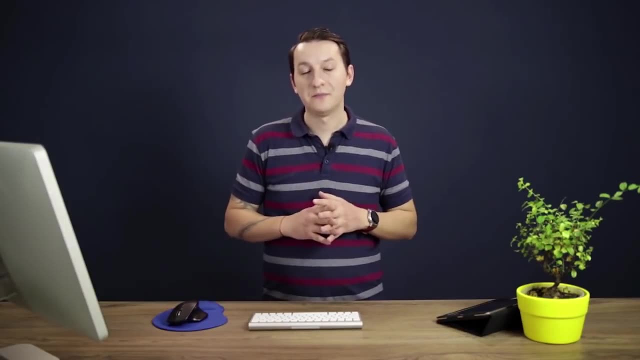 And I think that one is gonna be pretty popular because it is a content slider. So I'll see you in the next lesson. Hello and welcome to lesson number 14.. For our third demo, we'll have a look at a content slider. 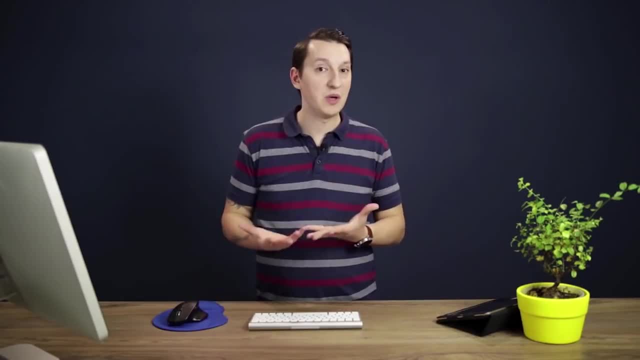 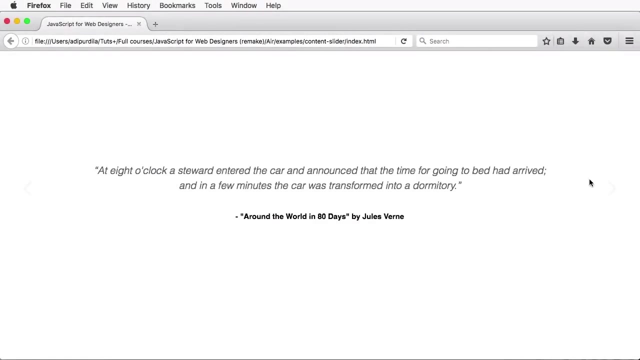 But we're not gonna limit ourselves to just images as slides. Instead, our slider can really take on any kind of slide, Text, HTML, whatever we can throw at it. Now I'm gonna show you the slide. It's the finished one. 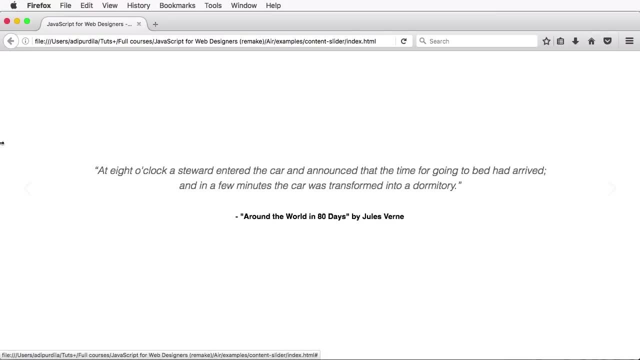 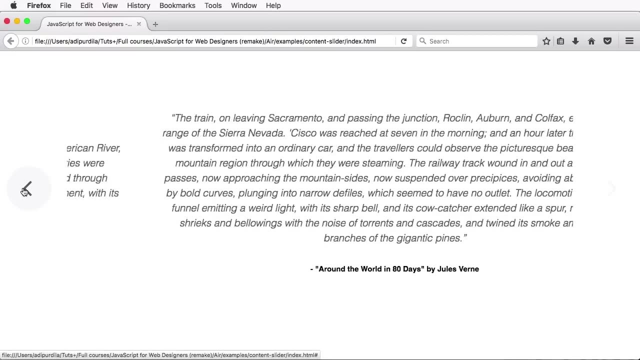 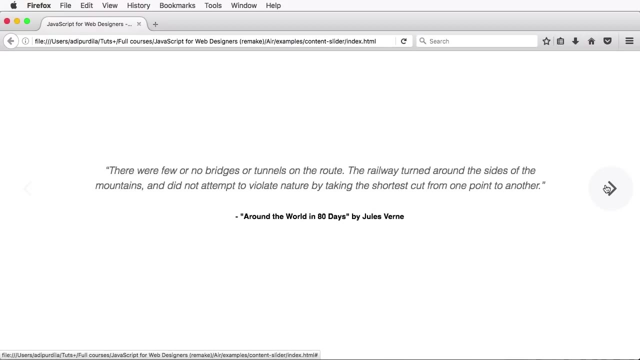 We just have some quotes here. We have the Next button, the Previous button- And we can cycle through the slides Through them like this: When we are at the beginning, the Back button doesn't work, And when we get to the end, the Forward button doesn't work. 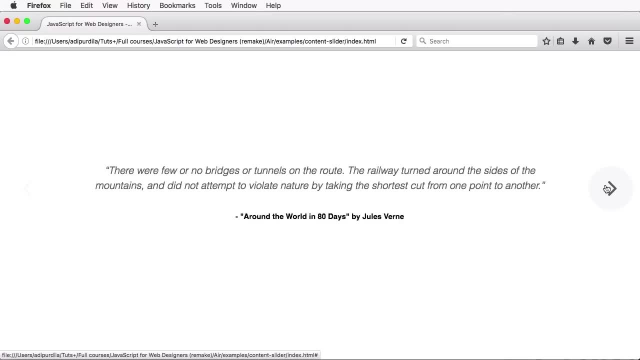 So, instead of wasting a lot of time writing this code, essentially you can just open the source files that come with the course And then just copy the code from there. I'm gonna walk you through the code. I'm gonna explain why I did what I did, and 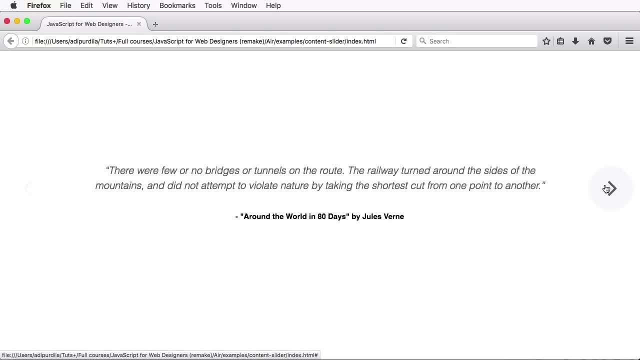 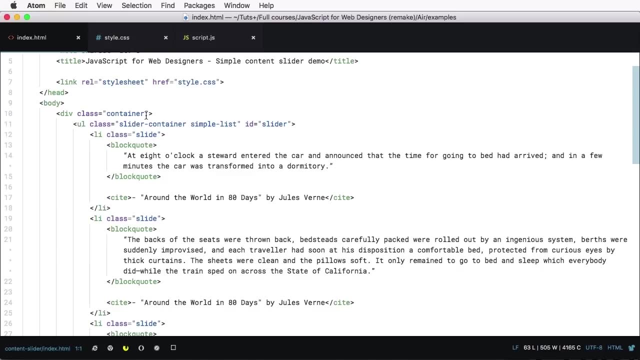 what's the purpose of each function and of each piece of code. So first things first, let's have a look at the markup here to understand what's going on. So we have a container that has a slider, container ul with an id of slider. 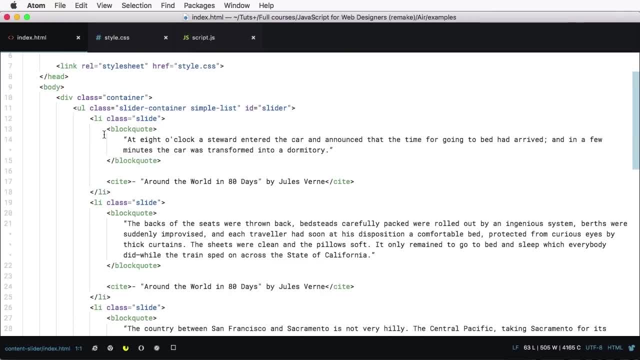 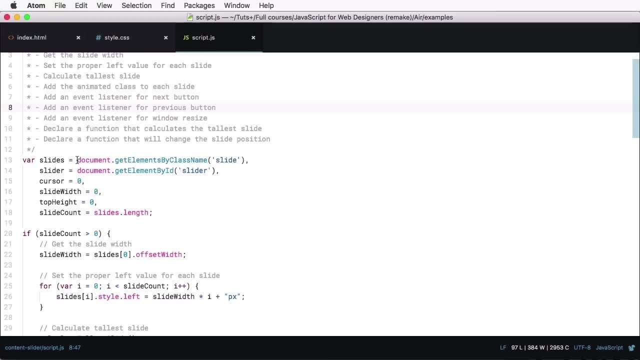 And each slide is basically a list item with a class of slide. So we start by defining a couple of variables. We're getting the slides and we're getting the slider itself. We're setting the cursor to 0.. Now the cursor is gonna serve as a guide, so 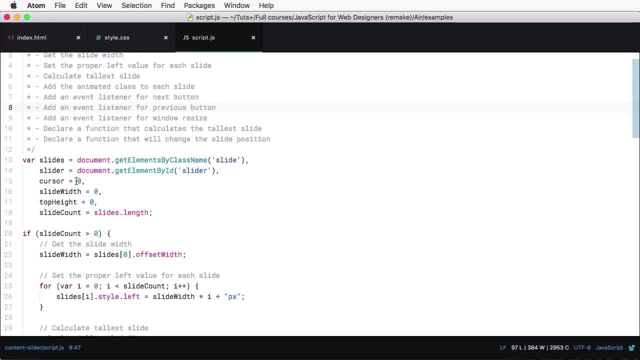 that it's not just a guide. So we're gonna set the cursor to 0.. Now the cursor is gonna serve as a guide so that we know on which slide we are. We're also defining slide width, a top height. Top height will be used to find the height of the tallest slide. 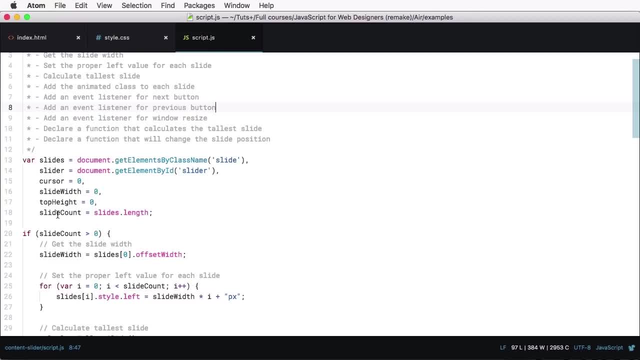 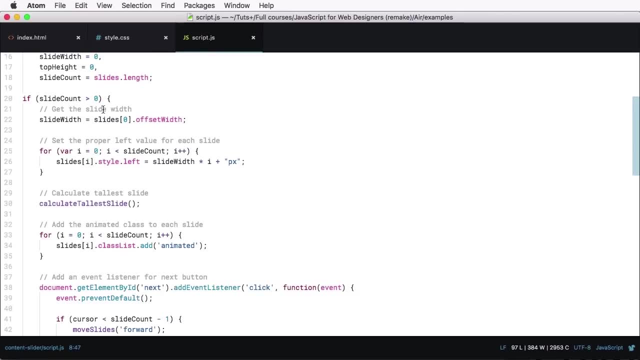 Slide count, of course, gives us the number of slides. Now, if we have slides- this is a check that we have to do- Then we're getting the slide width. Now, why are we doing that? Because the way we're gonna organize things is we're gonna have the slides. 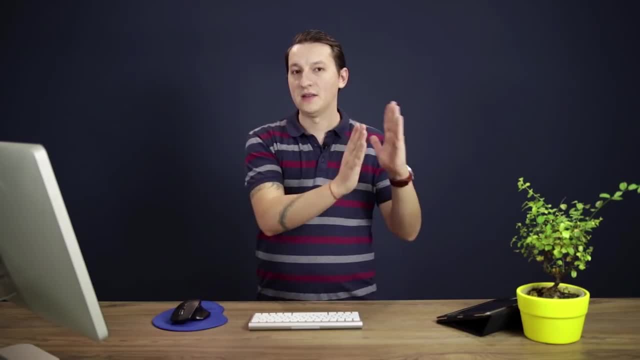 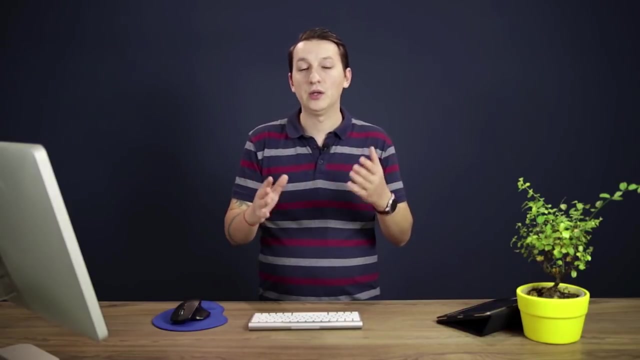 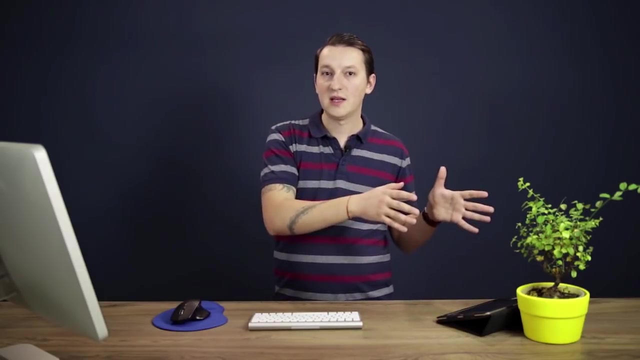 positioned absolutely and we're just gonna offset them by their height. So the slide that's currently being viewed is gonna be at left 0.. But the slide before it is gonna have the value left minus the slide width. The slide before that the same way. 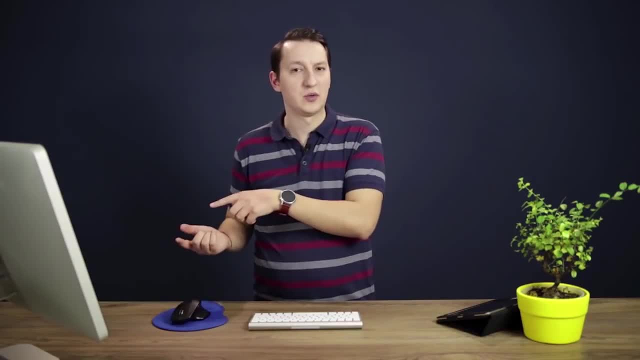 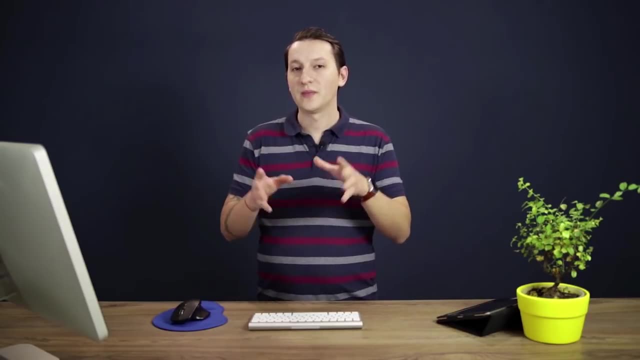 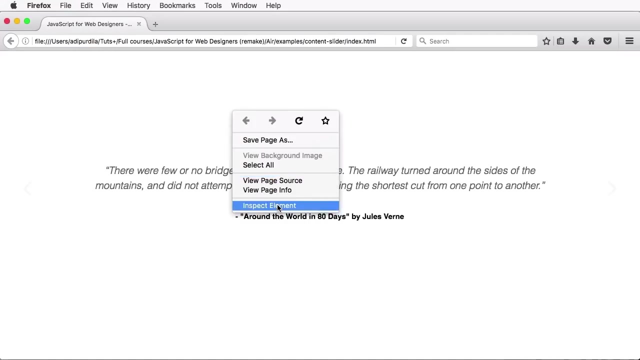 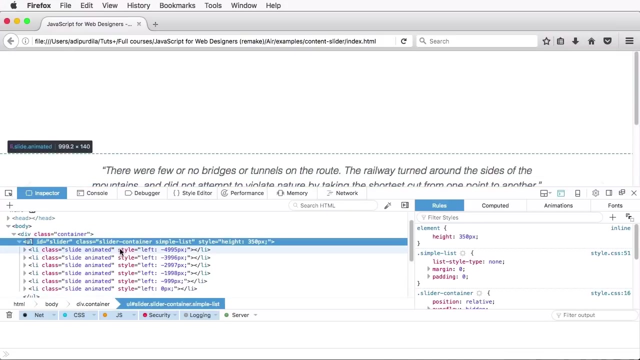 And the slides after the current one are gonna have the left value equal to plus the slide width. So let me actually show you that right here. If we take a look at the inspector, you're gonna see that our slides have a style set. 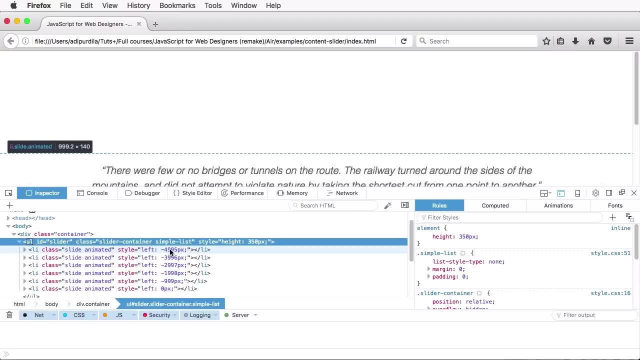 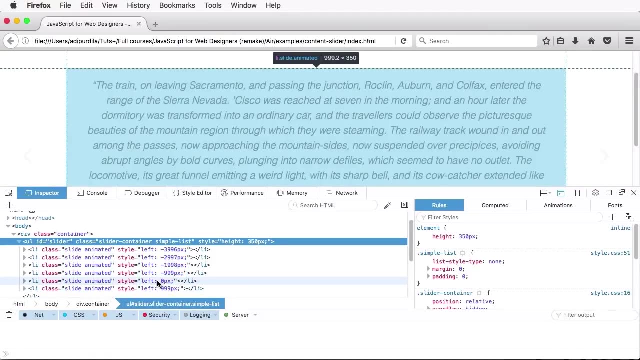 Look this first one: 4,994.. 95 pixels. and then we decrement like this until we get to 0,, which is the current slide. But if I'm gonna hit back, watch what happens with the left values. Now, this slide is the current one. 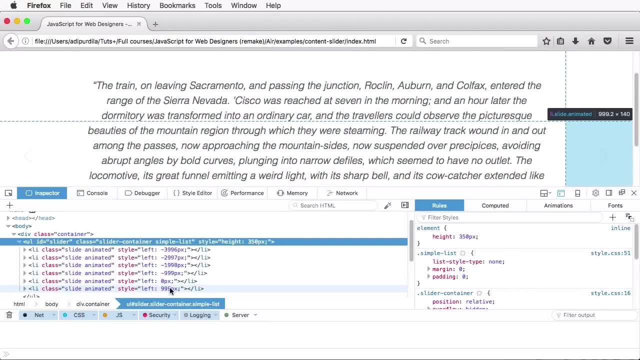 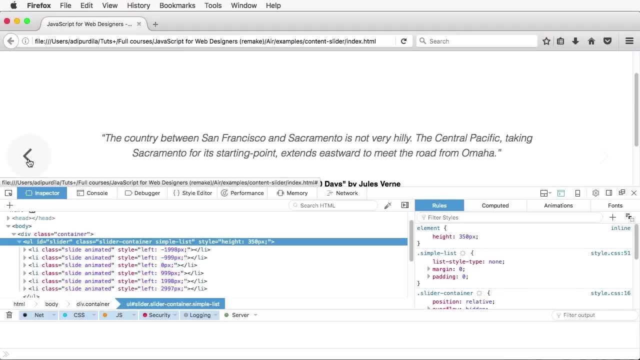 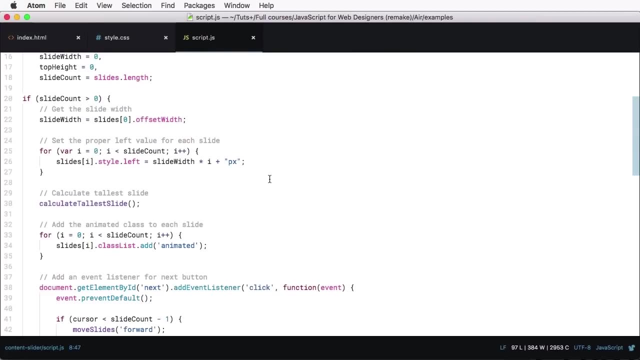 It's left is at 0.. And the one that was before is at left, 999.. We do back again. You'll notice that the value of the left property property changes. So how are we achieving that? Well, we're setting the left value for each slide here. 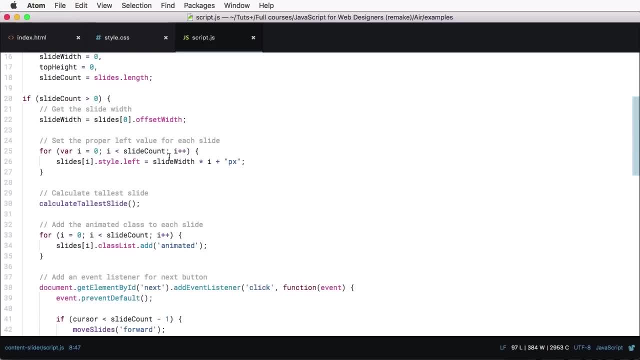 So we're doing a loop And then on each slide we're setting its width times this counter plus pixel. So if each slide's width is 1,000 pixels, then the first slide is gonna be 1,000 times 0,. 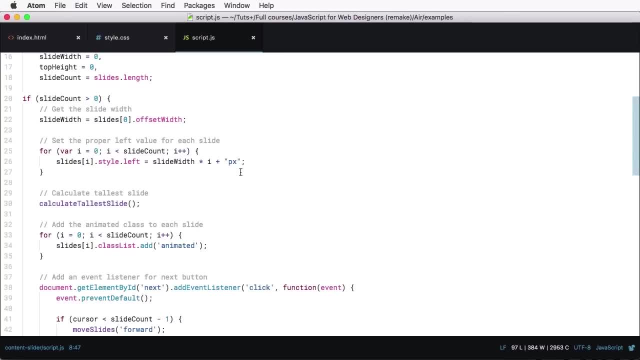 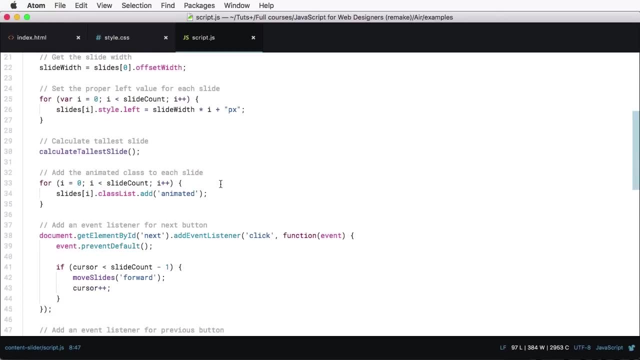 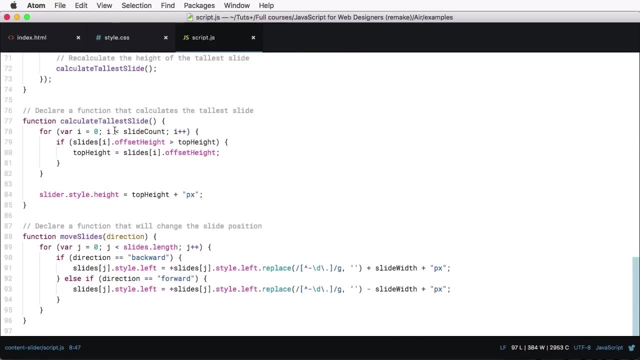 because the cursor is at 0, so that will be 0. The next one is gonna be at 1,000, the next one at 2,000, and so on. Then we calculate the tallest slide, And calculateTallestSlide is a function that basically runs through all of our 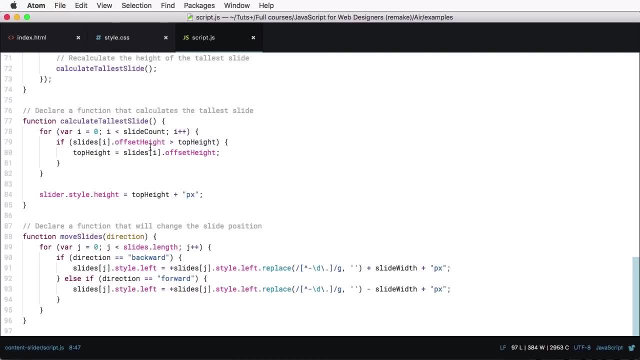 slides And it checks if the offset height of each slide is higher than the top height or the current top height, then we're setting the top height to the height of that slide. And then what we're doing is we're setting the the height of the entire slider to that top height. 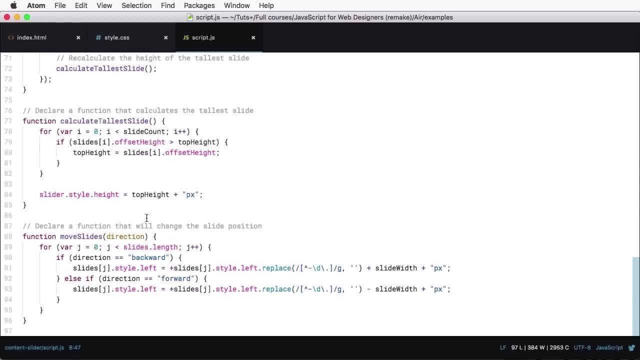 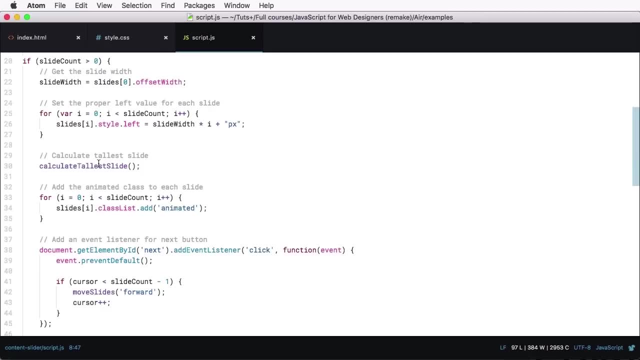 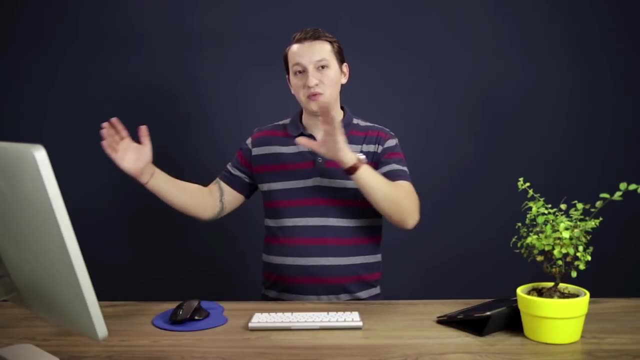 And we're doing this to ensure that all the slides are centered vertically And, of course, to do that we need to know the biggest slide. Next, we're gonna add the animated class to each slide And the animated class will basically allow for that smooth slide. 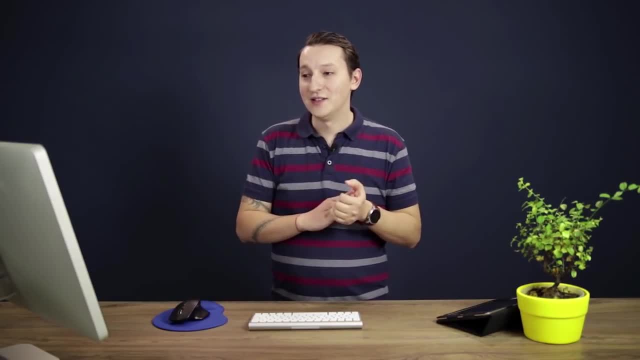 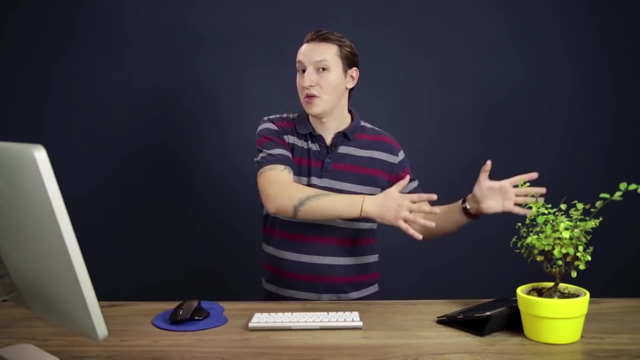 Well, slide is probably not not a good- not a good uh slide term here, but the transition right, So changing its left from 0 to minus 1000,, for example, is made with a transition. Now why aren't we adding this from the 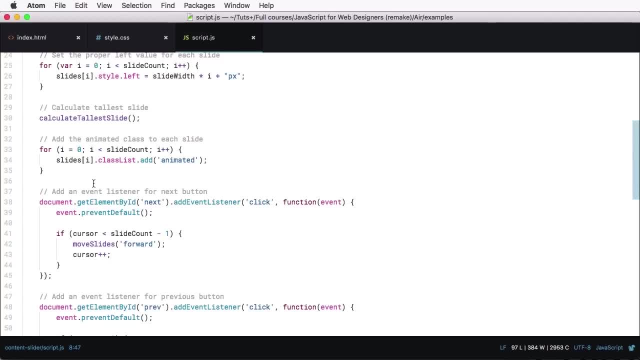 beginning. Well, if we did, when we refresh the page all of the slides would just go flying on the screen because they would have that animated class. So instead we're adding: after all the elements have loaded, Then we're adding event listeners. 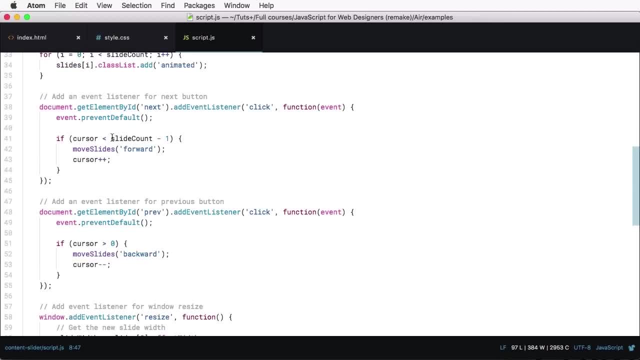 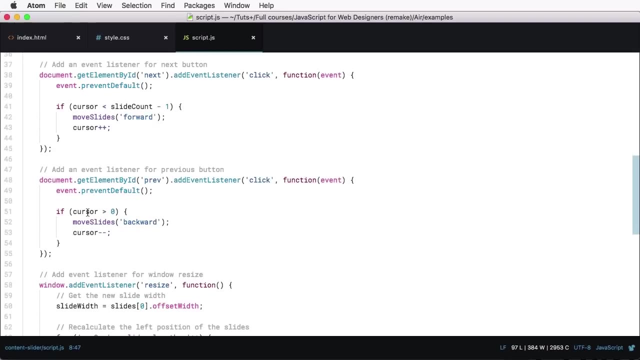 for next and previous buttons and we're checking if the cursor is smaller than the slide count minus 1, which means if we haven't reached the end, we move the slides forward and we increase the cursor. Same thing for this bit, only in. 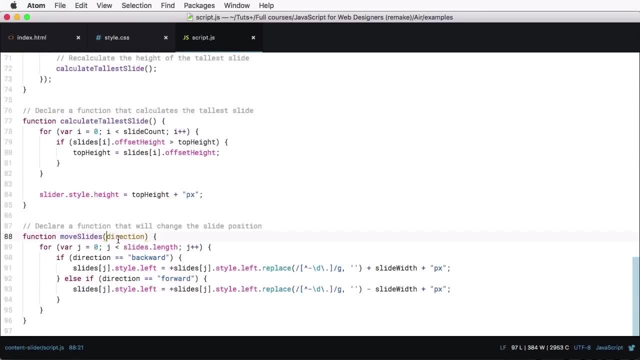 reverse. Now moveSlides will take the direction, so it's either forwards or backwards and what it's gonna do is it will redo those left values right? So the left values, as you saw when I showed you the inspector, when you're moving a slide, all of those values change. Let me show. 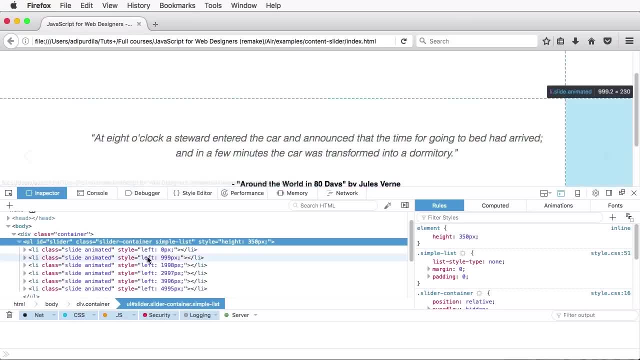 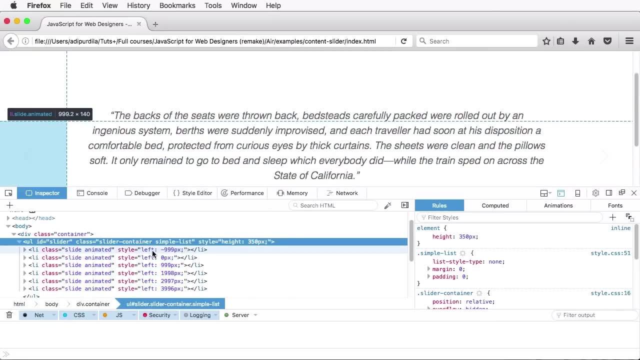 you again. So when I hit the Next button, notice this slide. here We're going to the second one. So the first one gets a left of minus 999,, second one is 0,, next one is plus 999, and so on, And that's what this code here is doing, basically. 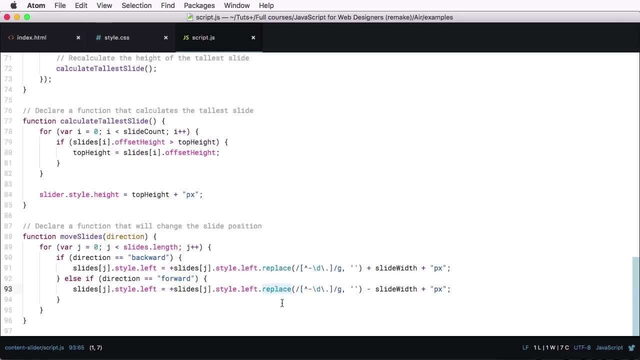 The replace that you see here basically has the role of stripping the value from the PX characters. It's always doing, And then we're adding slide width, and then we're adding pixels again so that it's compatible with this left property here, Finally, we're adding an event. 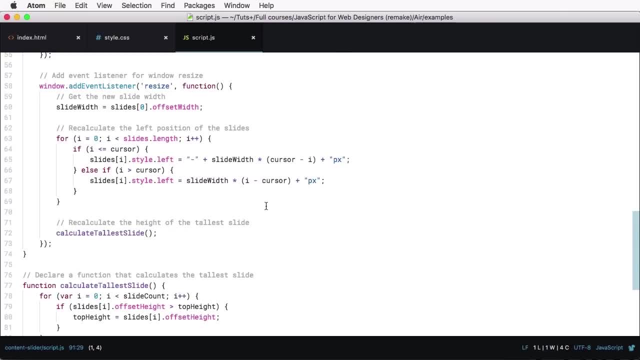 listener for resize, because when we resize our page the width of our slides will change because it's responsive. So that means the left values will be rendered useless. We have to calculate new ones, and that's what we're doing here, basically is we're recalculating those left values and the tallest slide. 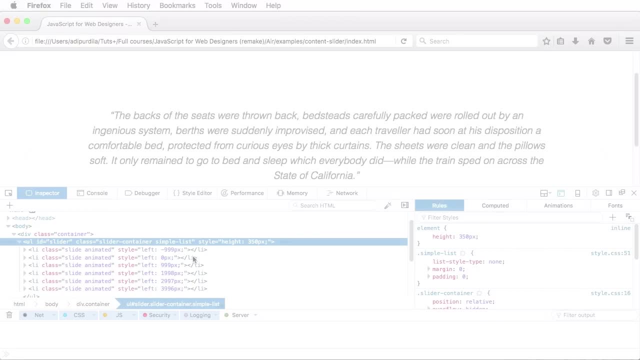 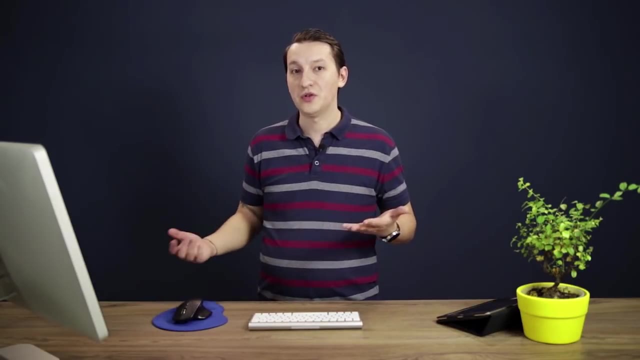 And that's it really. It's a very simple method of creating a slider, and a responsive one at that. It doesn't have any touch-enabled features, like when you're on a smartphone and you swipe it's gonna change slide. It doesn't have that. Instead, it just uses these two buttons. 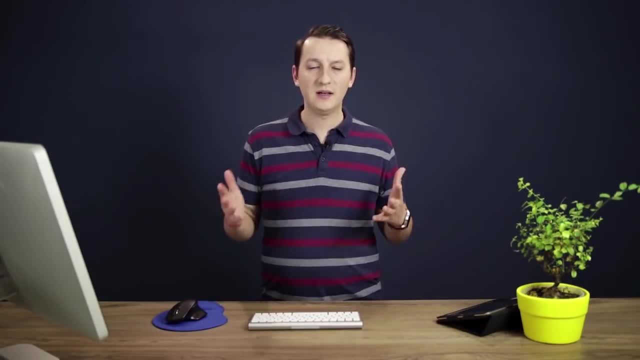 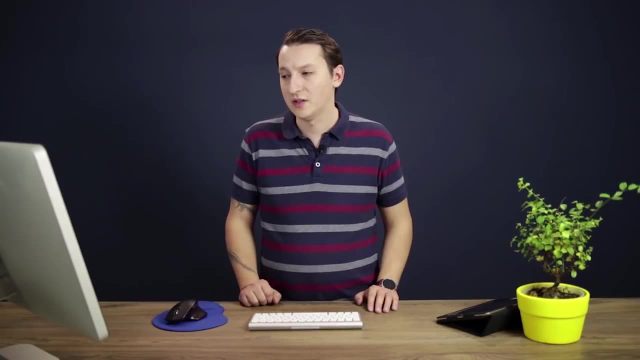 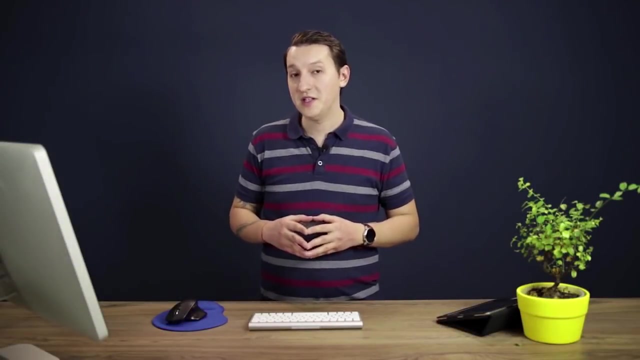 Now our fourth demo will be a image slider- Again a very popular JavaScript pattern that's being used in a lot of web apps, So we're gonna create that in the next lesson. Hello and welcome to lesson number 15, where we'll create a very simple image. 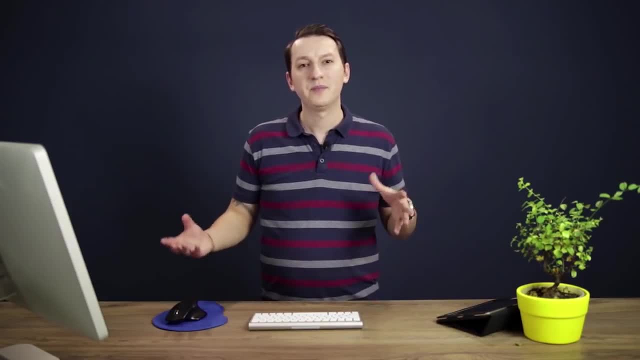 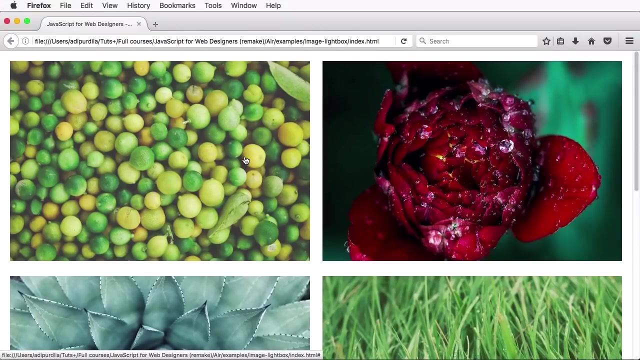 lightbox, And a lightbox is usually an overlay that shows a much bigger version of a thumbnail, essentially a larger image. So here's the finished result. We're gonna do the same thing as the previous: I'm gonna show you the finished result. 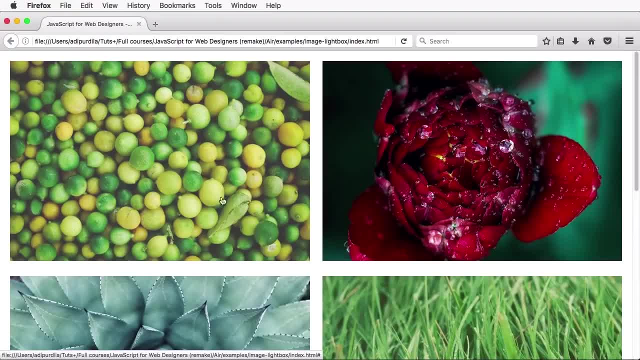 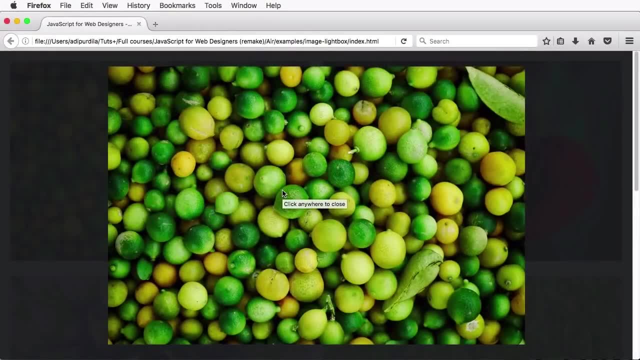 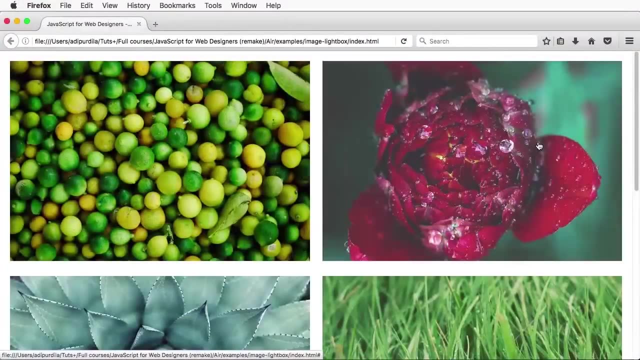 I'm gonna show you the code and just walk you through it. So we have a bunch of images here and when I click one of them we have this nice transition into a bigger version of that image And clicking anywhere will actually close that and 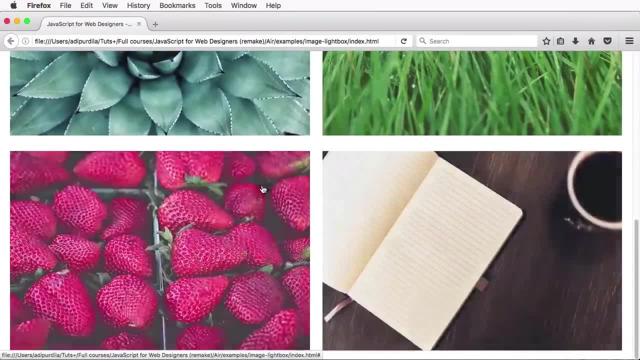 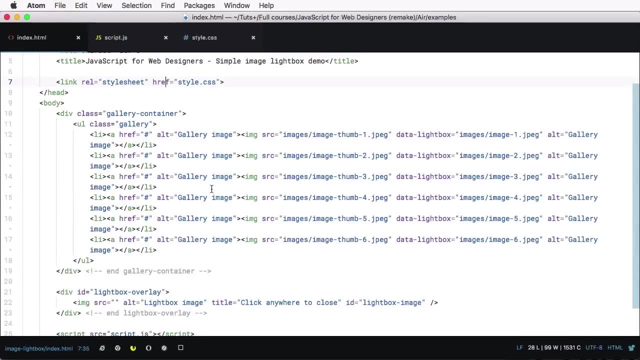 return us to our original screen. Now the markup. we basically have a UL with a class of gallery and each image has its SRC to a UL. So we have a thumbnail and then data lightbox to the main image And at the end we have a div with an ID of lightbox overlay. 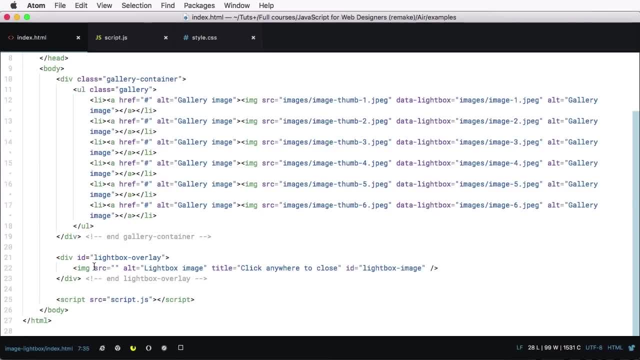 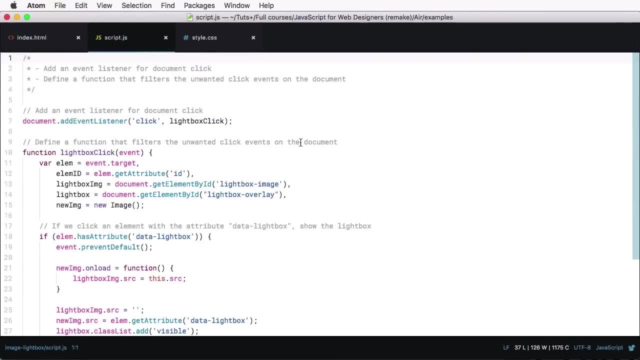 And this image element will be used to show the main or the bigger image. Now for the script, and the script is actually very, very simple here. We just have one event listener Click and we're listening on the document anywhere. 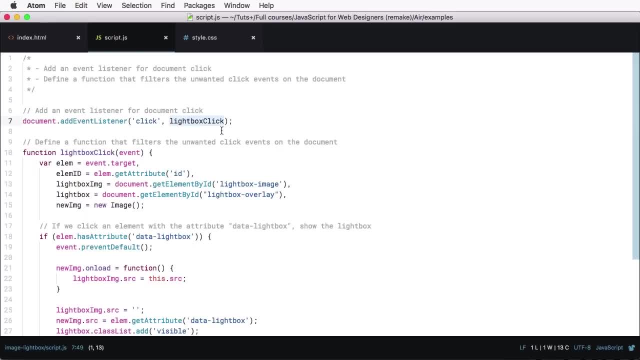 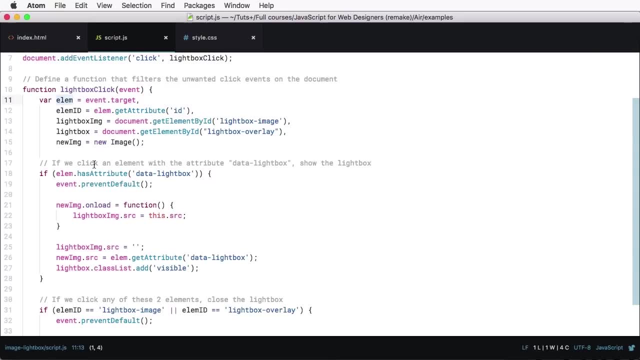 basically, and we're triggering the lightbox click function. So lightbox click gets the element that was clicked on, gets the ID of the element, gets the image that needs to display the larger version, gets the lightbox overlay itself and it creates a new image. 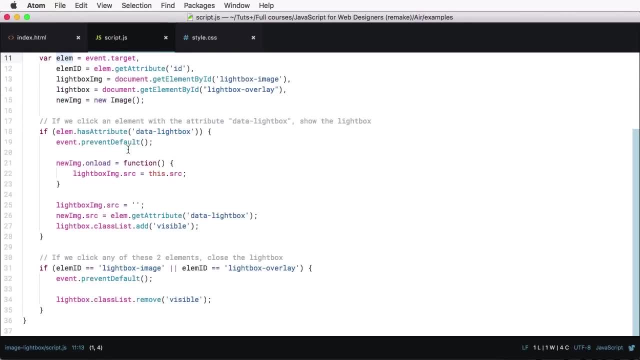 And this is actually another way of listening to click events. So, for example, instead of specifying which element we should listen for for click events, we're doing: document add event listener click And then, inside the function, that's triggered. 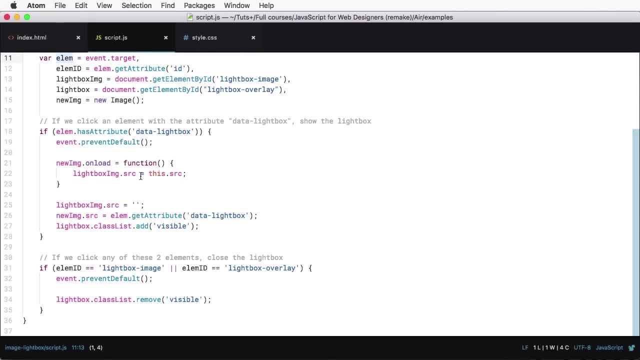 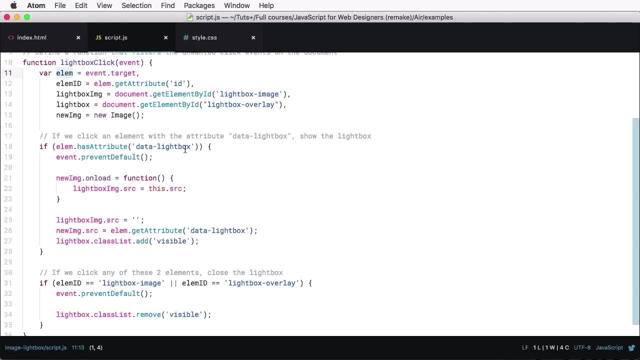 we just filter the results like we do here. So, for example, if the element we clicked on has the attribute of data lightbox, that means if we clicked on one of those images, then we know we have to open the overlay. 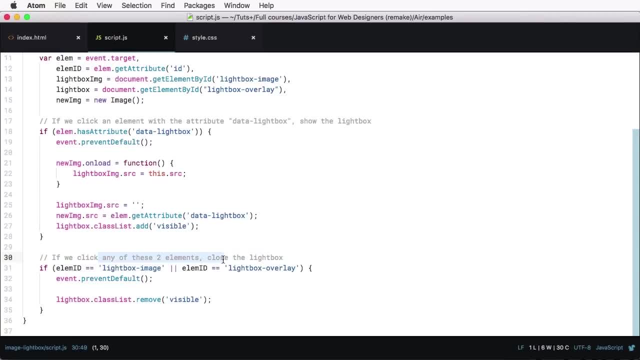 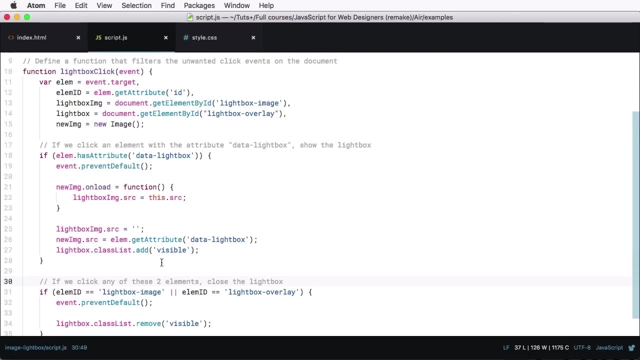 Otherwise, if we click on either the lightbox image, which is the image that's being shown, or the lightbox overlay, then we're gonna close the lightbox or we're gonna remove the overlay And inside here. so if we're clicking on one of the images, 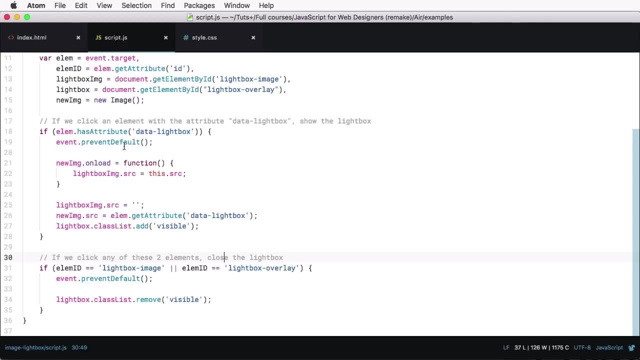 one of the thumbnails. we're preventing the default behavior because we are dealing with anchor tags And then we're creating a new image and onLoad We're setting its SRC to the SRC of the image we clicked on, Then we remove the old source from the lightbox image and 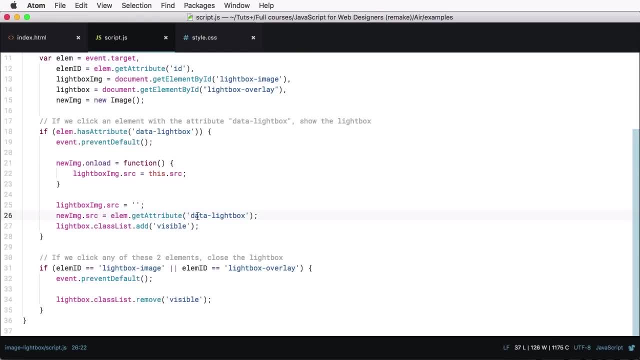 we're setting the source of the new image to the source of the image we clicked on. So, essentially, when we're doing this bit, we're triggering this function here And finally we're showing the lightbox, and that's all there is to it, really. 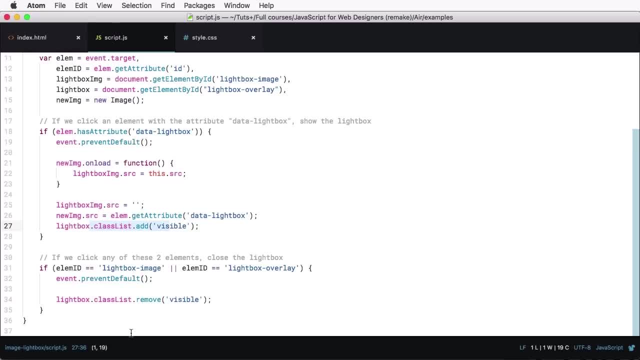 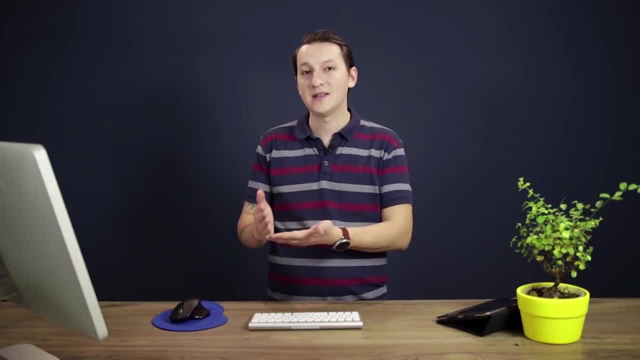 Again a very, very simple script. Just one event listener and we're doing two if statements. We're checking. hey, where exactly did you click? Did you click on one of those thumbnails? Fine, it means we need to open a new image. 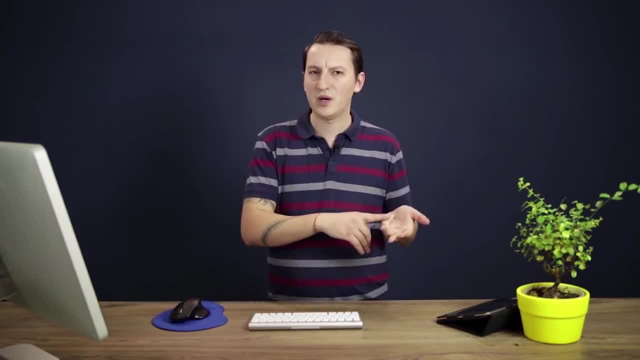 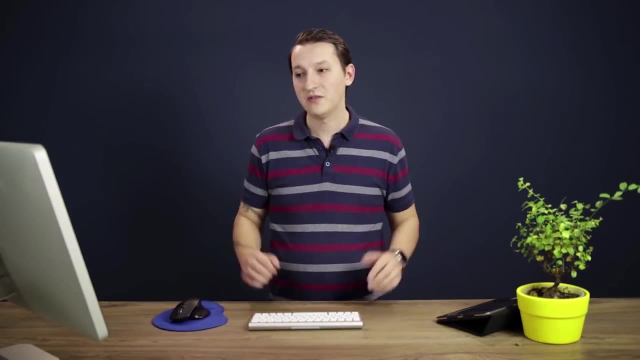 You clicked on anywhere else. you clicked on the lightbox overlay or the lightbox image. fine, That means we have to close the overlay, very, very simple. Now, the final demo we're gonna be looking at shows a very popular element. 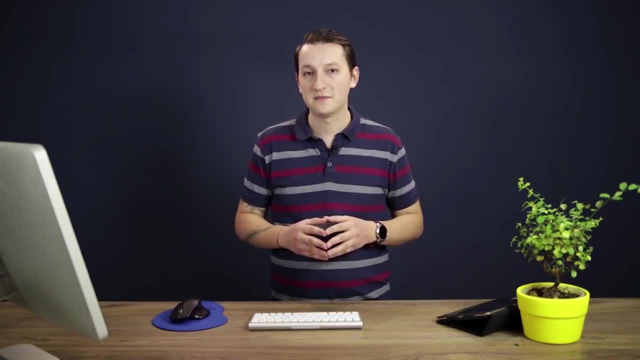 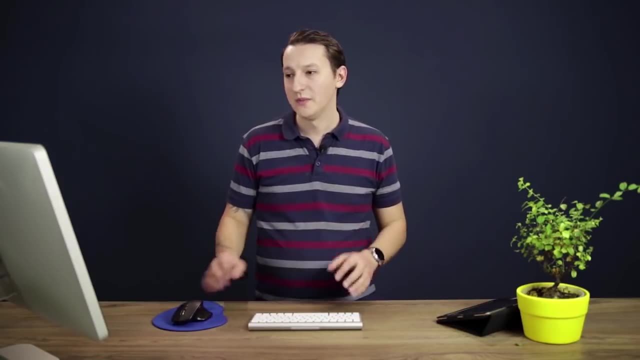 and that is a tab control. See you on the next lesson. Hi, welcome to lesson number 16, where I'll show you how you can build a very simple tab control. So this is the final result. As you can see, we have three tabs. 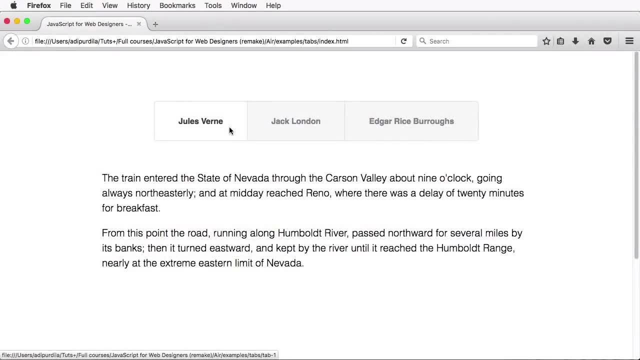 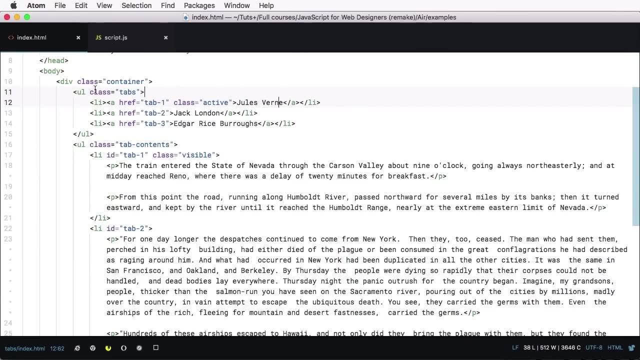 And clicking each one will toggle a different content. Now the markup is pretty straightforward. We have a new UL with a class of tabs that hold the links here on the top, The active one has the class of active And then we have tab contents which refer to these right here. 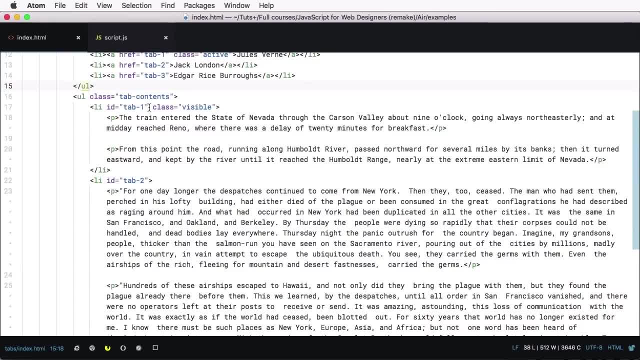 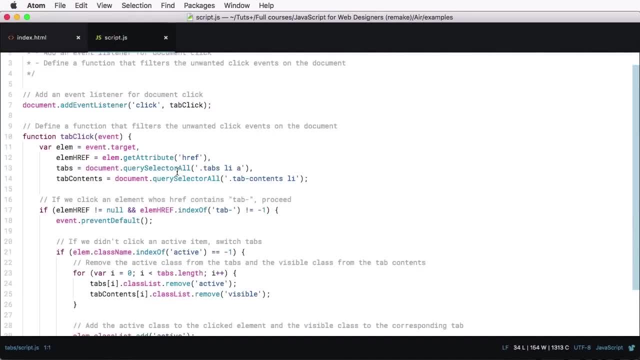 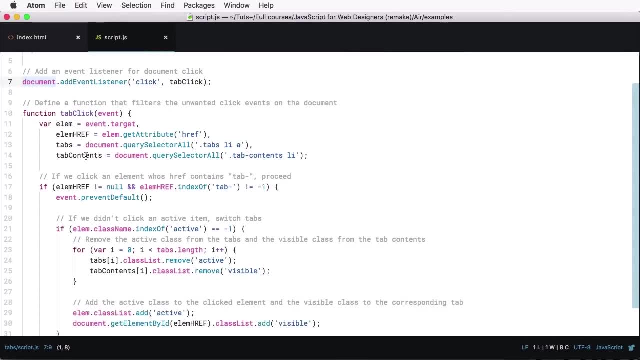 Each one has an ID tab- one, two, three and so on- And the active one has a class of visible. Very simple. Now the scripts. we do something similar to the previous demo: We're listening to click events on the document and then we're filtering them. 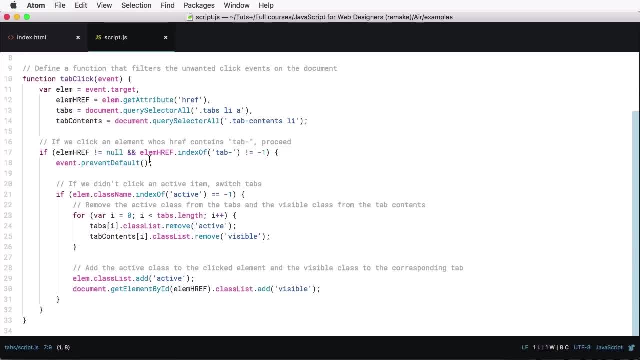 So if we clicked on an element whose href contains tab dash, then we move on, otherwise we do nothing. So if the href of the element, basically we get the attribute of the element that has been clicked, If it's not null and if it has tab dash inside it. 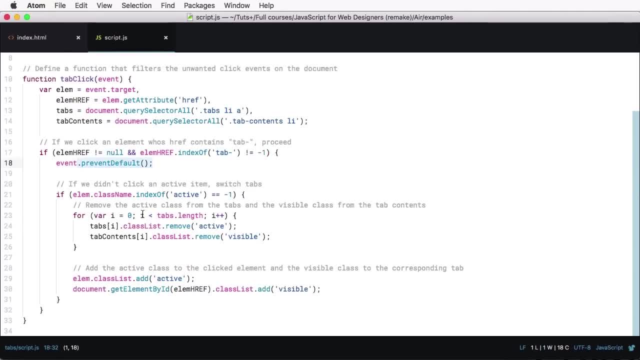 then, since we're dealing with links, we're gonna prevent default behavior And we check if we didn't click on an active tab. we switch tabs, We remove the active class from all the tabs and all the tab contents And we simply add it to the one, to the element that we just clicked. 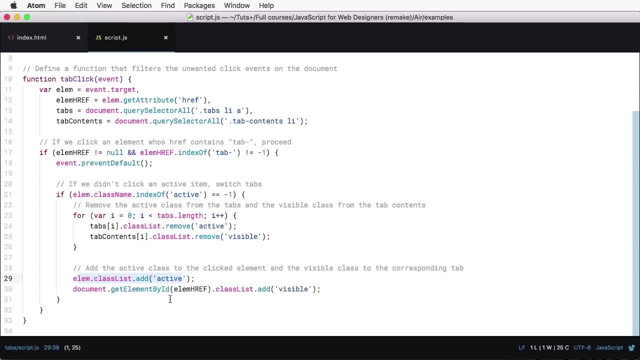 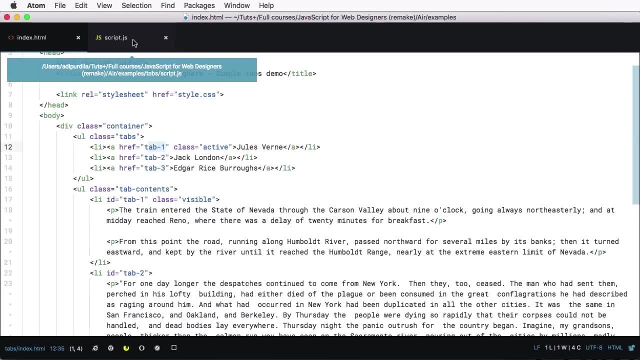 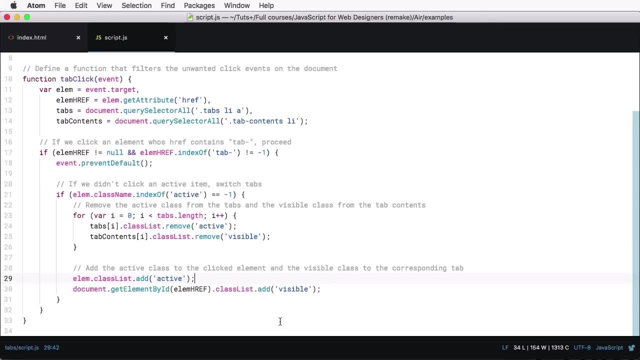 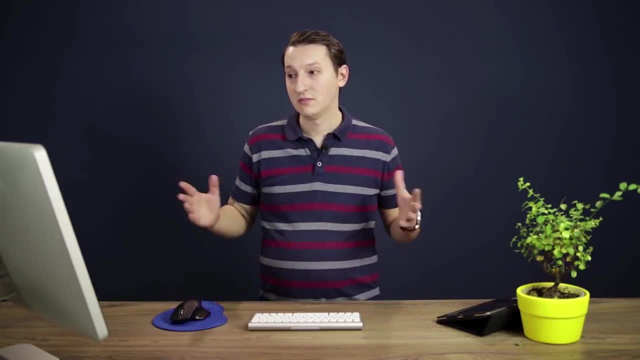 The href is tab1.. So we're getting that byId and we're gonna get to this item, Very, very simple, And we just add the class of visible. So that's how we can create tabs. As you can see, very few lines of code and a very basic principle behind it. 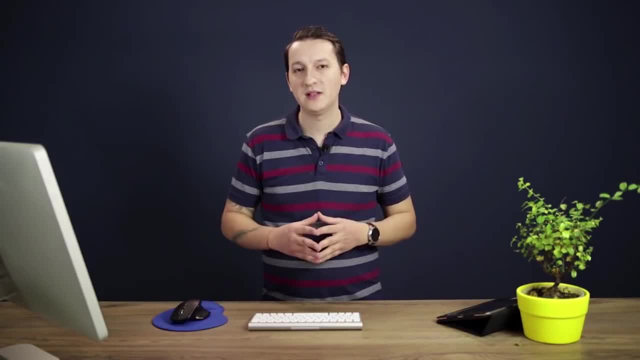 That was the final demo for this course. Please join me in the next one. Next lesson for the conclusion: Hi, welcome to the conclusion lesson of this course. I really hope you got a better understanding of what you can do with JavaScript as a web designer, right? 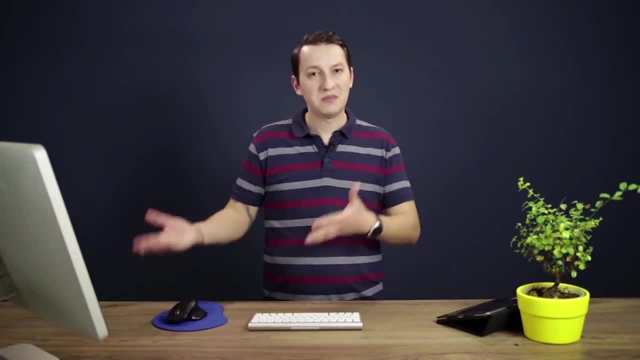 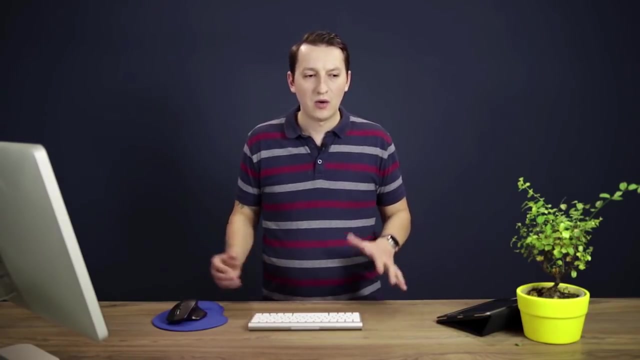 And, more importantly, how to do that. You saw some demos and those demos represent kind of very popular elements that you will find and elements that at some point you might be required to create yourself. Now you might have downloaded various components like sliders and 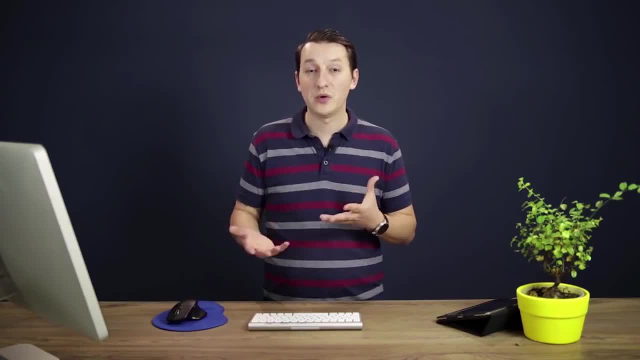